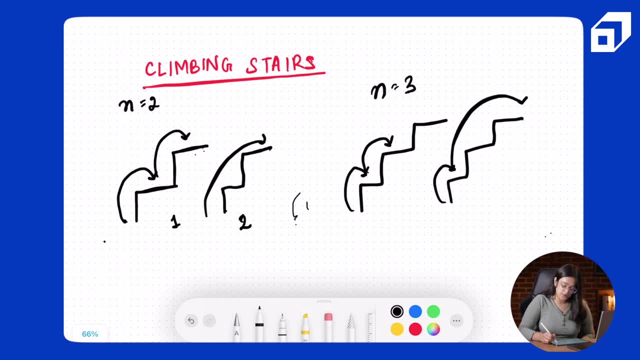 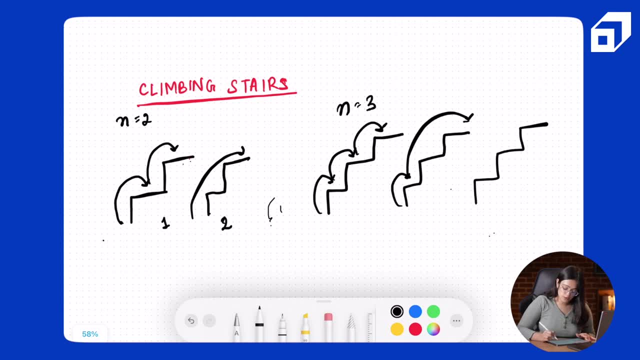 So it's like this or like this, and here we have to take one another step. There's also a possibility where we can take two steps initially and then one step. So there's only these three ways using which we can climb to the top, if there. 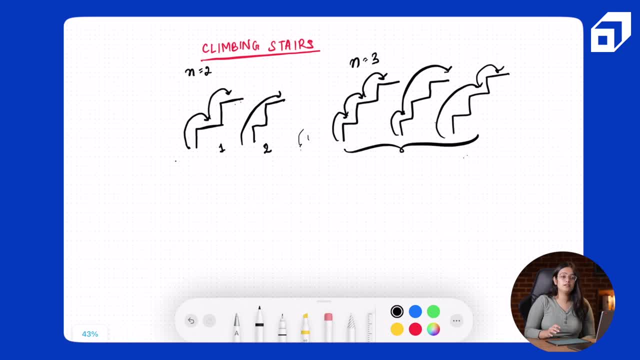 are three stairs, So now we have to find a the number of ways we can reach to the top for any generic n value. We were able to do this manually for n equal to 2 and n equal to 3, because these were pretty. 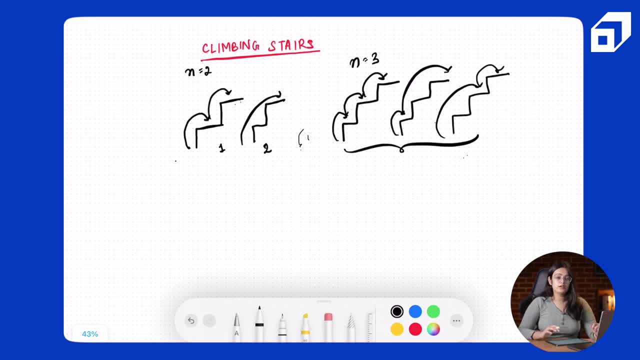 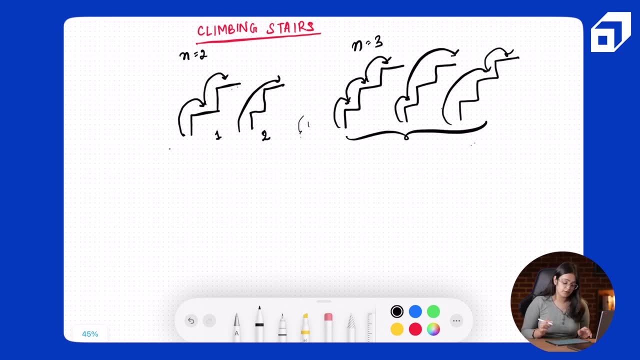 small values and it was easy to find, But here we are aiming to find it programmatically. So, if you observe, in this particular example or in this particular problem, we can either take one step or we can take two steps. So the 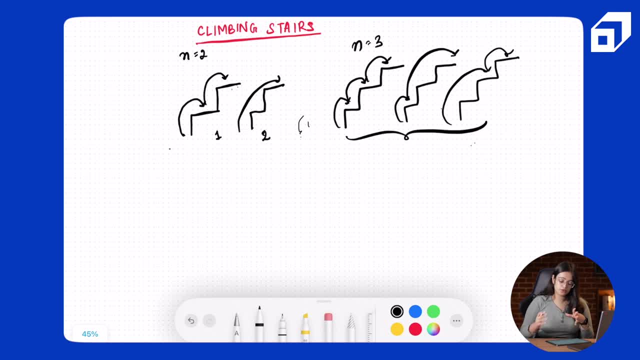 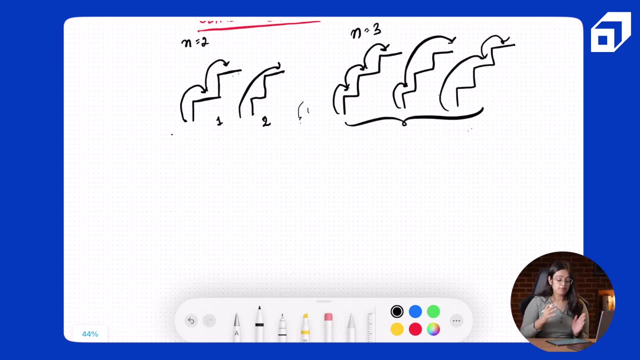 number of ways that are there to reach the top would be the summation of the number of ways that are there if we start with one step, plus the number of ways that are there if we start with two steps. So let's say we are standing at. 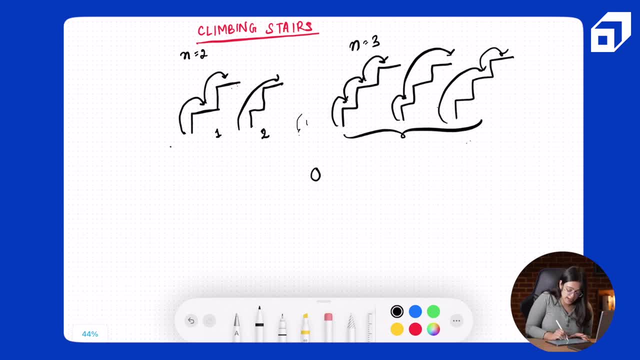 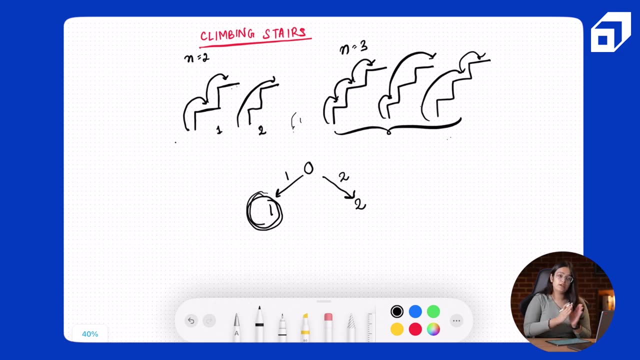 this ground at the stair zero. So we either take one step and we reach one, or we take two steps and we reach two. The answer would be the sum of the ways that would come from this chart. this point Like when we are going from one forward. 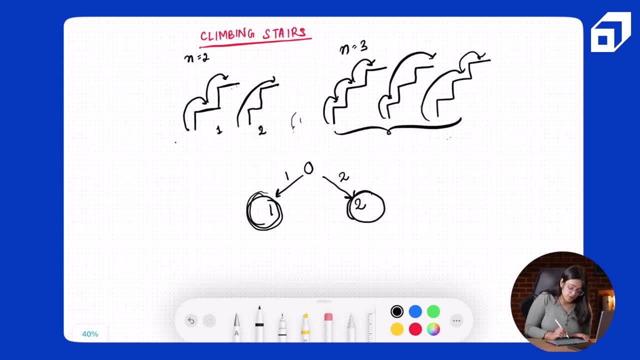 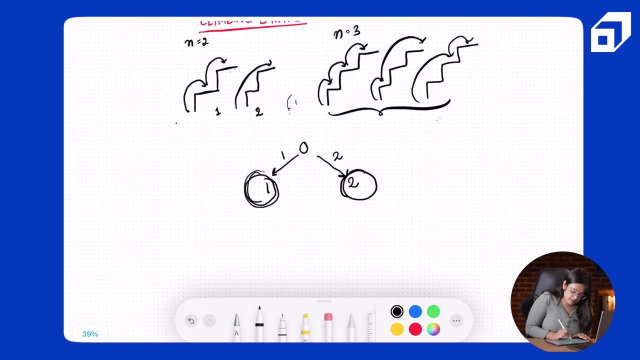 and the number of ways that would come from this path. So let's do it further, let's create our chart further for n equal to three. Then, when we are at the first stair, then again we can either take one step or we can take two steps. 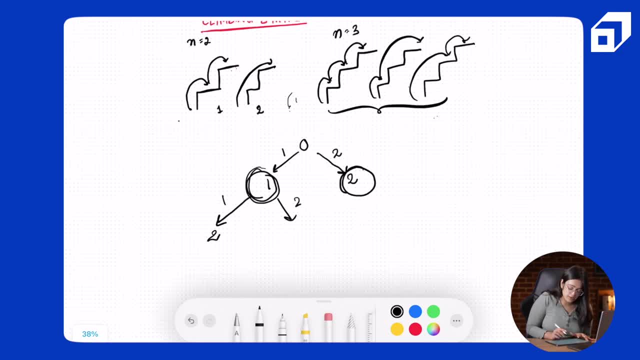 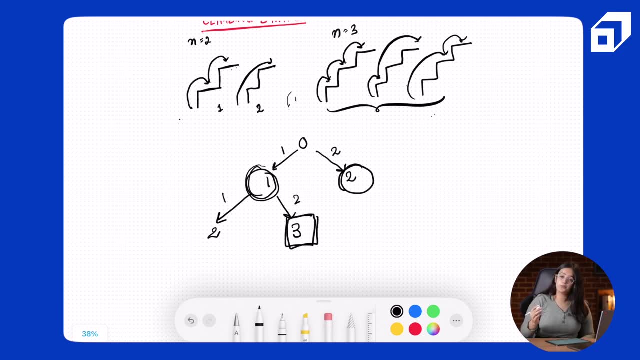 So if we take one step, we reach second stair. If we take two steps, we reach the third stair. So this is one answer. We've already reached our top of this stairs. So this is one answer, and from here we'll return one. So this path has. 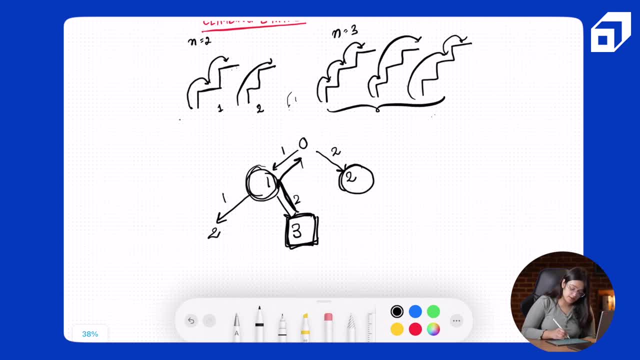 given us one answer: It will return to this stair and we will return it to the final zero. Then, from this path, we've reached two. There is again two ways: Either we take one step, we reach three, or we take two steps, we reach four. If we 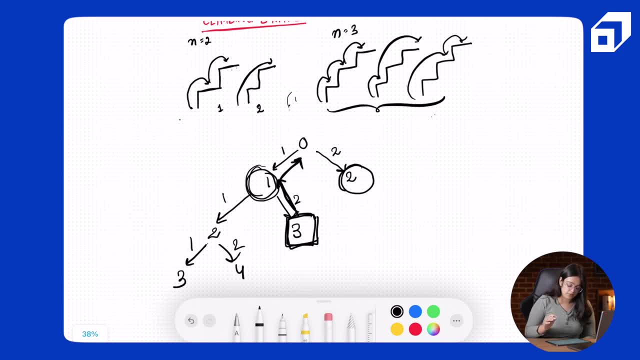 take two steps. it's out of the like, out of bounds, or we can say our array is considered till 3 only, since we have to reach the top. so this is out of the, this is out of the solution. we can't take this possibility. this is one answer again and this will return one, one way. 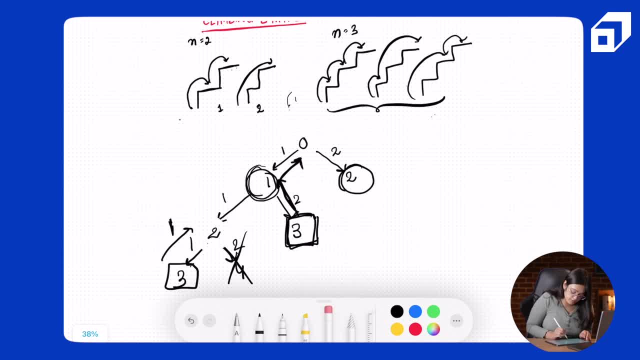 is there. so, basically, if we see from this point, if we see from second stair, at this point we have only one way. we are summing up the ways coming from both the sides, but since this, this right one, is returning zero, so we have just one way now. this will return one upwards and we this also return one. so this path, 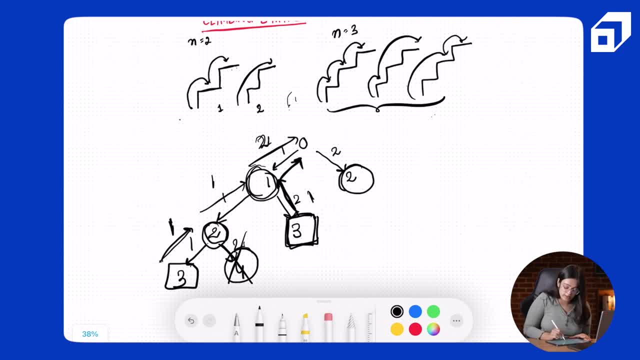 returns two as the answer. going along again, this right path again. here again, we can either take one step or we can take two steps. we take one step, we reach the top. if we take two steps, we reach four, which is out of bounds. so this path returns one. this path returns one again. so we were getting two from the left. 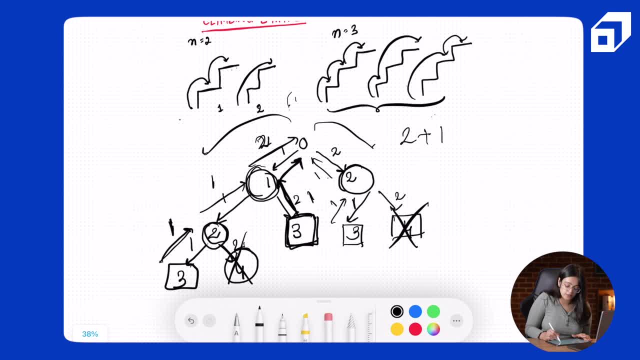 side and one from the right side. so 2 plus 1, equal to 3. now, if you observe carefully this, the paths that we're getting answer from is one, one, one and one, like three steps: one, one and one. so this is this answer that we discussed earlier: the. 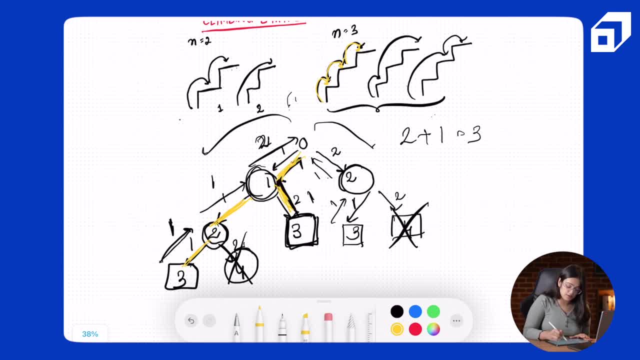 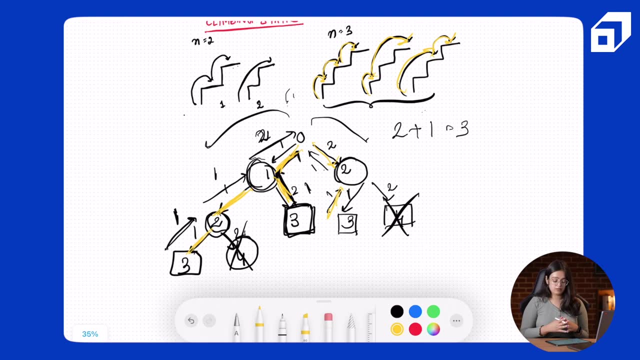 other answer that we are getting is one and two. this is this part that we discussed, and the third answer that we are getting is two and one. so this is this path that we discussed. So, all in all, what we get to know is the answer for. 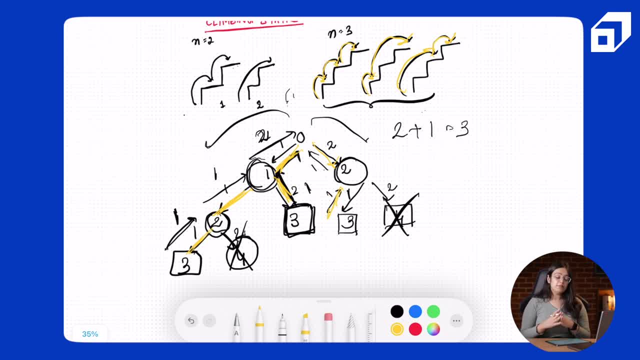 any particular point, starting from any particular point, will be the sum of answers that we get if we take one step at each point or we take two steps at each point. whatever answers we're getting from these two, which are successful answers, which is getting us to the top, those are the answers which 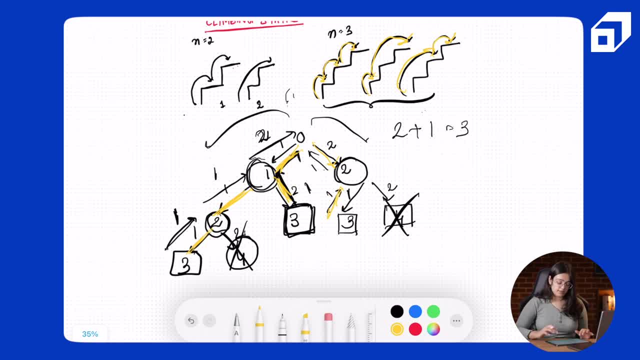 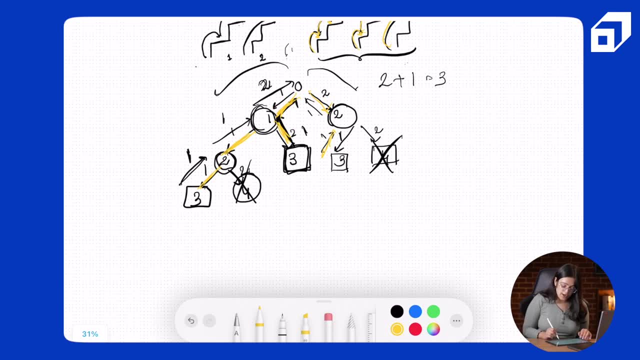 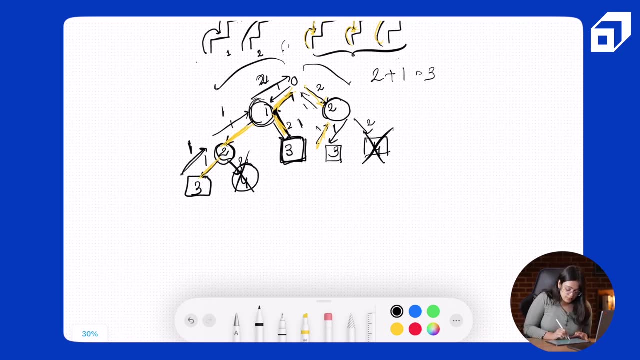 we have to sum up to actually find a final answer. So now we can try to write the recursive function for this, basically the recursive statement which will help us write the code. So for any generic point where we are standing for any generic value of n, our answer will be the sum of the number of paths we are 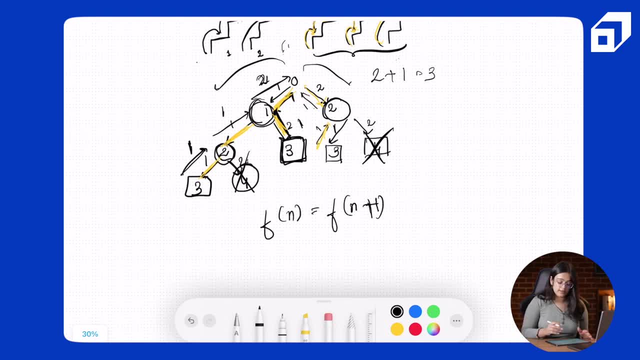 finding from by taking one step. so it's like, if you're standing at zero, it's the summation of number of paths coming from one after taking one step and number of paths coming from the second step after taking two steps. So f of one is f of n. 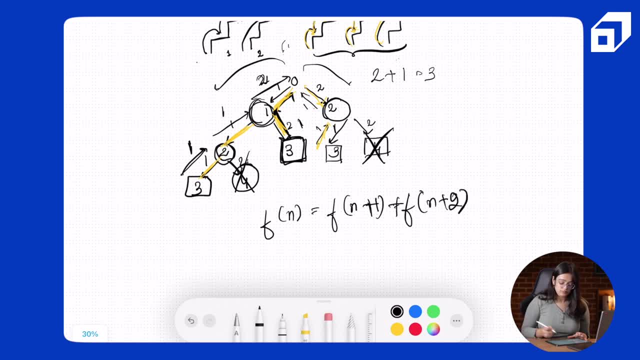 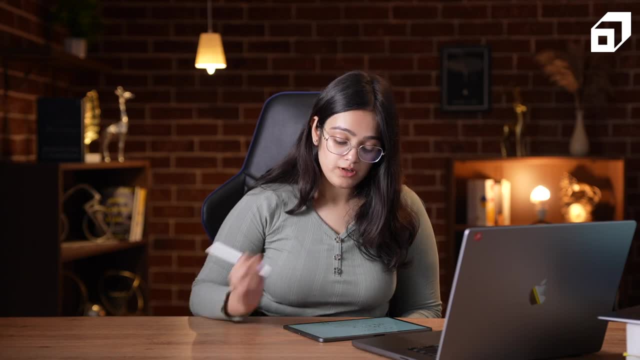 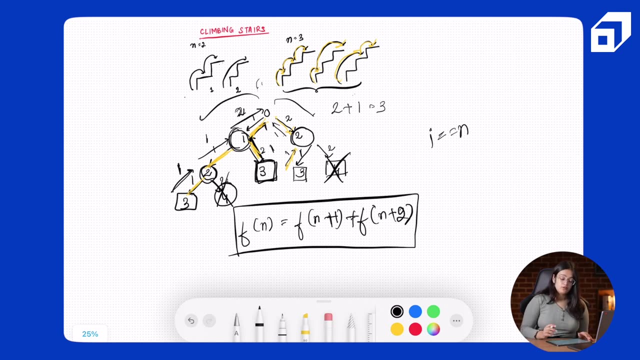 plus one plus f of n plus two. That's our recursive solution. Also, before moving on to the code, let's also discuss what the base case for the solution would be. So the base case would be: IE equal to equal to n. So n is our target. It's the point where we have to reach at. 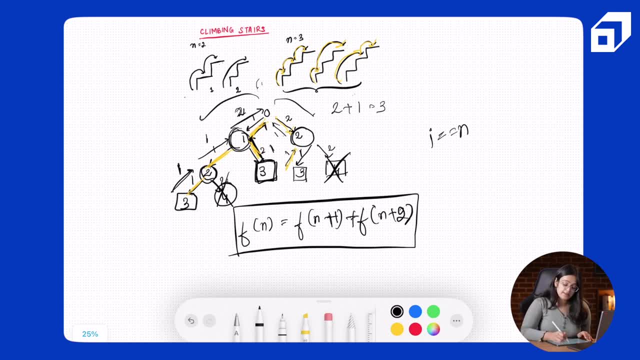 the end. So if we are already standing at n, if we're already standing at stair 3, that's when we've already got a successful solution. You would have seen that whenever we were reaching 3 in our recursive function, which means we would- 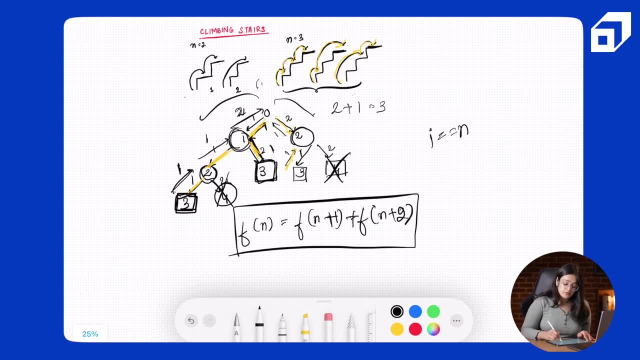 have achieved our target. we were returning 1 as the answer. So, whenever I equal to, equal to n, that's the, that's one way that we've achieved. So whenever we come to this base case, we will return 1.. Also, if we, if we reach to a number, 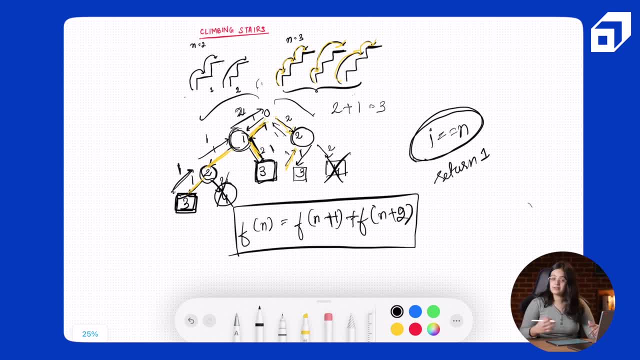 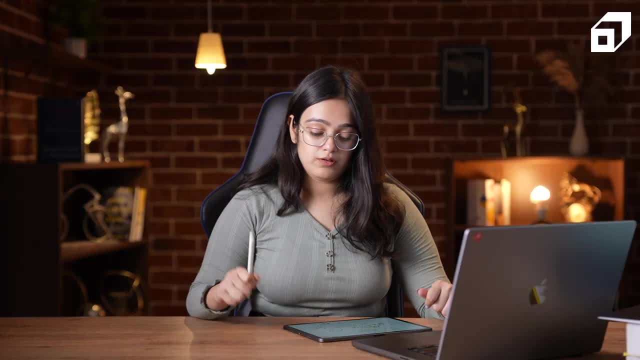 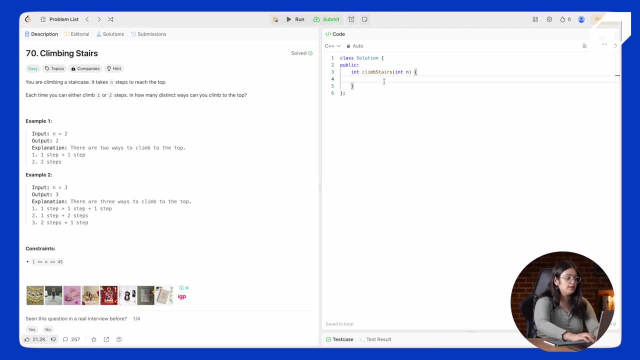 which is greater than n. so if we reach 4, let's say so, that's an invalid path. In those scenarios we will return 0.. So now let's write the code for this problem. So we have cLimbStairs, int n. I will just create a helper function. so int N. 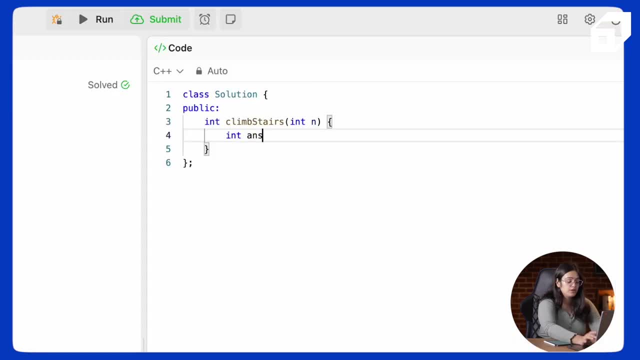 So we have cLimbStairs? int N. I will just create a helper function. so int N I will just create a helper function. so int N I will just create a helper function. so int N. answer equal to helper and we will pass on n. We will also pass on the starting. 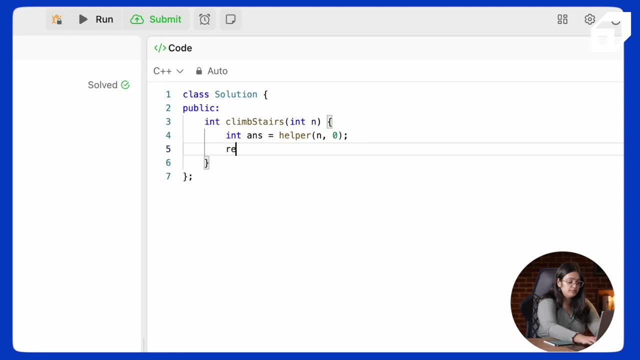 point, which is i. Here it's 0 and at the end we will return our answer. Let's quickly define our helper function. So, as I told, the base case is if i equal to equal to n, we have to return 1, and if i goes out of. 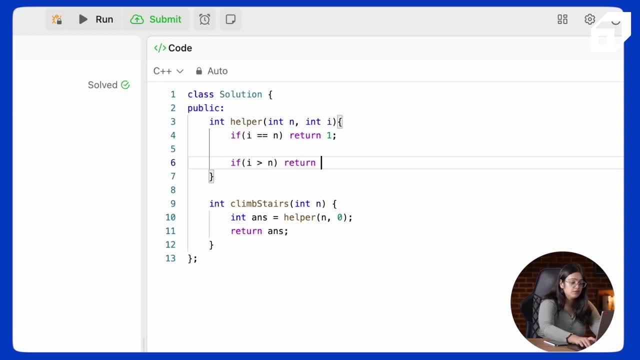 bounds, we can simply return 0 and the generic solution for anywhere value of n would be a summation of number of ways that come after taking one step plus the number of ways that come after taking two steps. So if it's f of n plus 1 plus f of n plus 2.. 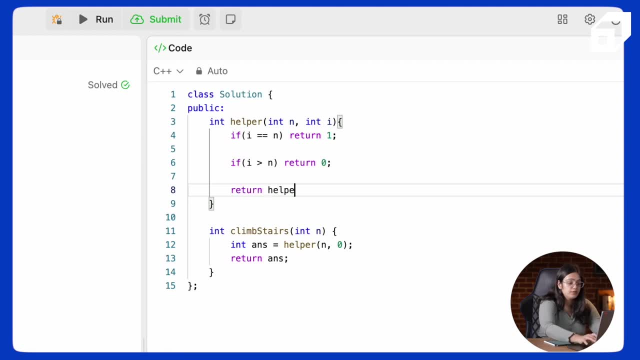 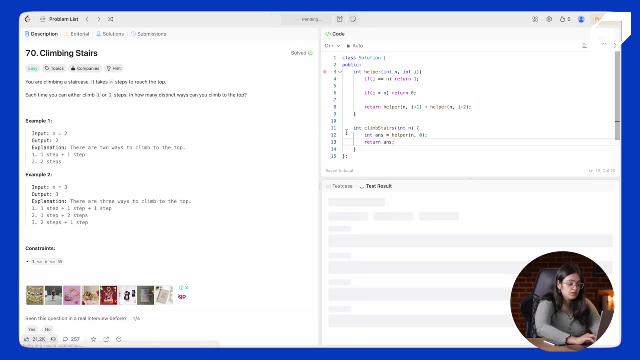 So I'll simply write return helper. I'll just write n i plus 1.. Plus helper of n i plus 2.. We can quickly test our code and see if it works. Yeah, so you see that for 2 it's giving the answer as 2 and for 3 it's giving the answer as 3.. 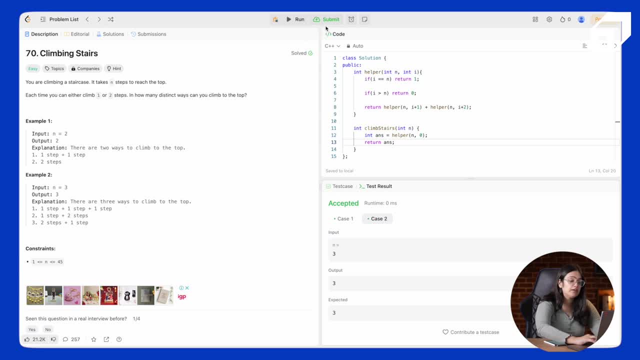 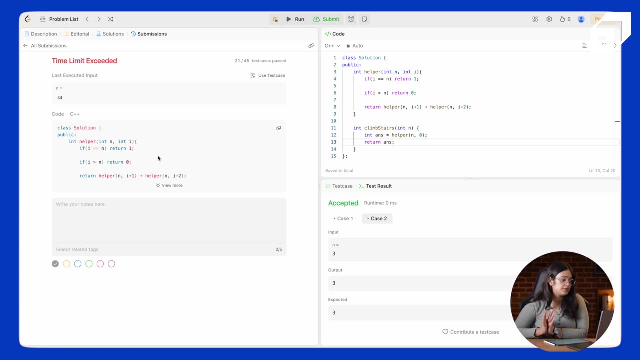 Let's try to submit our solution and see if it works fine for all the test cases. So it's giving us a time limit exceeded result. That's because if you're making recursive calls, if you're making two calls at every step, the time complexity will be really huge and it will go approximately 2 to the power n. 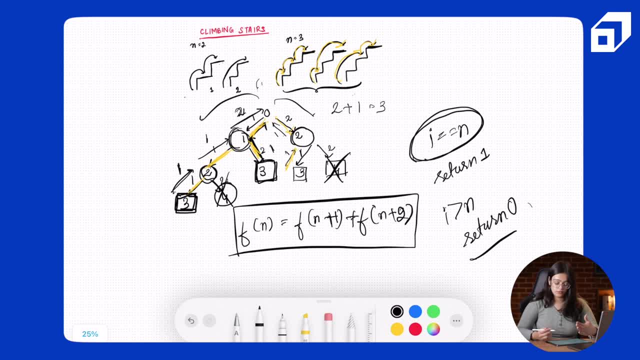 because at every step we are making two branches. So it will, like the branches will be 1 plus 2 plus 4 and so on, and it will come out to be 2 to the power n. So this isn't an option. 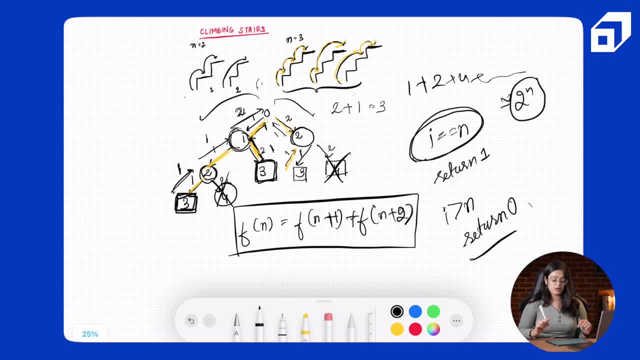 This is an optimal solution and we need to make it better and so that it works for higher n values. Since we're already given in the question time constraints, which is 45 and 2 to the power, 45 is going to be very huge. 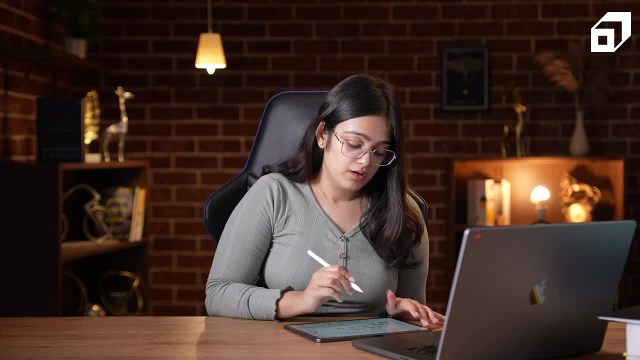 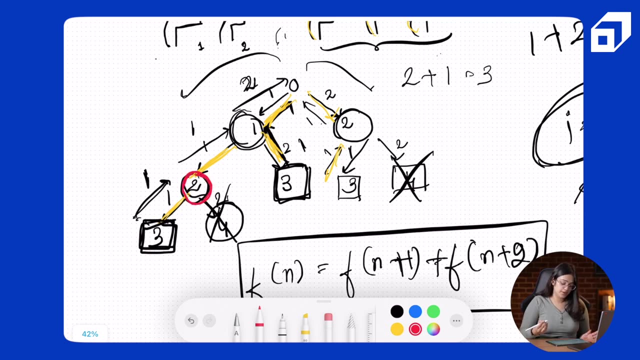 So if we observe our recursion tree, we have a few overlapping subproblems. So you see 2 here right, 2 again here. it has two parts and it's returning 1 as an answer. Here it's returning 1 as an answer. 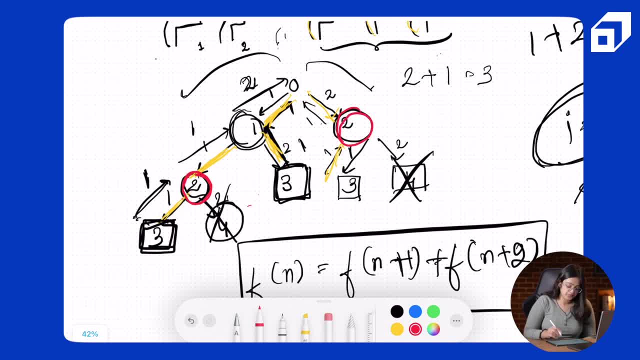 Here again we are having 2 and it's returning the same answer. So these are overlapping subproblems and the substructure also is optimal here and in such cases we can try to apply DP. So as we talked earlier that there are in the previous video that there are two ways of applying DP, 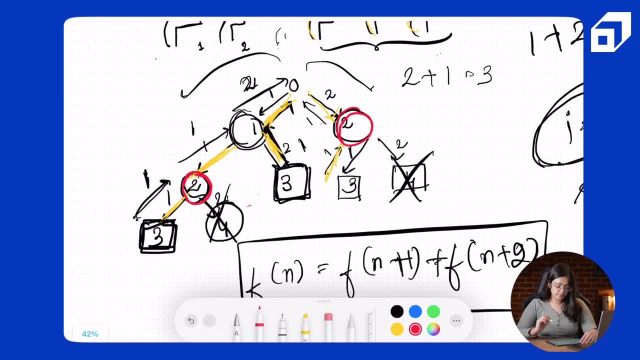 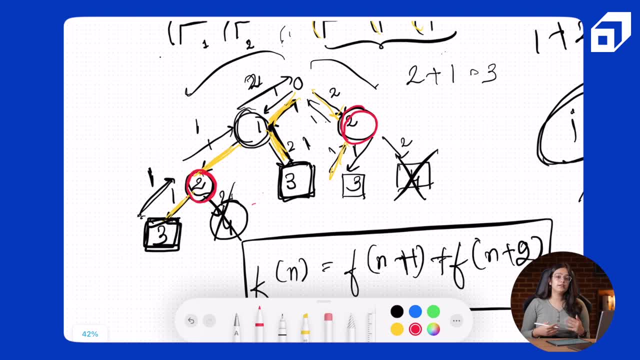 One is memoization and one is tabulation, So memoization is quite easy to implement. What we can simply do is, instead of calculating the result for this stage or any particular value of i again and again, we can just memoize it. 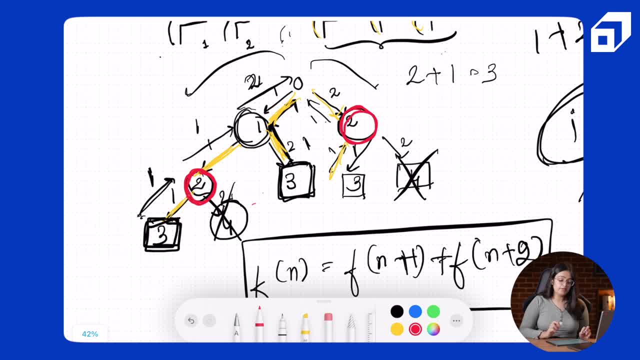 We can store the result in a DP table and we can refer to it. So before calculating it once again, we can always refer to it. If it's already stored, we don't need to calculate it. So let's say when we were going through this path: 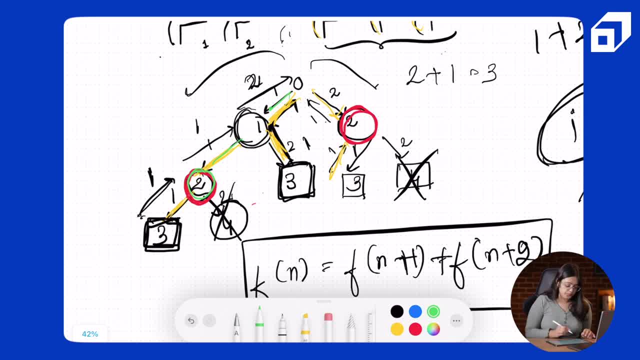 the left path and we already calculated an answer for 2.. So what we can do is in our table- let's have our DP table from 0 to 3.. In our table we can store answer for 2 as 1.. 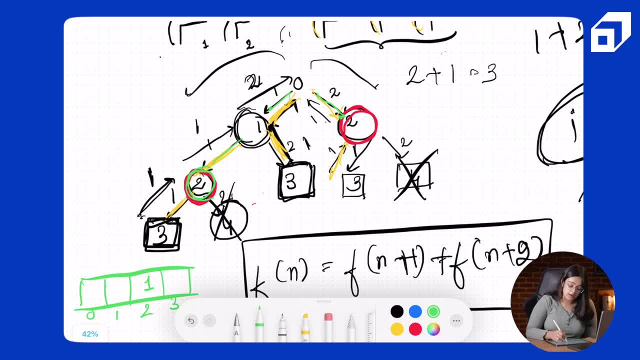 So when we again come to 2, in the right path, we already have the answer stored and we don't have to calculate it again. So when I'm coming to 2, I won't make any other recursive calls. I'll just check that my answer is stored in the DP table. 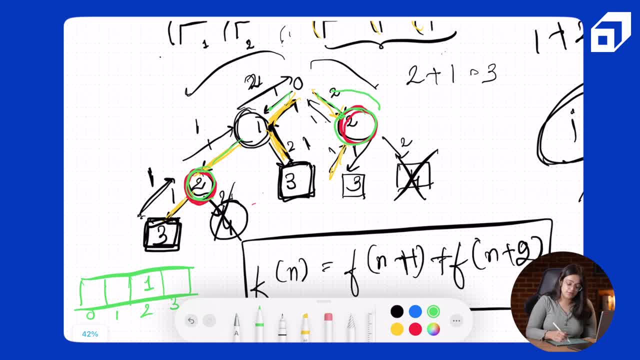 and I'll refer to the same answer and just return the answer from here. So how exactly do we go about filling this DP table? Initially, our DP table will be empty, So it will have minus 1 at all 4 places, Whenever we encounter any value of i. 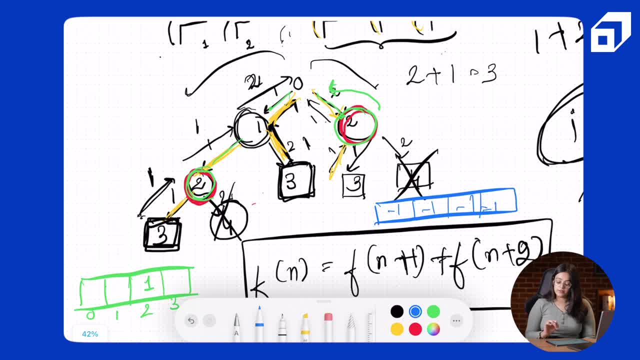 we'll check. is the value present at this i value? is the value for the DP table minus 1?? If it's minus 1, then we have to calculate and we will update the value in the DP table. Okay, And if it's not minus 1,. 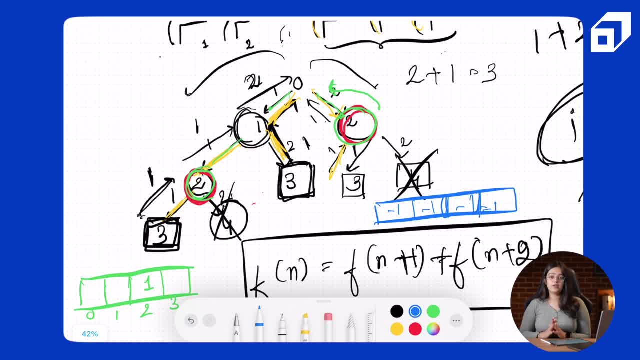 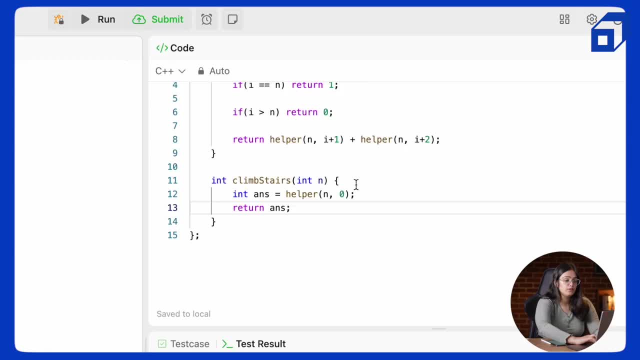 we'll simply reuse the value that we calculated earlier, So I'll just make the change in the previous code only. Let's make a DP table. I'll create a vector. Size will be n plus 1, because we have size 4 from 0 to 3.. 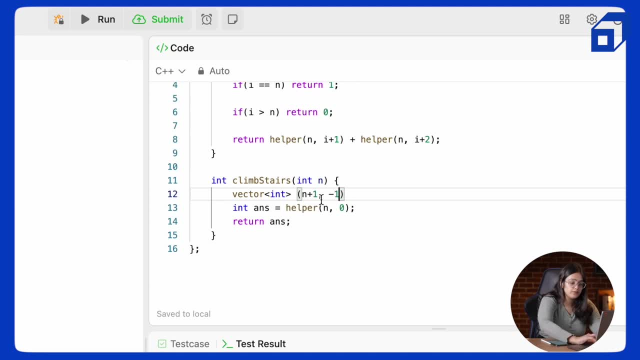 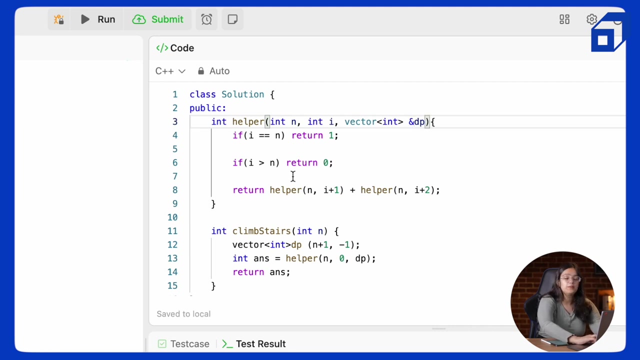 And I'll initialize it with 1. Vector: int. let's call it DP. Now I'll pass on this DP table to our helper function for calculation. Okay, So I'll just take this in our helper function and these base cases are fine. 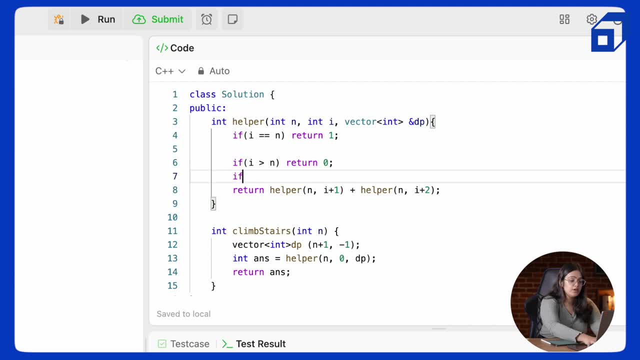 They'll remain the same. So if DP of i is not equal to minus 1,. so, as I said, if it was already calculated we would have it stored in the DP table. So if it was calculated, we can simply return DP of i. 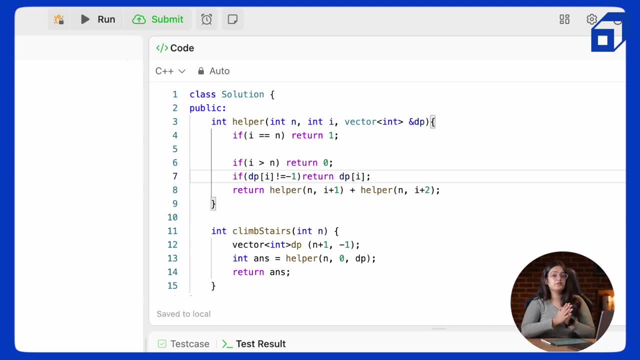 instead of going and making both of these recursive calls of helper i plus 1 and helper i plus 2.. But it was not calculated. If the DP at ith index is still minus 1, then we'll calculate the result. store it in a variable. 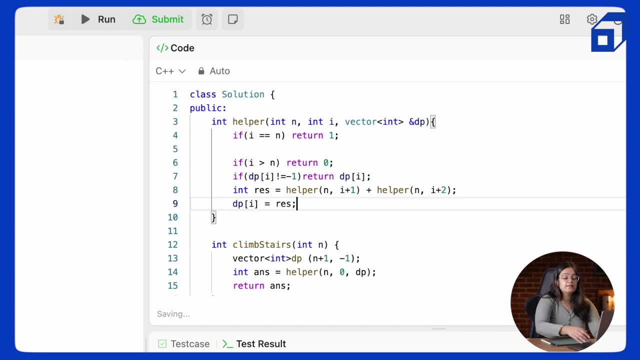 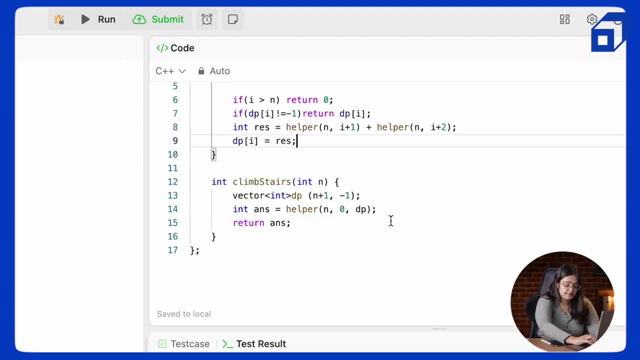 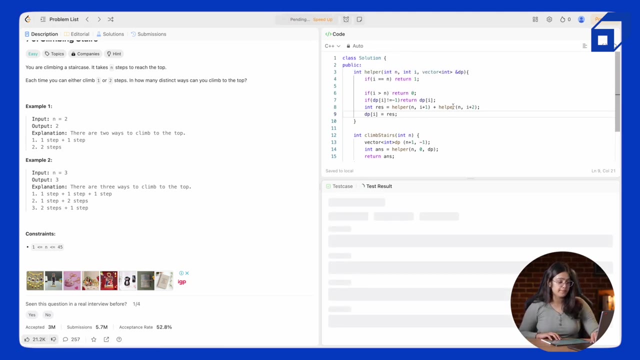 and we'll assign it to our DP. So the next time any call comes for the same value, we can just reuse it, Right? So let's just run this and see how it works out. Okay, So we have a small error. 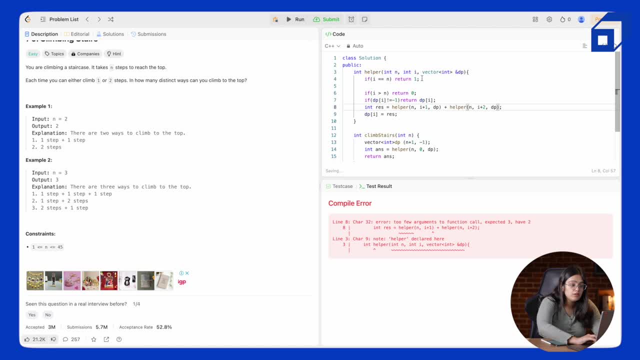 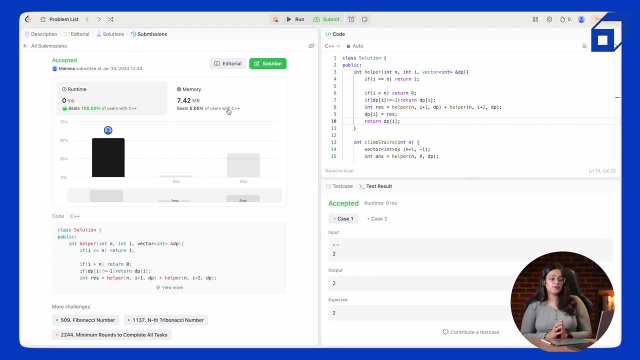 Let's just pass on the DP table here as well. Okay, So we have to return from this function. So what we'll do is we'll return DP. i Now let's try and submit. So this got accepted. And why it got accepted is because 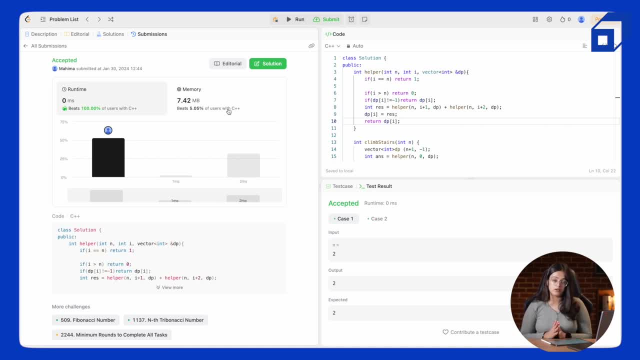 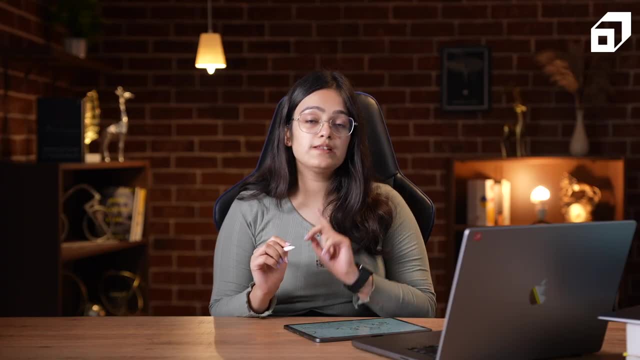 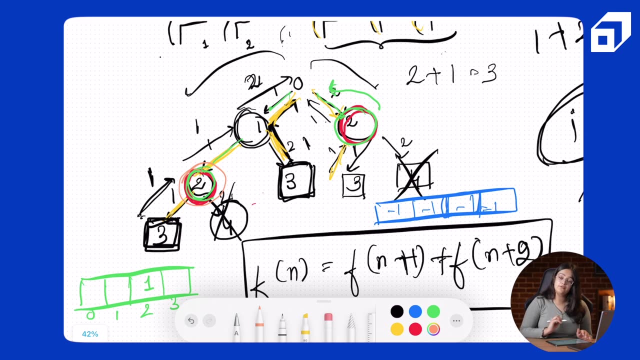 the time complexity is significantly reduced when we memoize this solution. So how is the time complexity reduced? Is that we're always calculating 1s for every i value. So when we came here at 2, we calculated for it 1s. 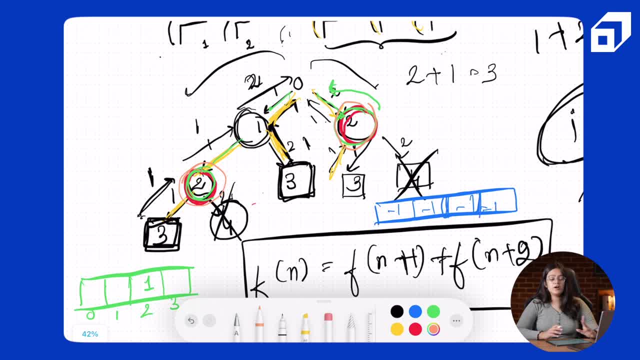 But when we came at this 2 again, we didn't calculate, We just returned from our already stored answer in the DP table. So here, since we are doing the calculation 1s for every number, so the time complexity will be O. 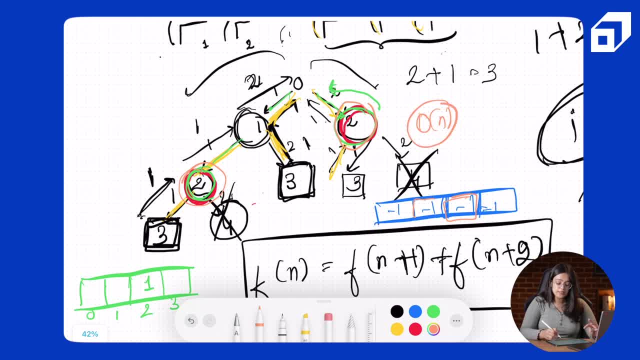 And the space complexity will also be O, because we are using an extra vector of size n plus 1.. So this is a significant optimization over the recursive solution. Now let's also write tabulation solution for the same problem. So for the sake of tabulation solution, 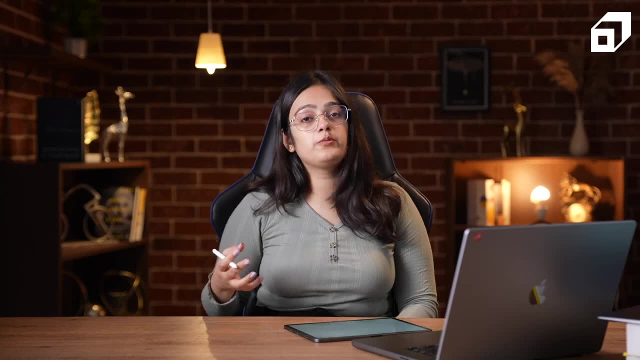 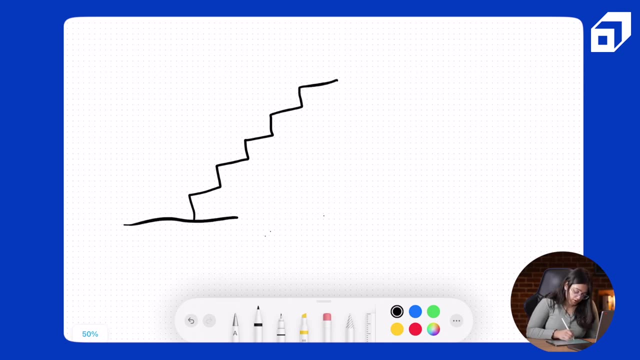 let's consider that- I mean, I'm trying to formulate the solution in a different way, similar, but just let's consider a different way. This was the ground and this was n. So we can also say that for reaching this n point, a person would come either by taking 1 step. 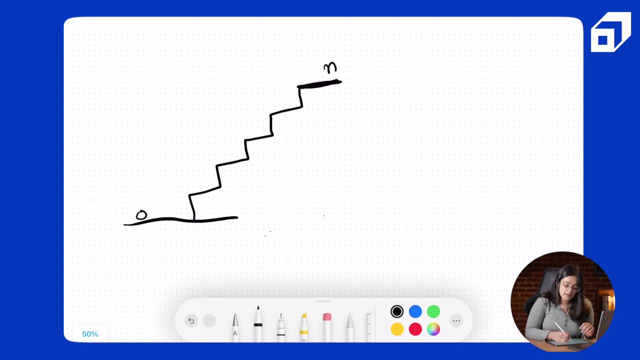 or by taking 2 steps. So a person can come either from the n minus 1th stair or the n minus 2th stair, n minus 2nd. So answer for n would be f of n minus 1 plus f of n minus 2.. 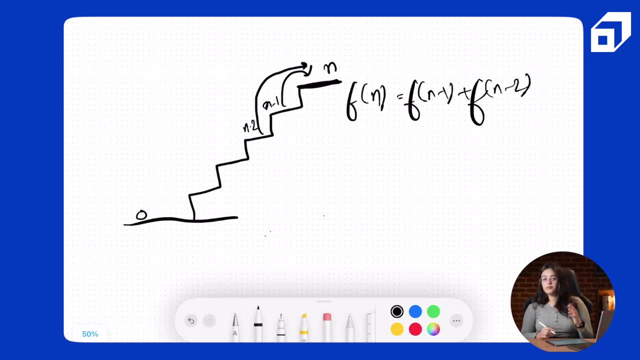 So the valid ways that are there to reach n from the n minus 1th step and the valid ways that are there to reach from the n minus 2th step. That is the answer for f of n. It's very similar, it's just a different way of writing this. 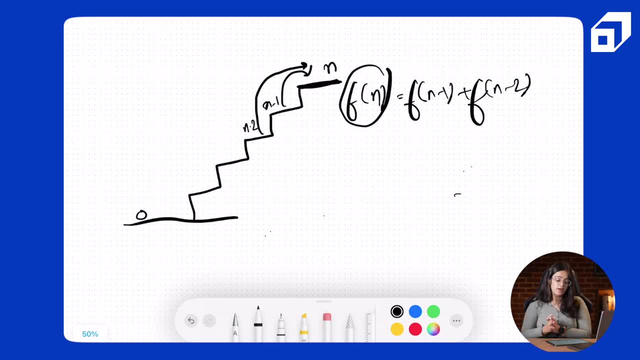 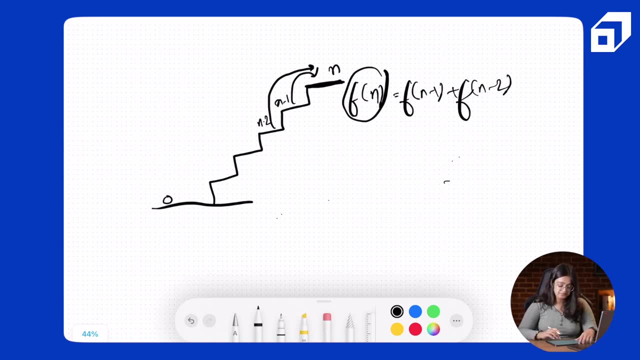 Initially we were having f of i equal to i plus 1, plus i plus 2.. And it just makes same sense here. So we will try to write a DP solution for the same. For this particular approach our base cases would be: first would be n equal to 0.. 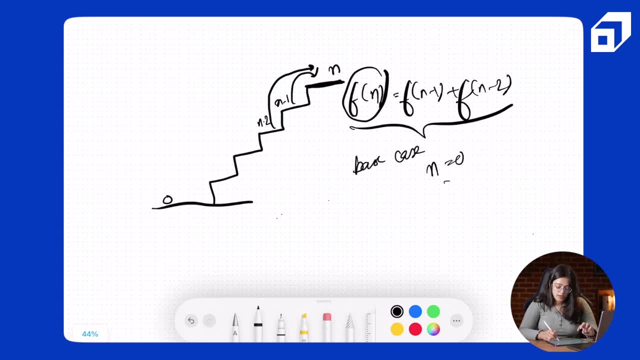 So we are already standing at n equal to 0. And the answer would be 0 for this particular point. So there are no ways to. we are already at 0.. So we can simply return 0 for n equal to 0.. 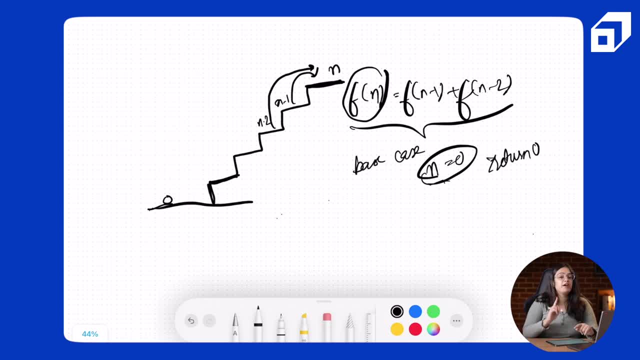 For n equal to 1,, there is only one way to reach 1.. So n equal to 1 means we can simply return 1.. We can just take one step from 0 and we will reach n equal to 1.. For n equal to 2,. 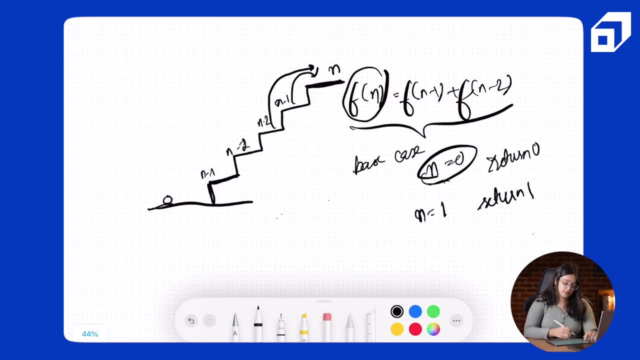 we already discussed earlier that there are two ways. Either we take two steps and we reach 2, or we take one step of two lengths. So either we take two steps or we take one step of two lengths, So the answer for 2 will be 2.. 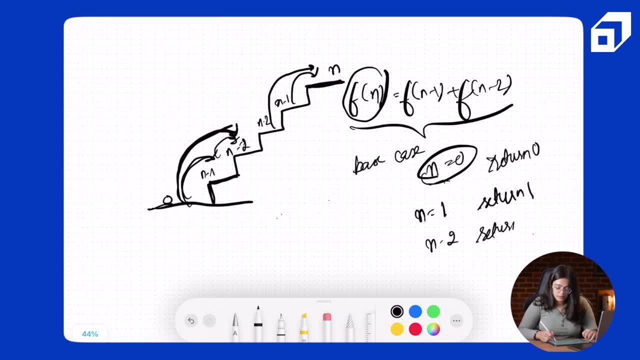 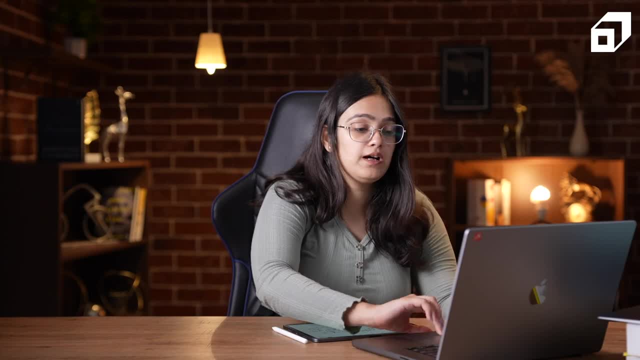 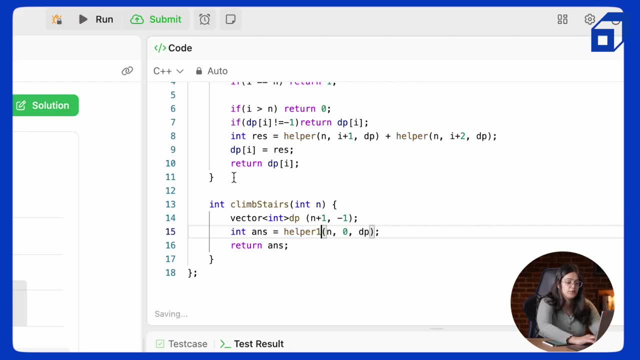 We'll make a separate helper function for it. Let's just make helper one, Or let's maybe write the code here itself instead of making the helper function. That would also work. So we already have a DP table. We can fill up dp of 0 with 0,, we can fill up dp of 1 with 1 and we can fill up dp of. 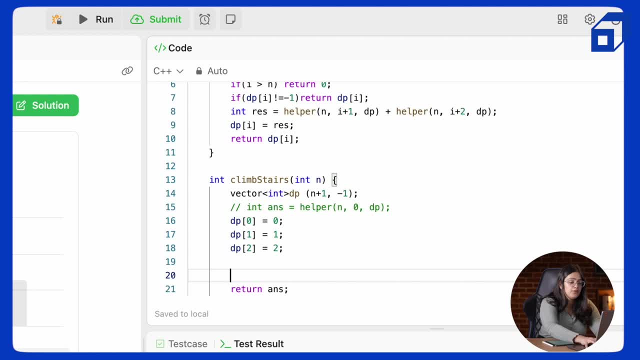 2 with 2.. These are the base cases that we already discussed. For the other cases we'll just put a for loop. we'll start from i equal to 3, we have to go till n value and we can do an i++. 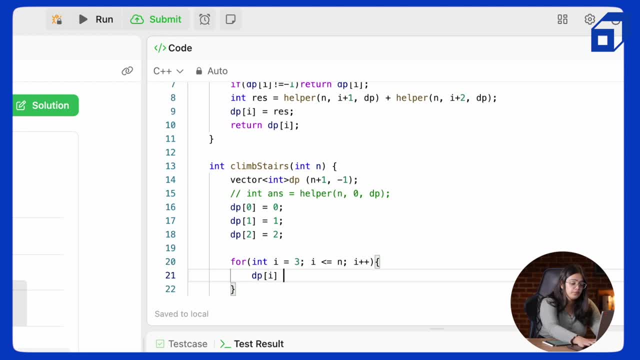 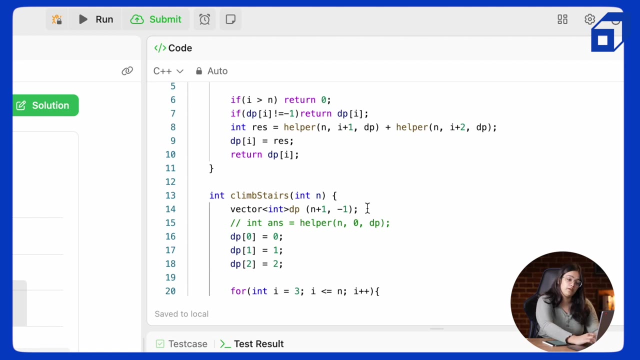 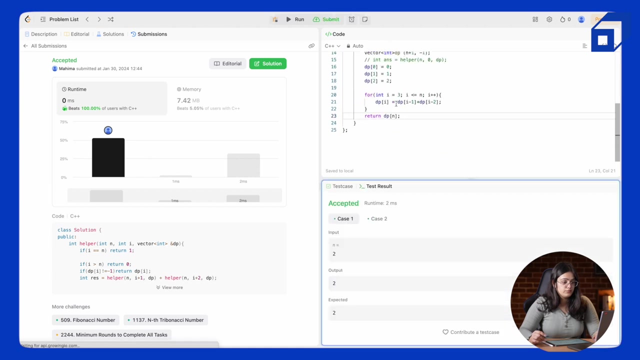 So here dp of i would be equal to dp of i-1 plus dp of i-2, and at the end we can just return dp of n. That's the desired answer, the number of ways there are to reach n. Let's quickly run this code, yeah. 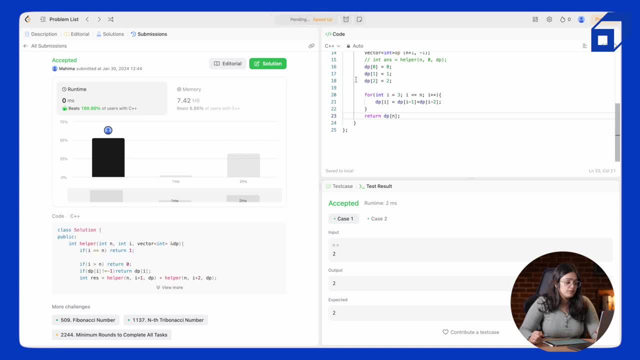 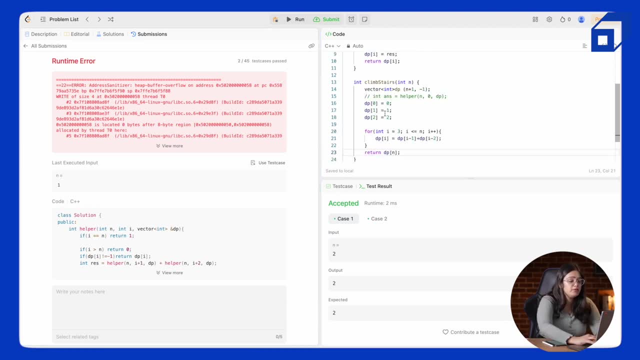 Let's submit it, Okay. So it's giving error. it's giving runtime error. That's because when n will be 1, we should not fill up dp of 2 value, because it will be out of bounds. So in case n is equal to, you know, let's say 0 or 1 or 2, we can also simply write. 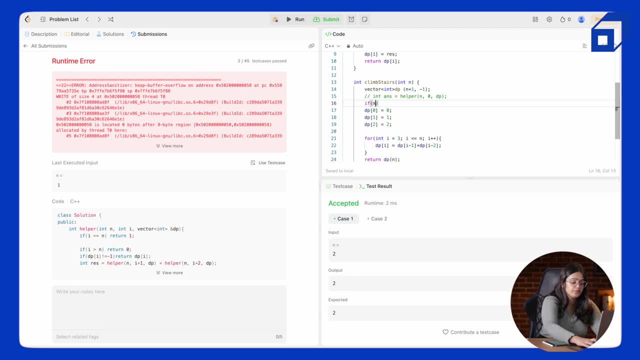 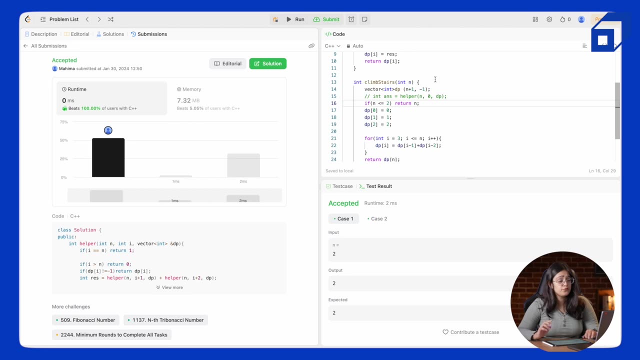 a statement: if n is less than equal to 2, we can return n. Now it should work. Okay, Yeah, so it got accepted and this is the tabulation solution. So for this particular problem, we discussed the recursive solution, which was of complexity. 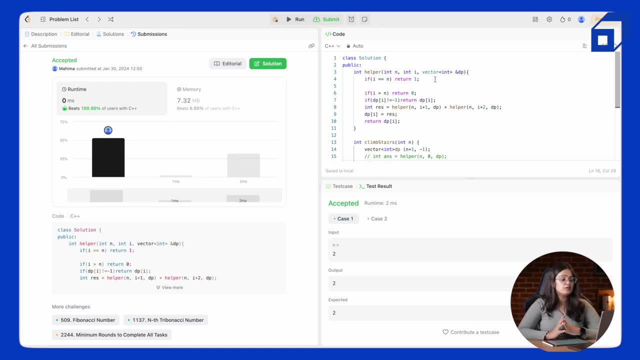 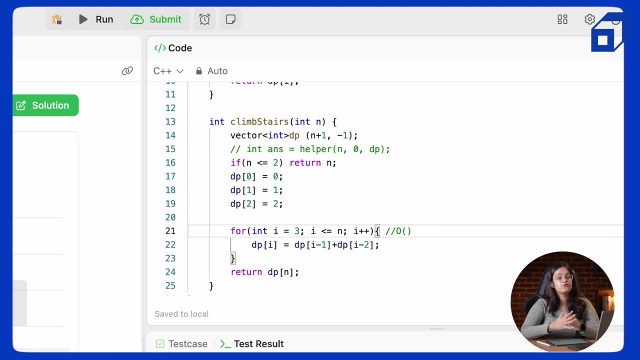 2 to the power n and which was quite inefficient. We discussed the memoization solution which was O of n in space and time complexity. So even the tabulation solution which has a for loop of length n, the time complexity will be O of n here. 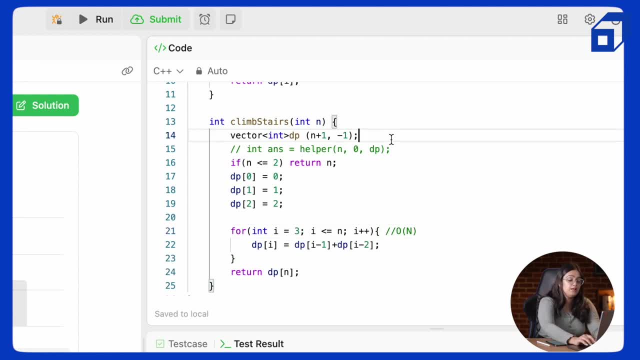 Okay, Okay. So the time complexity will be O of n as well, because we are making a vector of size n. So these were the three solutions for this problem. Now let's move on to the next problem. So let's discuss the problem. minimum cost- climbing stairs. 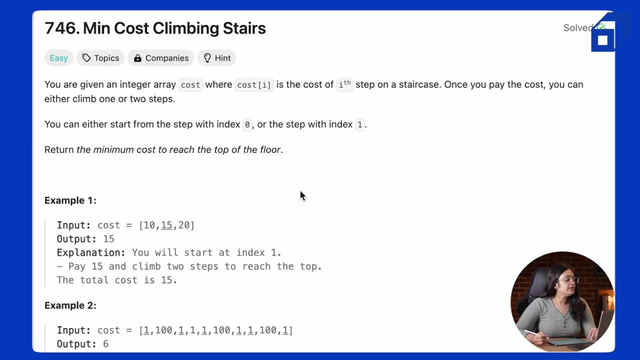 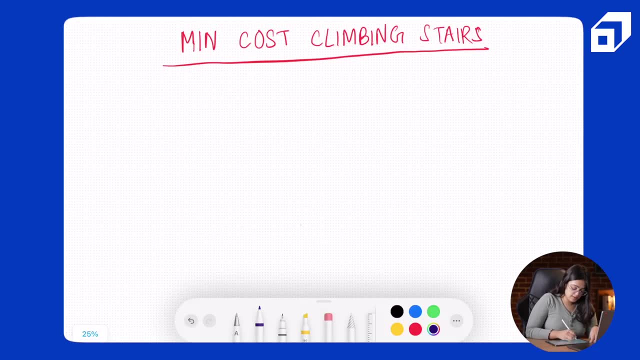 So we're given this problem on lead code and it says: you're given an integer array cost where the cost i is the cost of i-th step on a staircase. So there's a staircase and it's the cost for climbing every step. Okay, 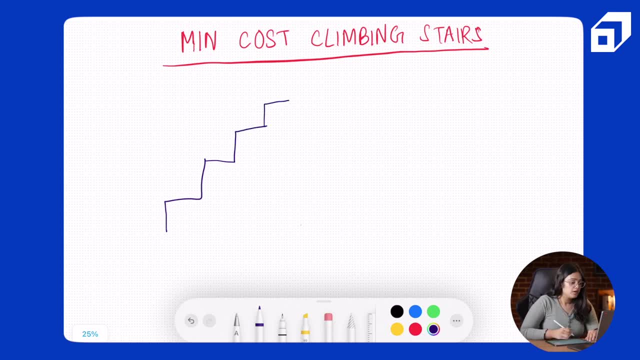 Every step of the staircase is given. Once you pay the cost, you can climb either one or two steps And we okay. So let's say we have. let's consider the first example. We have three stairs and the cost of climbing them is 10,, 15 and 20.. 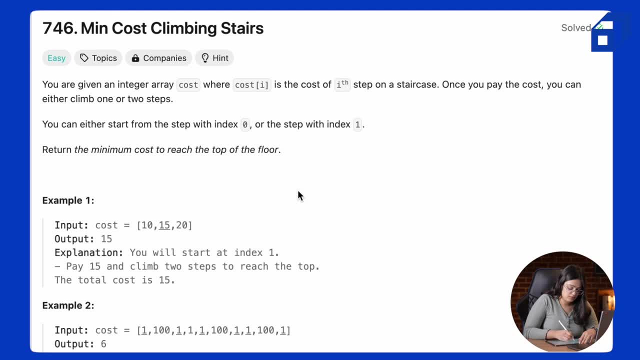 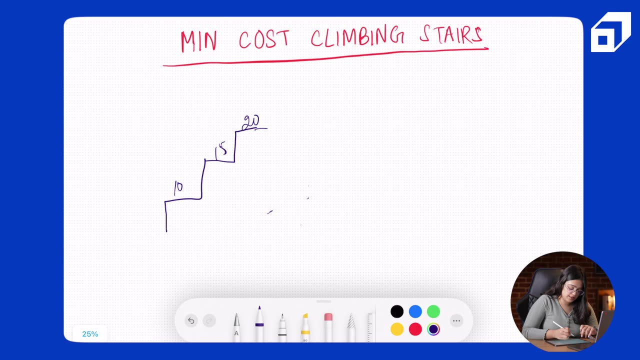 So it's 10,, 15 and 20.. Okay, Now they say that we can start from the 0th index or the first index. So essentially, the index 0 is this one. We can either start from this stair or we can start from this stair. 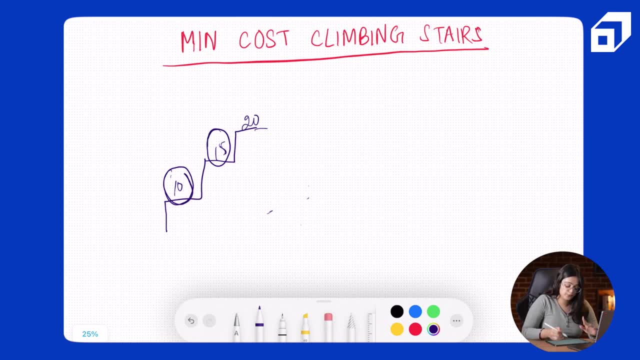 And we have to reach the top of the staircase, the top of the floor. So we have to climb all the stairs and reach here. So here Now we have to return the minimum cost to reach the top of the floor. So, as it is said, we can. so there are two things. 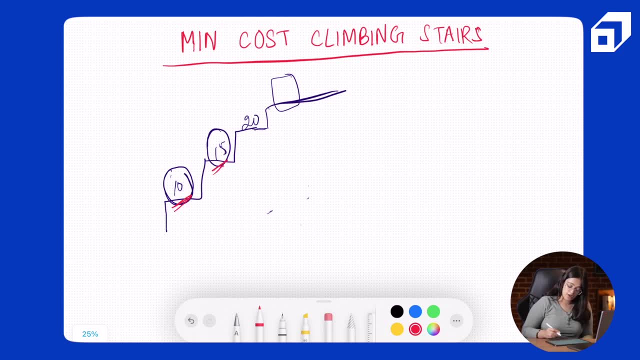 Either we can start from 0th or we can start from first. One is this: And then we can either take one step every time we climb, or we can take two steps every time we climb. But irrespective of that, the cost of climbing that stair or starting from that stair will. 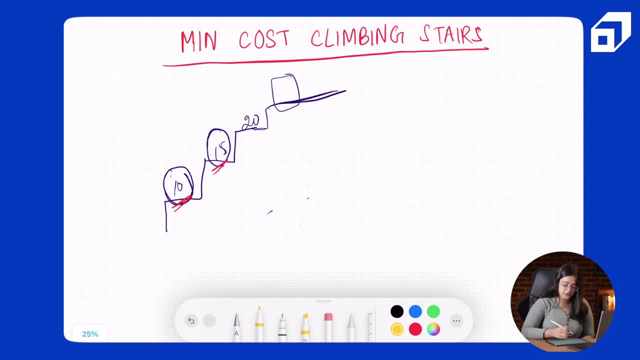 be the same. That is the value present at that index. Okay, So if I start from 10, I can either go to this stair or I can go to this- The cost will be 10 only, Right, So what I can do is let's see what all ways are there and how much cost it will take. 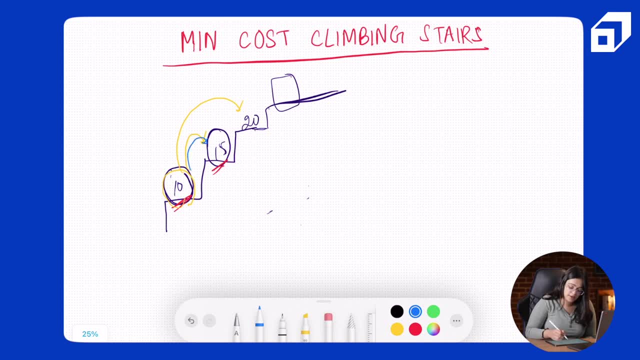 If I start from 10 and if I take one step, it will cost me 10.. Then I start from 15 and I take one step, it will cost me 15.. And then I again go to the top of the floor from 20.. 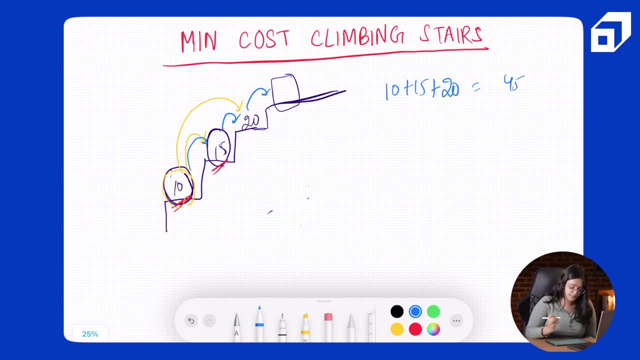 Okay, The cost will become 45.. The other way is so: starting from 10, taking two steps will be 10, because the cost is same irrespective of the number of steps you are taking, And then, after reaching here, the cost will be 20 again. 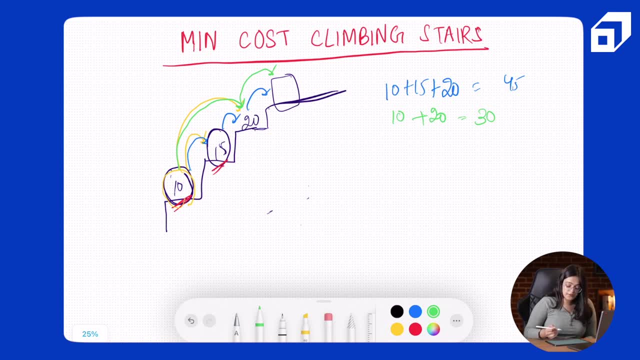 So it will be 30.. Another way is: so we started from 10, right, There was another thing in the question. But we can start from index 0 or index 1.. So now let's start from 15.. So if we start from 15, I take one step- the cost will be 15.. From 20 again, I take another step, the cost will be 20.. The cost is 35. or if I start from 15 and take two steps directly, the cost will be 15 only. Out of all these possibilities, the minimum cost comes out to be 15.. 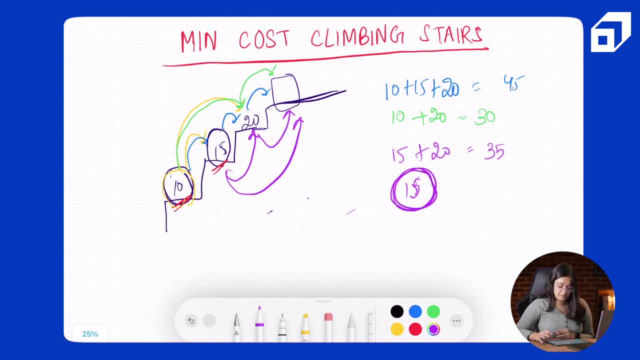 So that's supposed to be our answer. So I hope the problem statement is clear. Two things are there: either take one step or take two step. And for starting, you can either start from index 0 or start from index 1.. 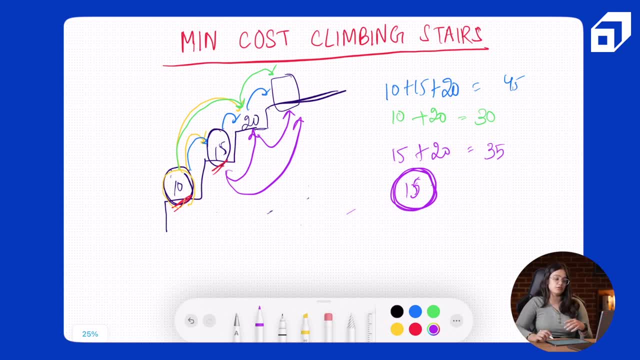 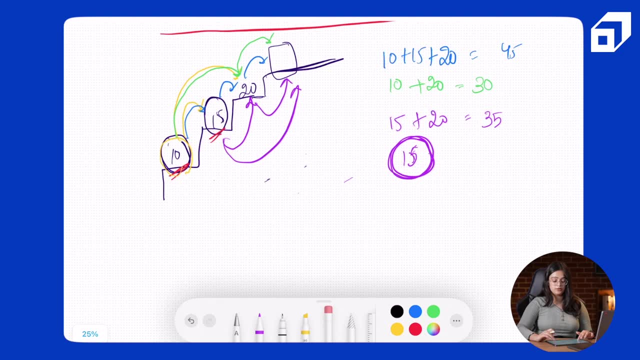 We have to reach the top of the floor and we have to find the minimum cost to reach there. So that's the explanation of this problem, And now let's try to figure out a solution for the same. So, as we did in the previous problem, this will also have a recursion. 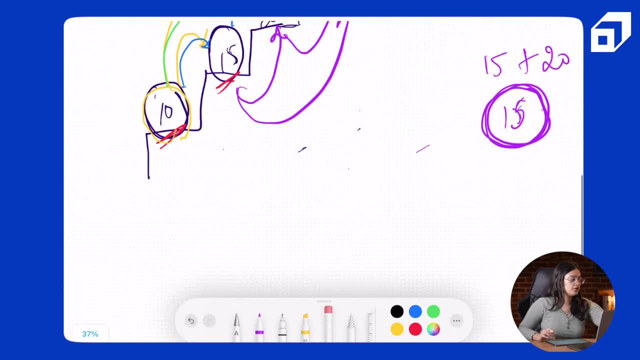 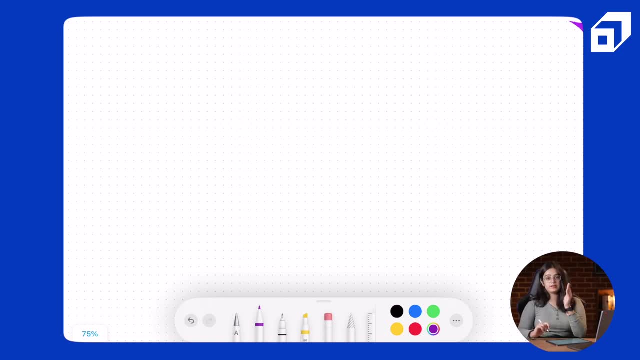 Okay, Okay, So we have a recursion chart, a recursion tree. So for the recursion tree, we have two things. We have either we can start from 0th index or we can start from 1st index, And the answer would be the minimum cost that will come from both of these spots. 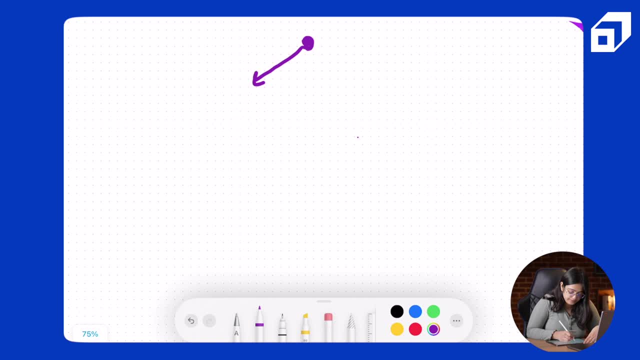 So either we start from the 0th index or we start with the 1st index. The value at 0 index is 10.. The value at 1st index is 15.. Going down both these spots, so here at every index, we can either take one step or we can. 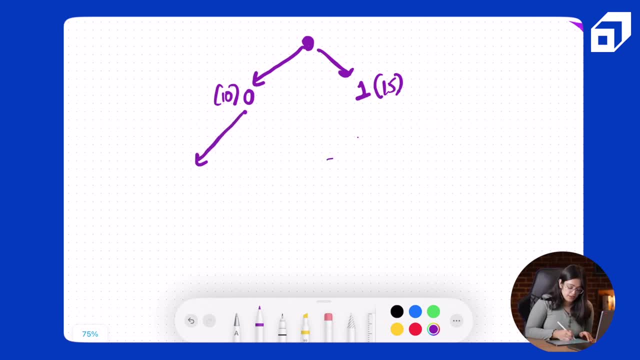 take two steps. If we go one step down from 0,, we reach 1.. And if we go two steps down from 0,, we reach 2.. So when we go again from 1, we either take one step, we reach 2 or we take two steps. 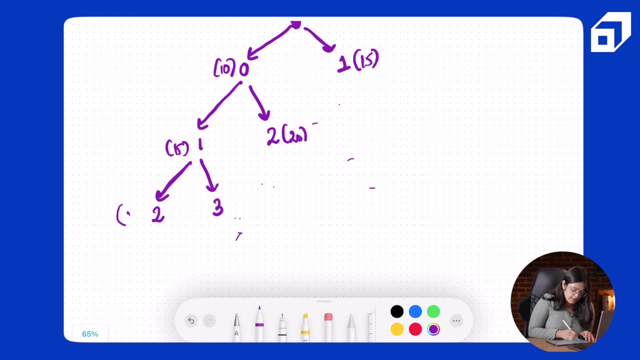 we reach 3.. Okay, Then again, 3 is one of our solutions. 3 is like we've reached the top of the floor, So this is one valid solution and we can calculate the cost of it. So here it will like we've reached one of the base cases. 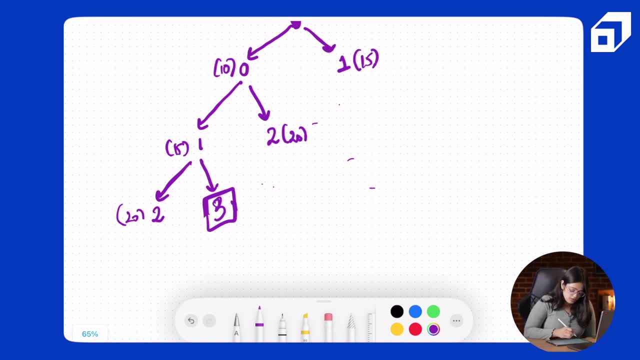 3 is the base case, since we have to reach index 3.. So it will return the values up top, So this will return, let's say, at 0.. Okay, Okay, So at 3, there's no cost, so this will return 0. 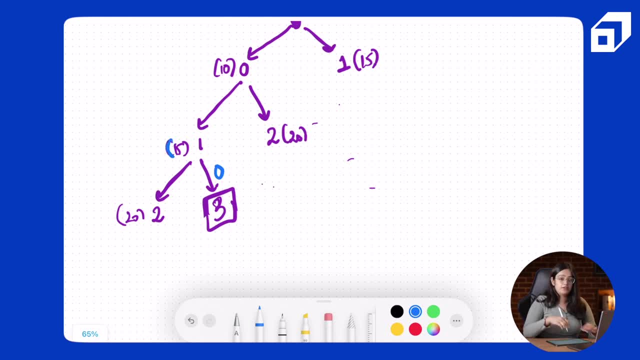 And here 1 will return. 1 will have taken the cost of 15.. So 15 here and 10 here. So this particular path has the cost of 15 plus 10, 25.. Now, continuing over the other paths, after 2, we can go. we can take one step and go. 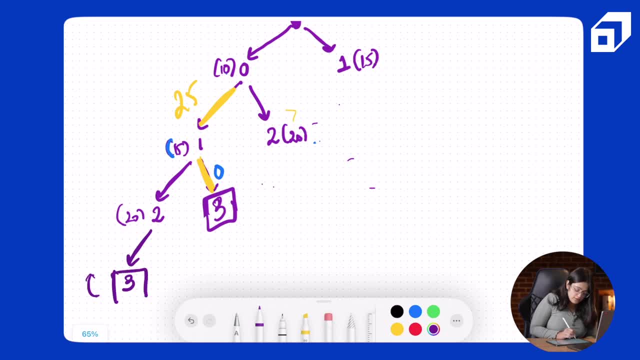 to 3.. And this is our one of the goal. again like this is the top of the floor again. So this is one of the paths And if we take two steps, we reach 4,, which is out of the bounds. 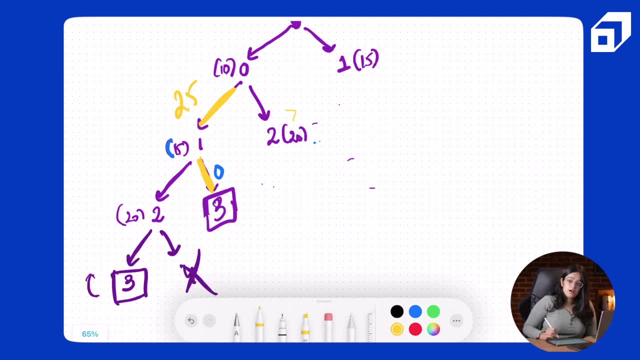 So this is a discarded solution And if we check a path that we've reached again, this is reaching from 2 to 3 and 1 to 2.. And here is 0 to 1. So it's 10 plus 15 plus 20.. 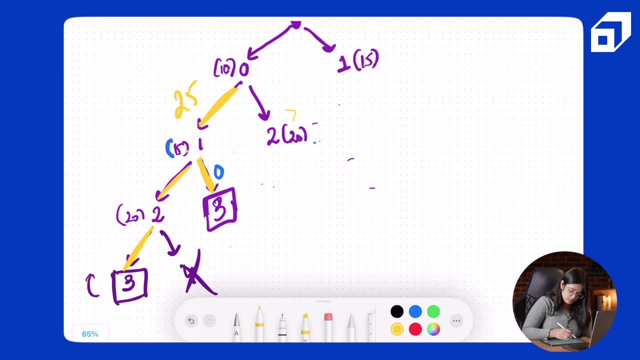 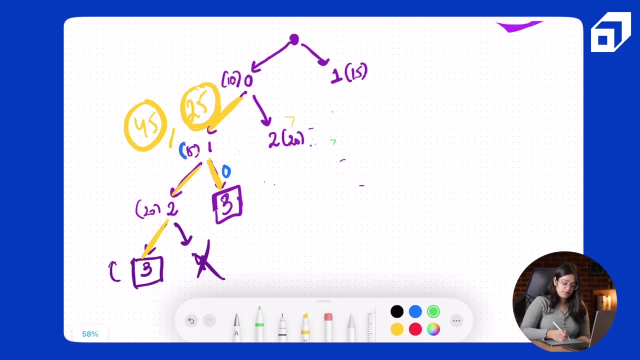 So it's 45. So another cost we've gotten is 45. Since this is the minimum. so we've got two answers when we started from 0.. One is 45 and one is 25.. So the answer is like the minimum here till here is 25.. 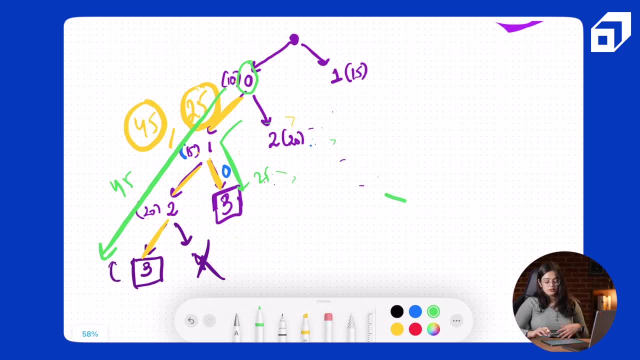 We've yet to explore other paths, But the gist is that we'll keep exploring the recursive path, Okay, And we'll find the minimum that comes from either of the sides. So even if we go on 2 again and we find one answer, that will come out to be, let's just 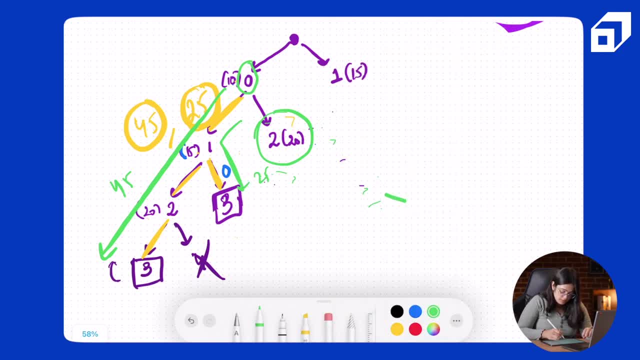 quickly make this recursion chart complete. So from 2, we can go to 3,, we can go to 3,, which is our final answer, or from 2, we can go to 4,, which doesn't make sense taking two steps. 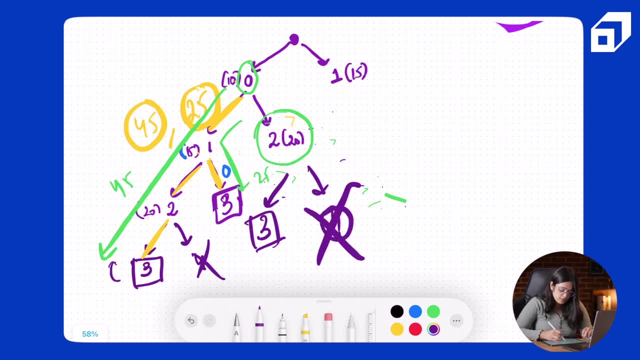 So this is discarded And this gave us a cost of 20 plus 10, which is 30. And if we start, if we start on this path. so we took a cost of 15, starting from 1.. We can either go to 2 or we can go to 3.. 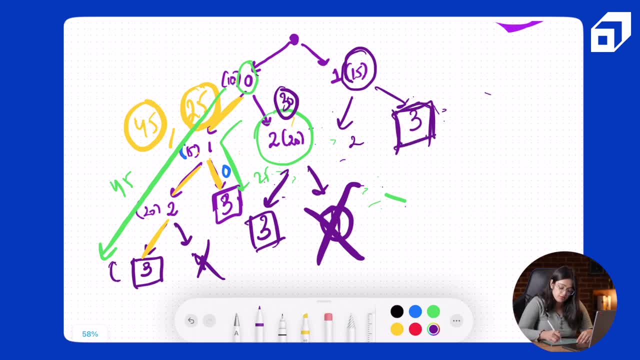 This is one path, And this returns a cost of 15.. From 2, again, we'll calculate the cost, but the minimum costs will be this one only. So this is how the recursion tree for this problem would look like. All right. 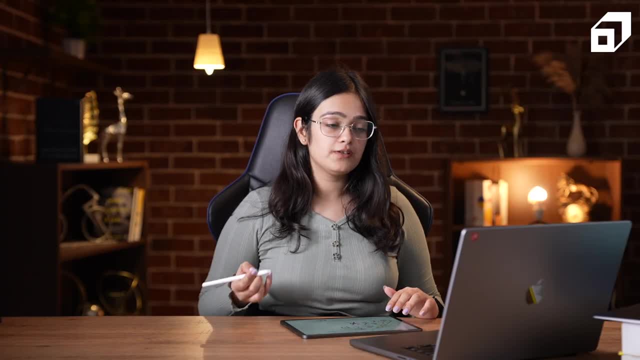 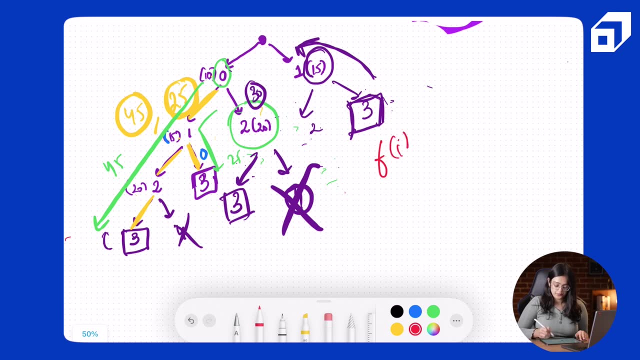 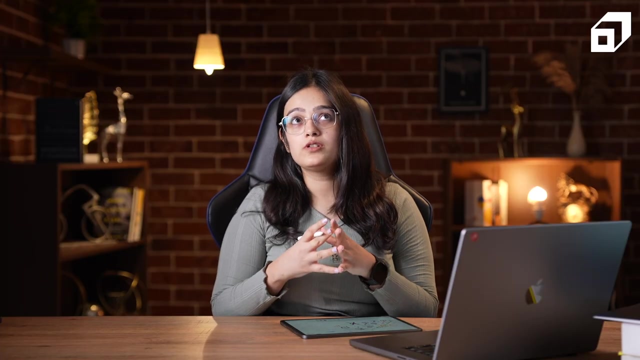 Okay, So let's write a generic recursive equation for a generic i value For any particular i that we are at. we're looking at what if, like, what's the number of steps, what's the minimum cost, what's the cost that incurred if we take one step and 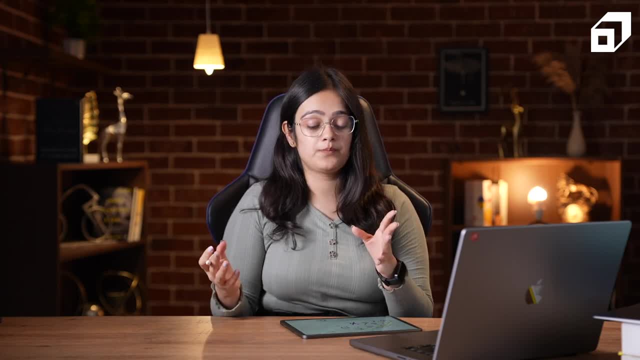 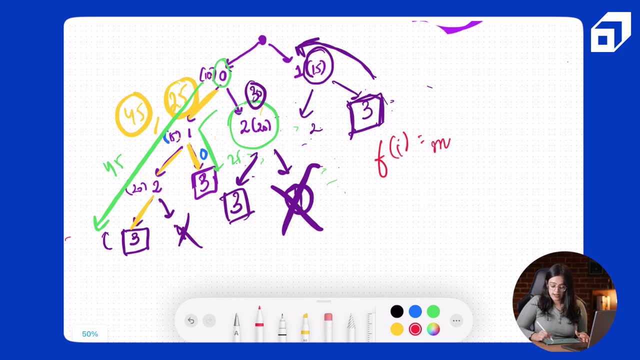 what is the one that that's incurred when we take two steps. So either we start with one step or with two steps, but at the end we take the minimum of both. So our equation will have the minimum of whatever we get after moving one step. 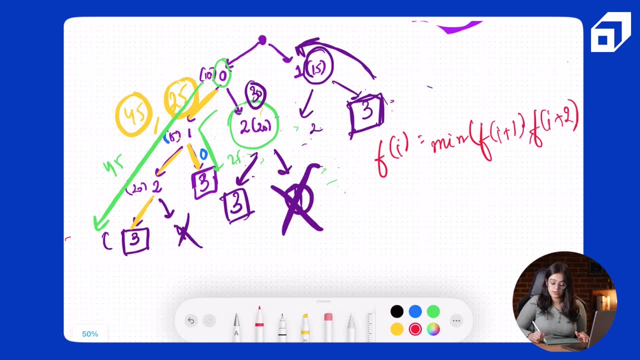 and whatever we get after we move two steps plus, we'll also be adding the cost at that particular position, because that's the cost that's required to take one step or two steps. So this is the generic equation. We can also write it in just the opposite way. So to reach, 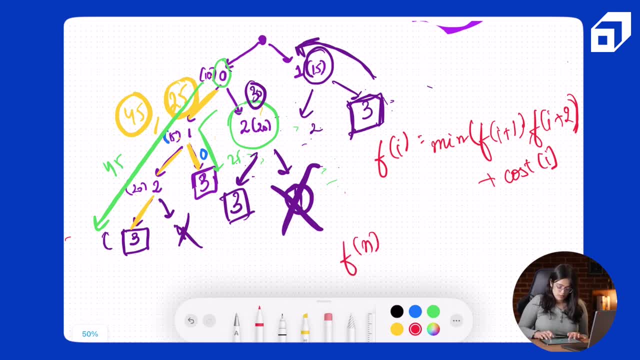 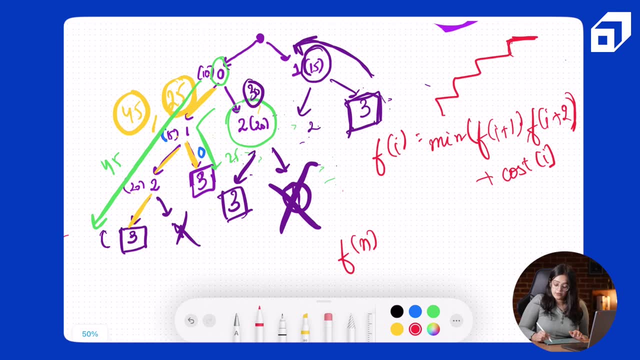 at any point n. So let's say these are our stairs. So to reach this point, either we'll have to come from one step lower or we'll have to come from two steps lower. So the answer will be minimum of f of n minus. 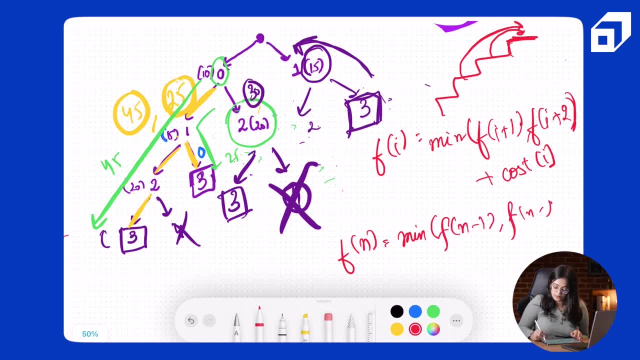 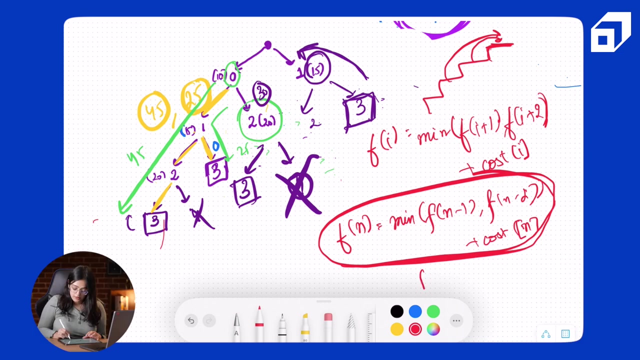 1 comma, f of n minus 2 plus cost of n, because that's the cost that will take to move from n. But keep in mind that this is for any generic value for of i. But the final answer will be always the minimum of f of n minus 1 and f of n. 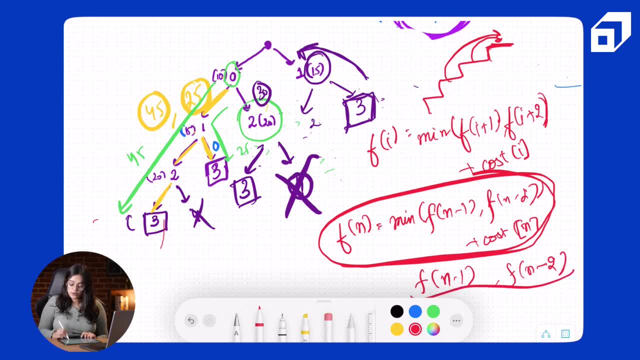 minus 2, because these are the two places where we can reach the top n, the top floor. So our goal is to reach to the top floor and the answer for n will be minimum of n minus f, of n minus 1 and minimum of f of n minus 2, because 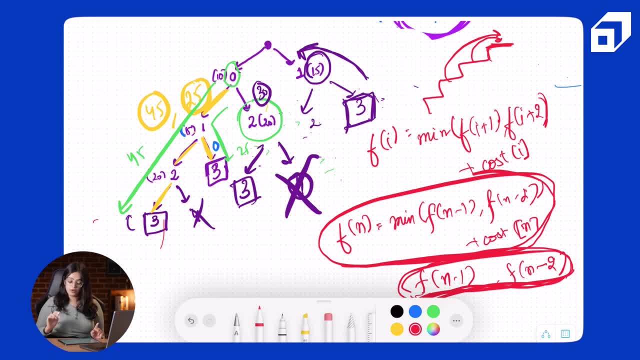 there's no cost to go from the top floor to anywhere. The top floor is already our answer. So this cost of n factor will not be there in the last, like when we are, when we are considering for n But for all other generic values, the answer. 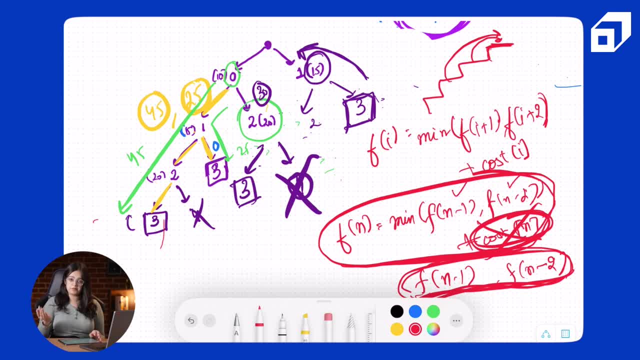 would be f of n minus 1 plus f of n, minimum of f of n minus 1 and f of n minus 2, and we'll be adding the cost of n. So our base case here will be n equal to 0 and n equal to 1, and for n equal to. 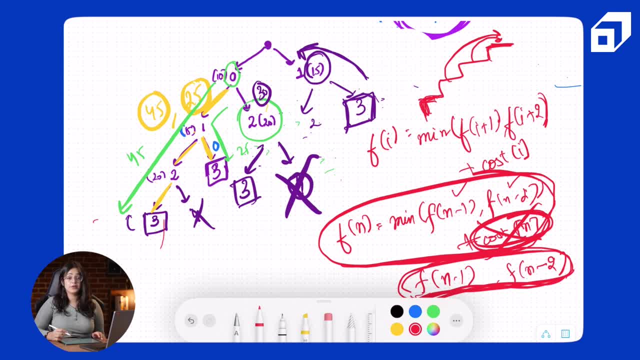 0, the cost would be cost of 0. That's the value present at the 0th index of the array, and for n equal to 1, the answer would again be cost of 1.. That would be given in the cost array. So, moving on to 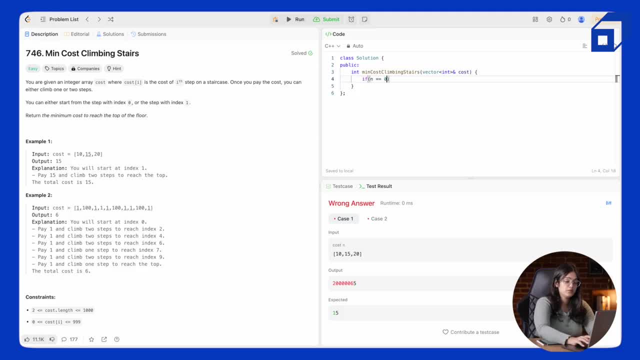 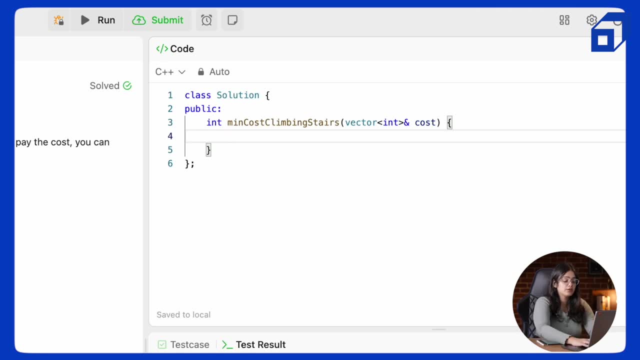 the code: if n equal to equal to 0.. First, just quickly, let's write the helper function and get the value of cost dot size into n. So let's just say n equal to cost dot size, We have to calculate the minimum cost. 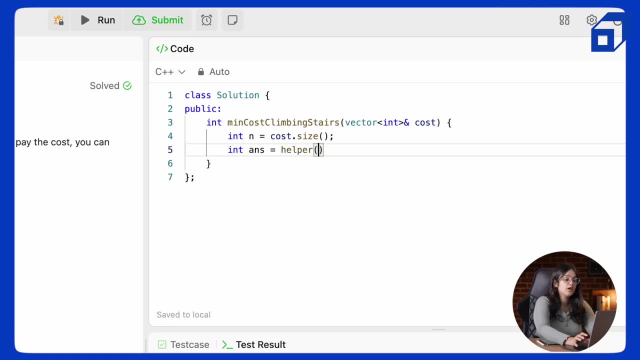 I'll just get this and get the answer from a helper function and store it in answer variable. So I will call the helper, I will pass on the cost, I will pass on n, I will pass on the i value we are on, So we have to calculate two. 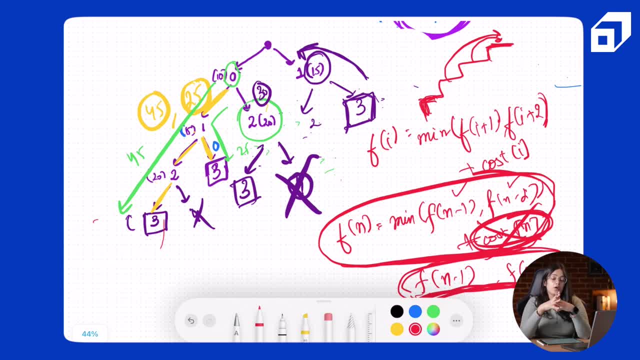 answers To reach n. we either come from n minus 1 or we come from n minus 2.. So here, instead of calling it for one value, I call it for two values. I call it for n minus 1.. I call it for n minus 2 and I. 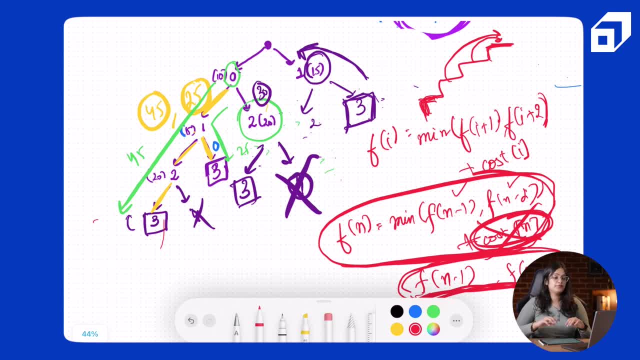 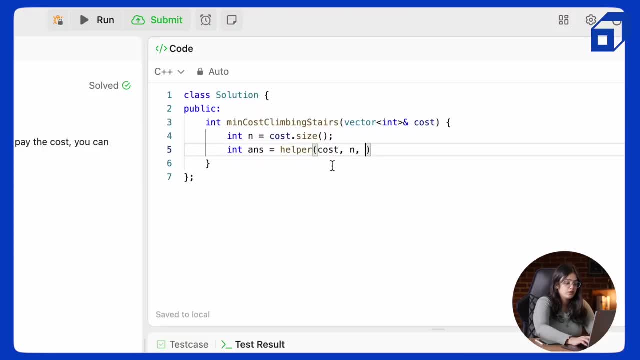 take the minimum of both of them, And we already discussed that. for n, the answer would be the minimum of n minus 1 and n minus 2.. And the cost factor wouldn't be there because it's zero. So cost n and I will pass on n minus 1.. I will take the. 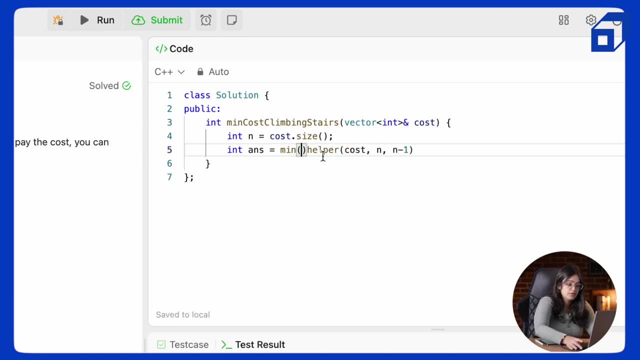 minimum of two calls. So minimum of helper this and cost n, n-2, and we'll return this answer. Now let's quickly write the helper function. The helper function is taking this cost vector. it's taking n, which is the size of the cost vector, and it's taking the value i, the generic value. 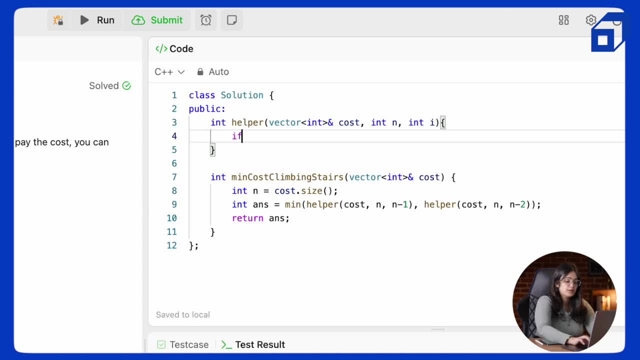 that would be Now, as the base cases we discussed were n equal to equal to 0, where the answer would be cost of 0, and if n equal to equal to 1, the answer would be cost of 1.. For the rest of the cases, we can return cost of i plus helper. 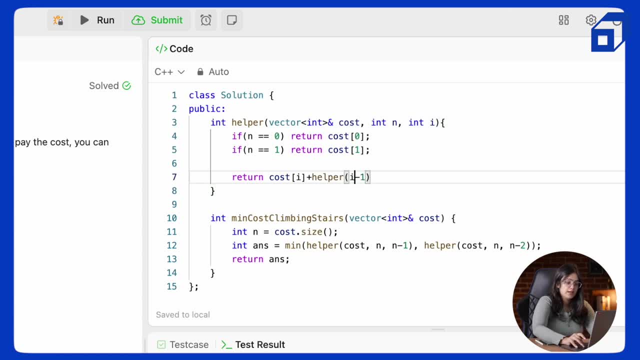 of i-1, that is, we'll be passing on cost n and i-1 and we'll have to take, as we discussed. we'll have to take minimum of two calls: one for the i-1th value and one from the i-2th value, if a person is coming after taking two steps. 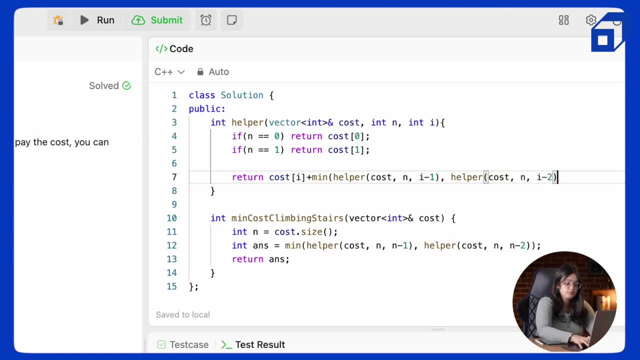 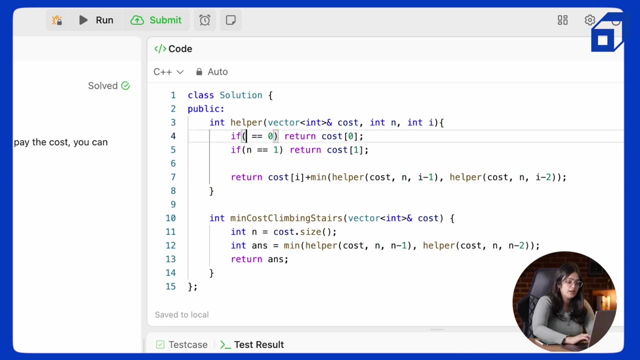 Yeah, so adding cost of i, the current cost plus the minimum of one step or two steps, whatever is there, and we can run this code Before that. here we have to write i equal to equal to 0,. here we have to write i equal to equal to 1.. So if we are, 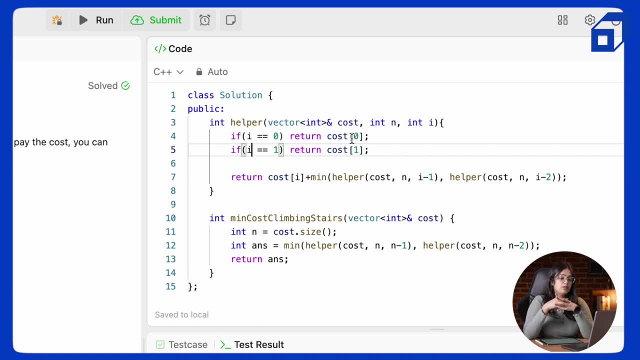 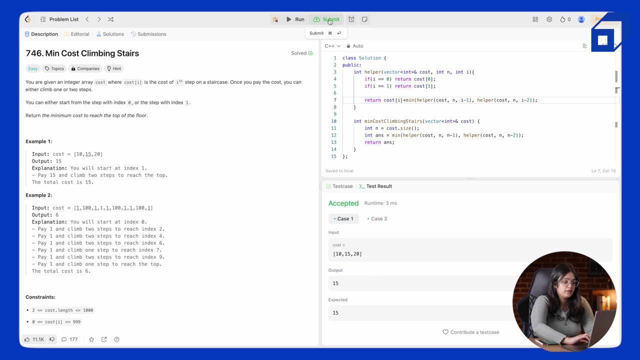 finding the answer. for 0th, it will simply be the cost present at the 0th index, and for 1 it will be the one present at the first index. So we'll just run the code now. Yeah, it is accepted. and now let me try and submit the code. 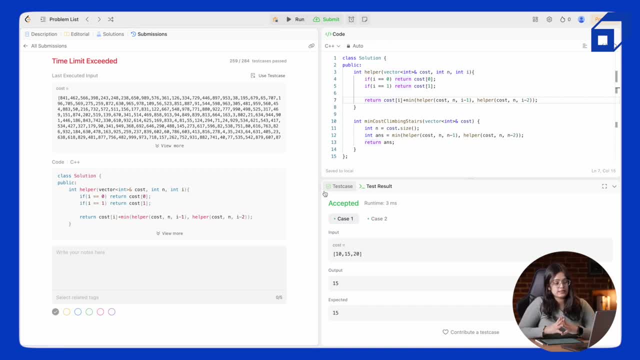 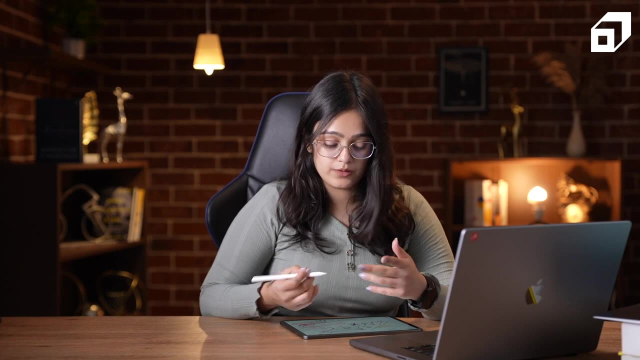 Yeah, so it works for most of the test cases, but it's giving time limit exceeded in certain other ones and we know the reason for that, as we discussed earlier that we're passing repetitive calls for certain values. So we can optimize this like we did in the last problem: we can first Memoize it. 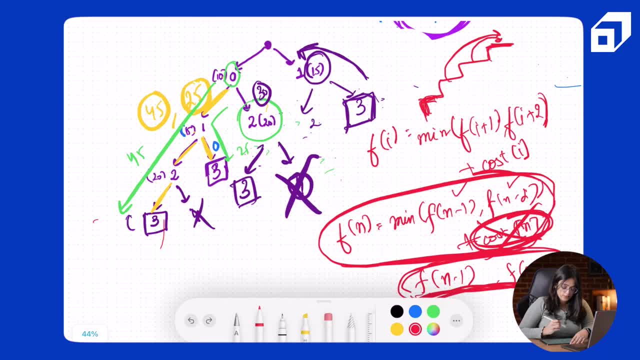 So, as you see in this problem that there was certain repeating cases, like 2 was present here as well and here as well, And it's they're overlapping subproblems in this question. so, like we did in the previous problem, so whenever we found a value for any index, we stored it in a Memoization table. 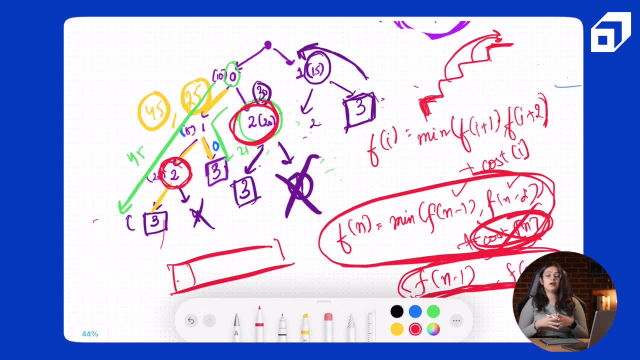 in a Dp table And whenever we come again to that value, we first check that if if the answer was calculated for this particular index- and it was calculated- we just reuse the answer. so, like the previous problem, we'll just initialize our DP with minus 1 and, as in when we 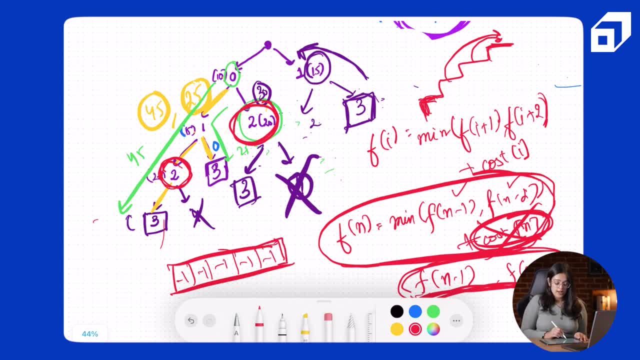 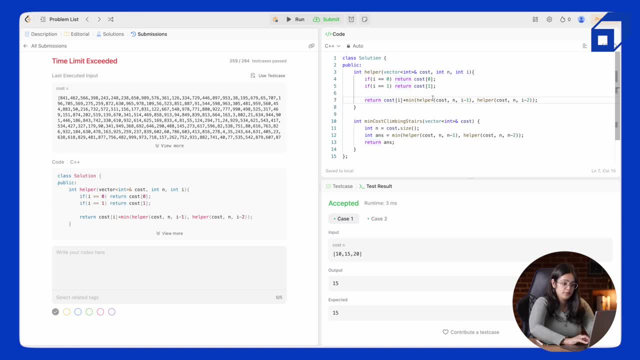 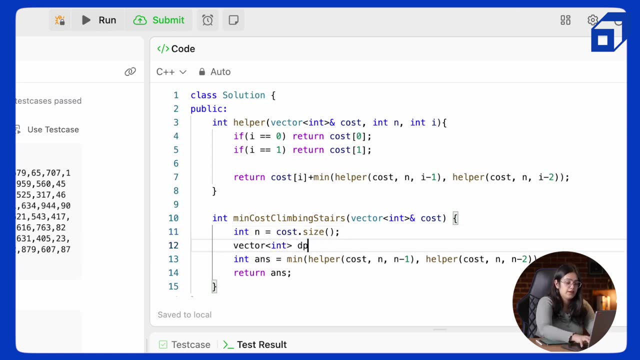 calculate the answer, we'll store it in the DP table and while calculating it again, we can just refer to the old answer. so I'll quickly memorize our already written code. let's create a DP table. it will have a size of n plus 1. let me initialize it with minus 1 and I'll pass this on in our helper function. 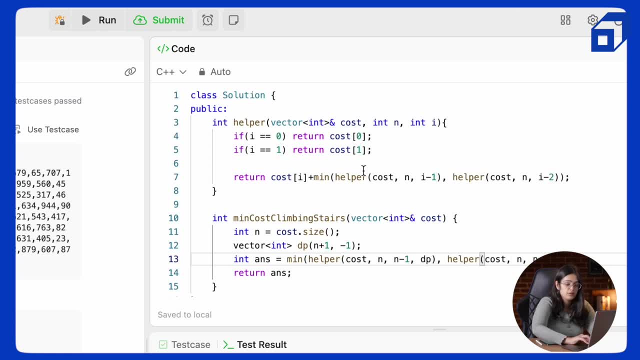 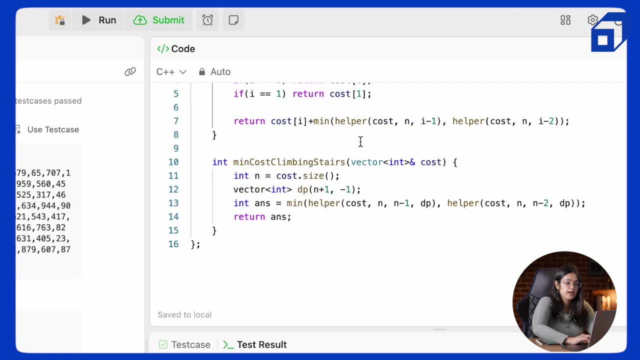 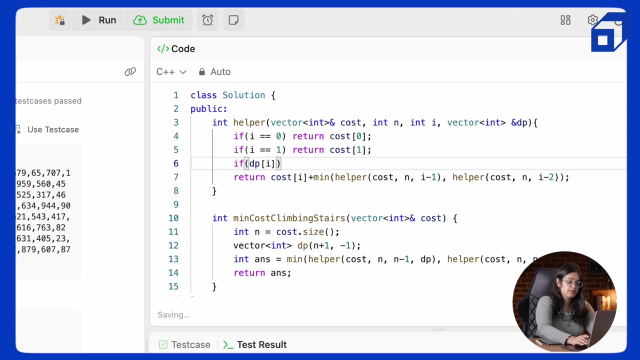 calls. we pass it by reference and before calculating the value for any particular, I will check. if dp is not equal to minus 1, which means if it's already been calculated, we'll just return dp, and if it's not been calculated yet, if it is equal to minus 1, then we calculate the value, will store it into the dp table. 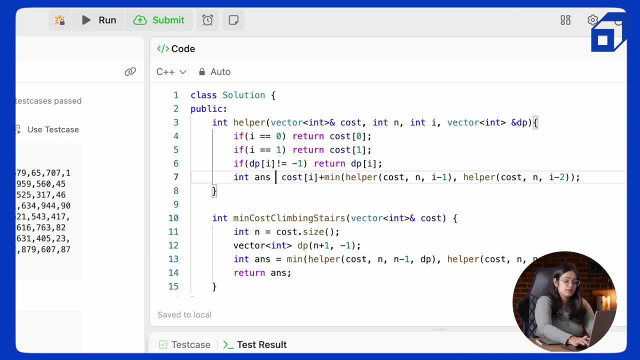 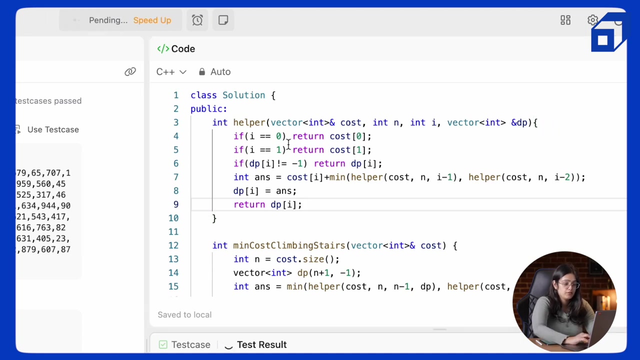 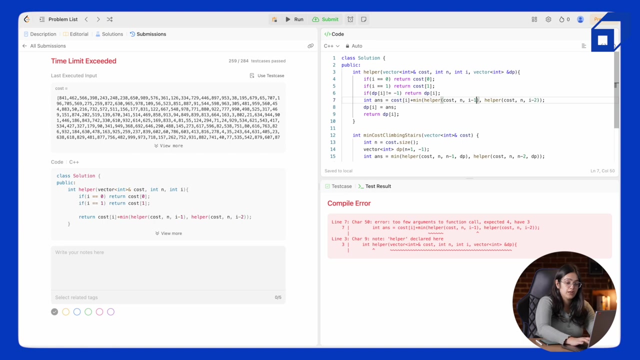 and then we'll return it. so let's just say I'll store it in this answer, I'll populate the DP table answer and I'll return the dp of i. So let's see if this runs well. Okay, we have a quick error, so let's just pass on the dp parameter here as well. So it got accepted and let's 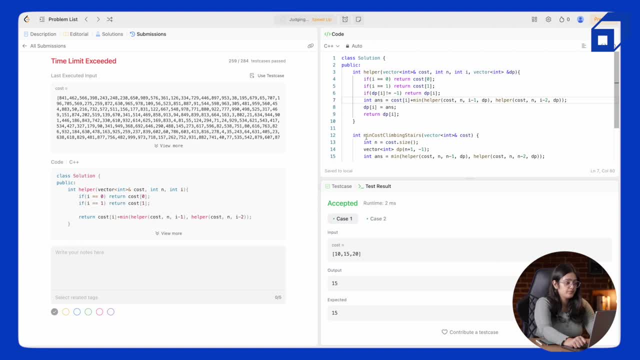 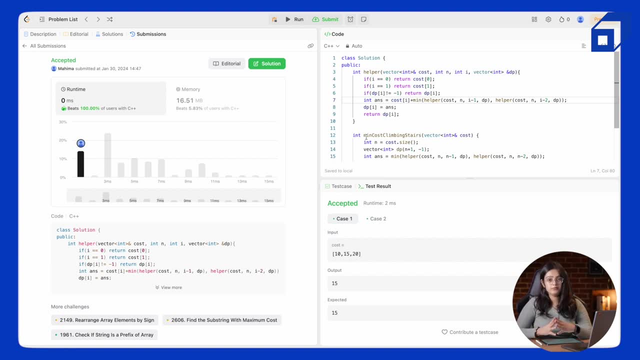 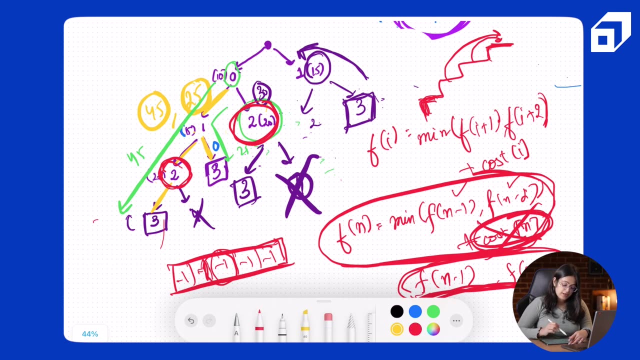 submit the code. Yeah, so it got accepted and the time limit exceeded is not coming again, because the time complexity is significantly opposite. Okay, optimized, Like the last problem. we'll see here that whenever we are encountering a same value, we are not calculating the answer again and we are 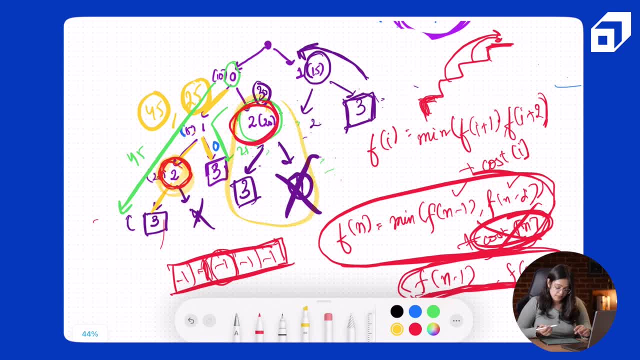 storing it in the DP table. So the repetitive calls are saved, and for every value we are calculating it only once. So the time complexity of this solution is O and the space complexity is also O because we are maintaining a DP table of size n. So now let's move to the tabulation solution for the. 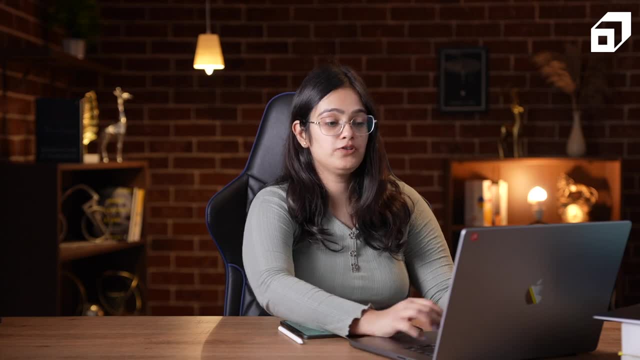 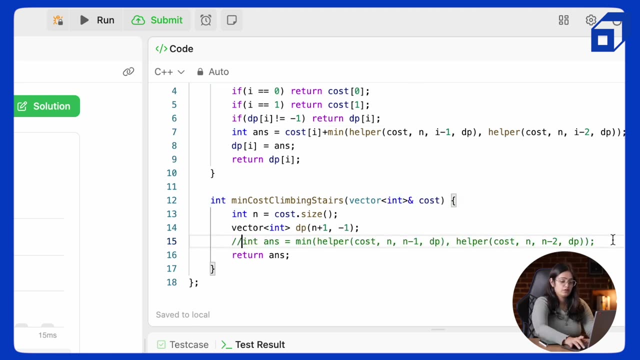 same problem. So instead of making another helper function, I will just write my for loop here itself. I'll comment the existing code. I will write a for loop. Before that, I'll initialize this DP table for our base cases. So, as we always. 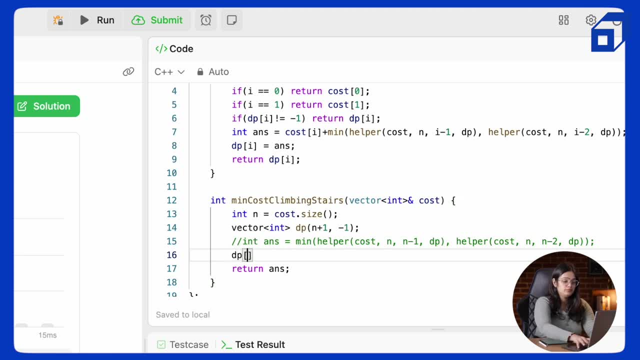 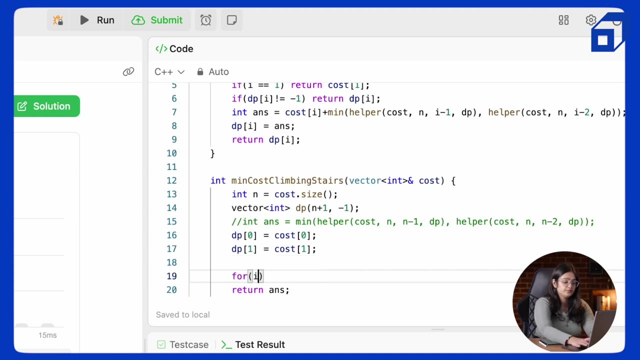 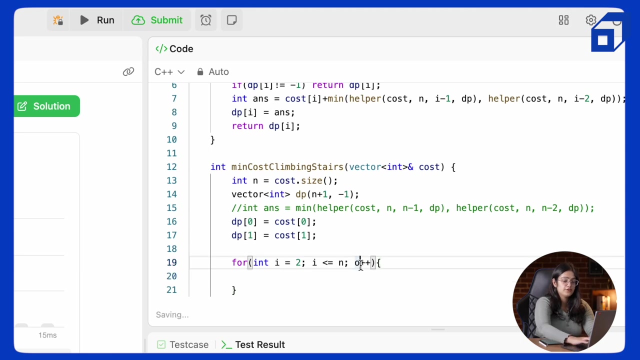 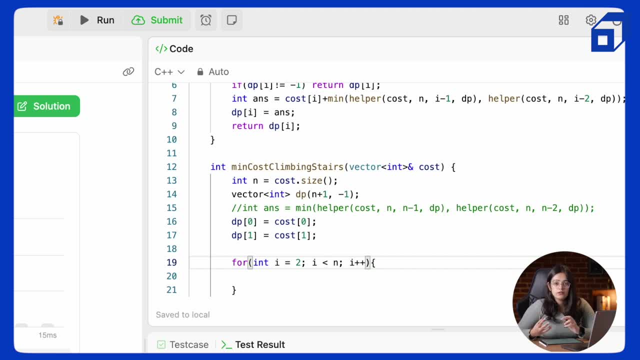 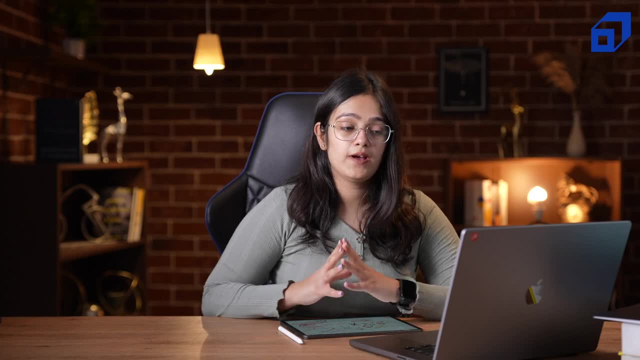 at the end we need to return the minimum of DP of n minus 1 and DP of n minus 2, because those are the two places that we can reach n from. So at the we will calculate the DP till n minus 1 and at the end we can return the minimum of DP. 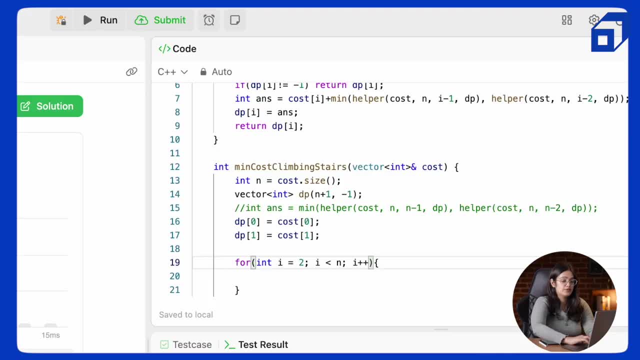 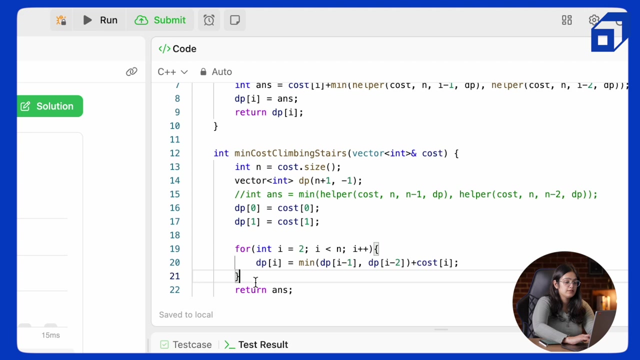 of n minus 1 and DP of n minus 2.. So I'll just write the formula for DP here. We had minimum of dp i minus 1, comma dp i minus 2 plus cost of i and at the end, instead of returning this answer variable, i will be returning minimum of dp of n minus 1. 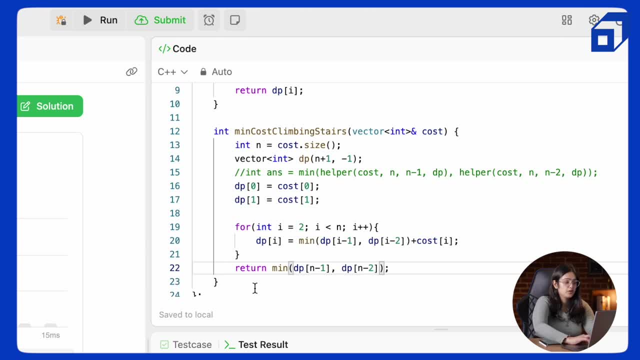 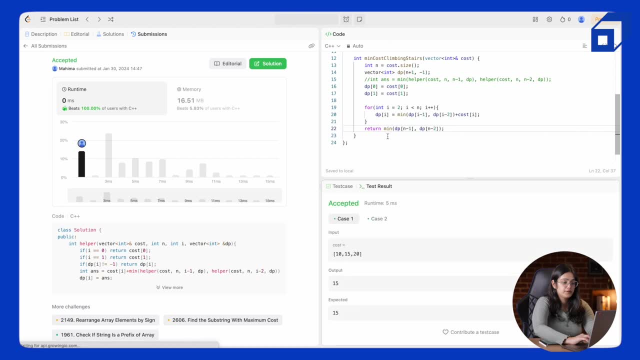 comma dp of n minus 2. i will run this solution. yeah, it's accepted. i will submit this. so it's accepted here as well. so this is a tabulation solution. this, the code, looks a lot simpler than the recursive and memoization solutions and here also the time complexity. 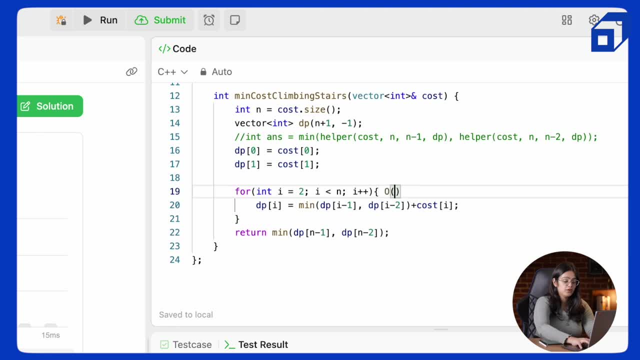 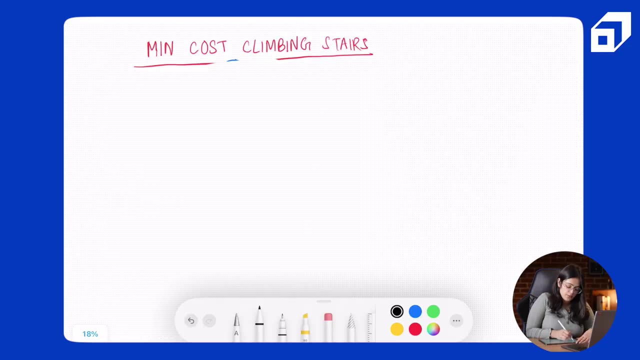 is o of n because we are using a formative, formative, formative, formative, formative, formative loop to iterate over n values, and the space complexity is o of n as well, because we're maintaining a separate array of size, n. so right now, we saw three approaches. one was 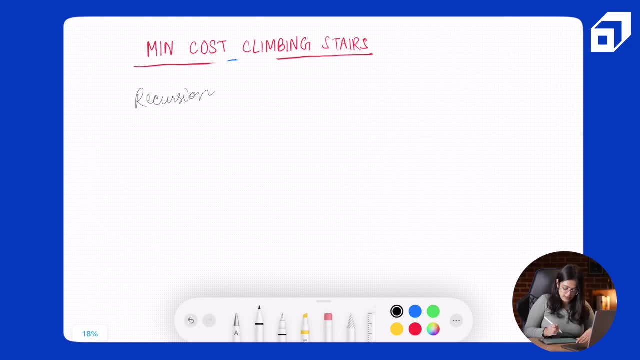 recursion, where our time complexity was of prox 2 to the power n and our space complexity was of. it was not any of external memory that we were using, but the recursion stack was taking the space and for the memoization solution our time complexity was o of n and our space complexity was also. 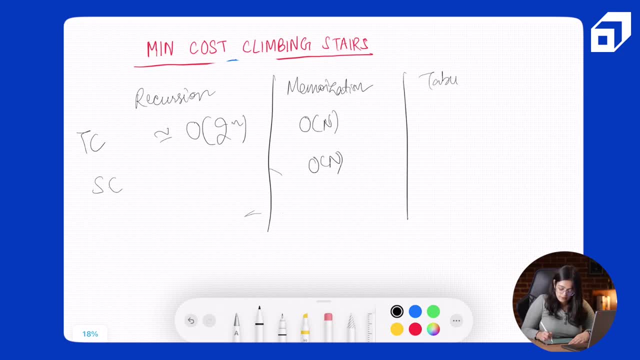 o of n for the tabulation solution again, the time complexity was o of n and the space complexity was o of n as well. this was also o of 2 to the power n. now we can further optimize the space complexity to go from o of n to o of 1. how we can do: 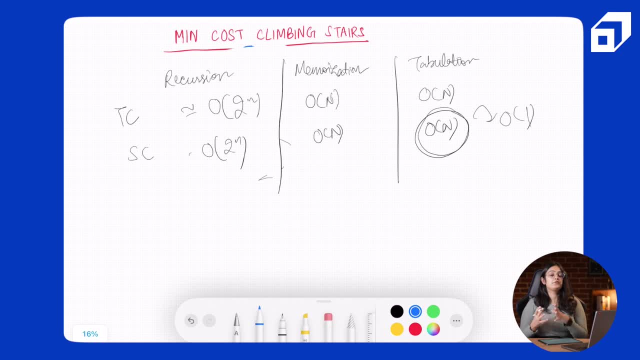 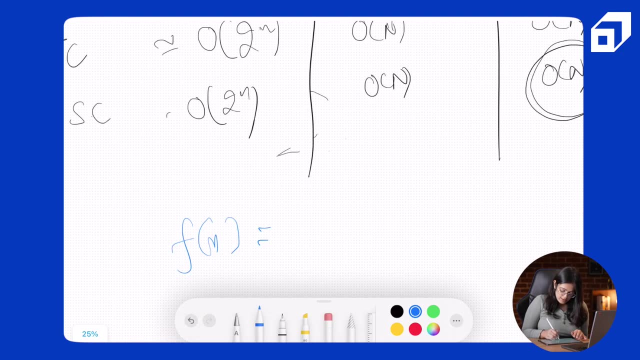 that is, if you observe our recursive equation, is f of n. this is coming out to be f of n minus 1. we are taking the minimum of f of n minus 1, f of n minus 2, and we are adding the cost of n and we are adding the cost of n. 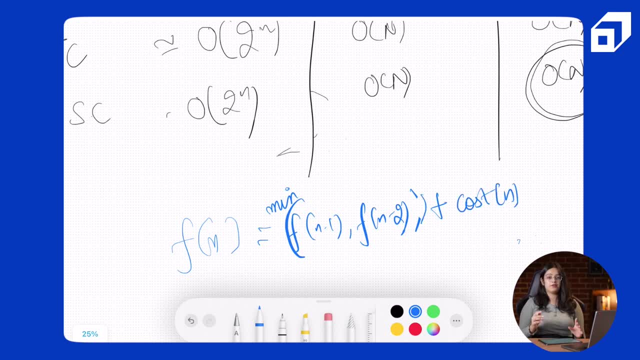 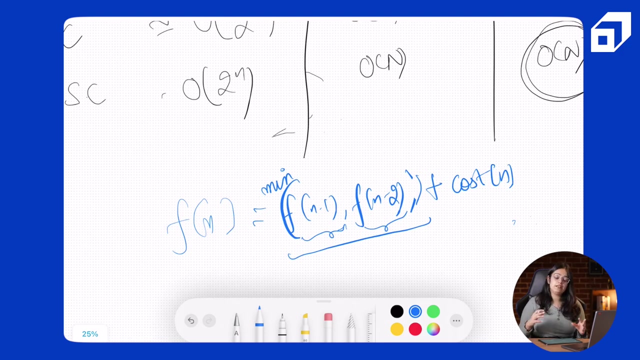 so if we carefully observe the value for any particular state, the value for any particular i is depending on the previous value, the value for the previous state and next to the previous state. so it's just depending on two previous states. so what if, instead of showing the values for the complete dp, 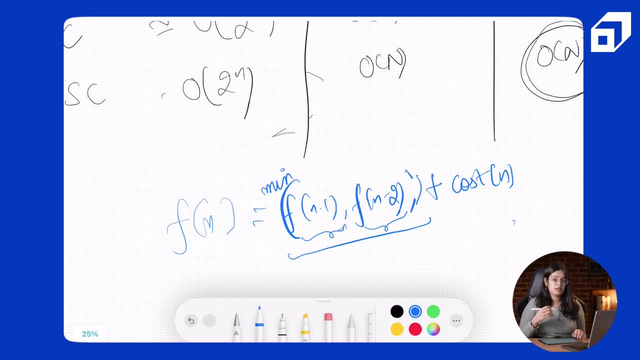 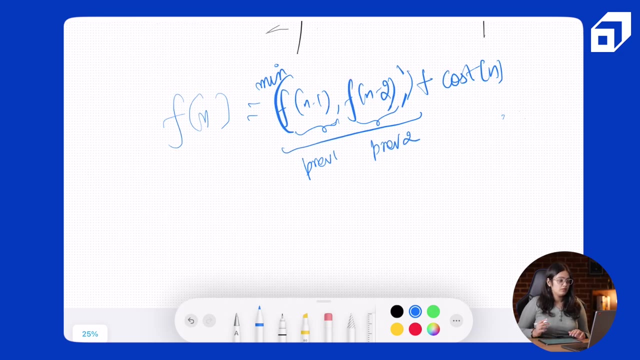 table if we go by the tabulation solution when we are making a for loop, what if we store just the previous two values, because those are the only ones that will be useful for us? so we'll be storing previous one and previous two only, like the previous one and the next to the previous one. so let's say our 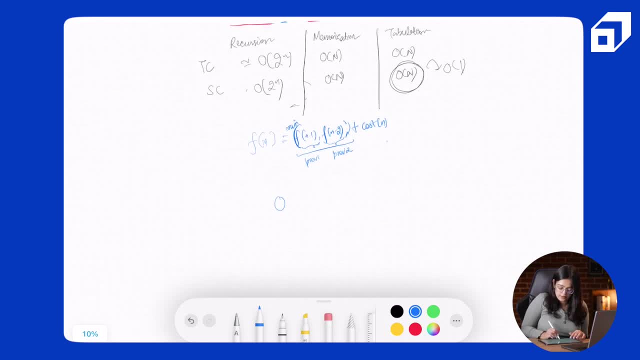 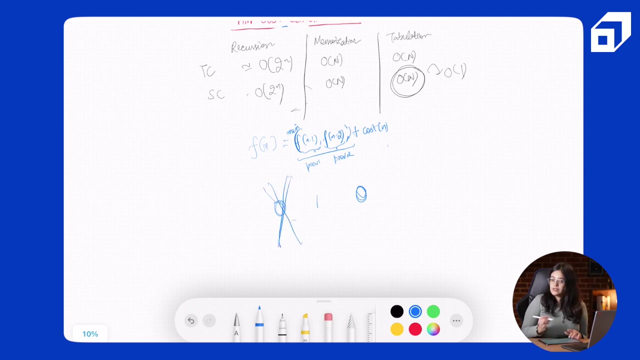 answer for you know, any particular array was 0 and 1 till till two values. so the next answer is, let's say, the minimum of these two. so we will store the next answer here and then we'll discard this one. we don't need this one because 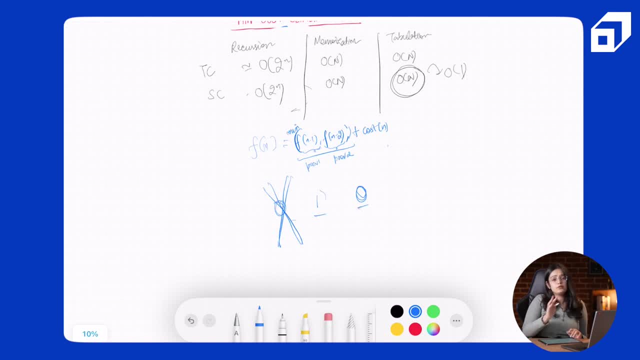 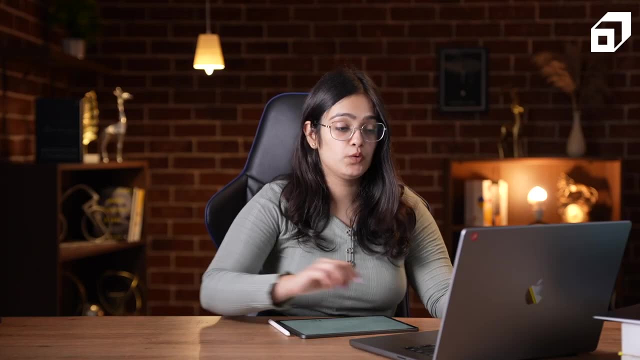 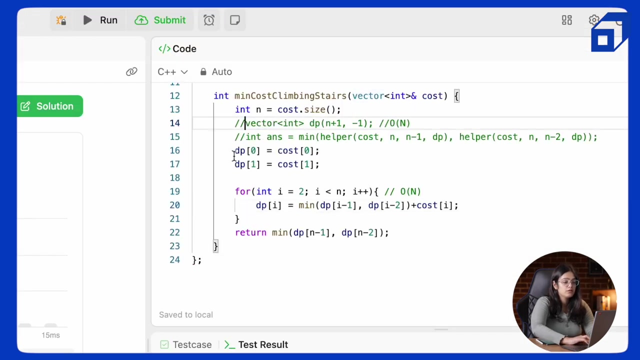 for the next one, we just need this and this, and we need to compare both of them to find the final answer. so we'll be storing just two previous values. so let's try and write this in code. so, instead of maintaining a DP table, I'll remove this. 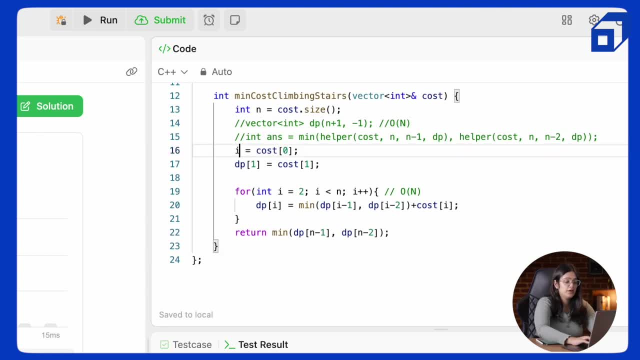 okay, so I maintain two variables: one is previous one, the other is previous two, and I will just- okay, let's just name this previous one because this previous two, because this is next to the previous one and this is previous one, the immediate previous one, for so here then again, the cost, the DP for 0 and 1 is: 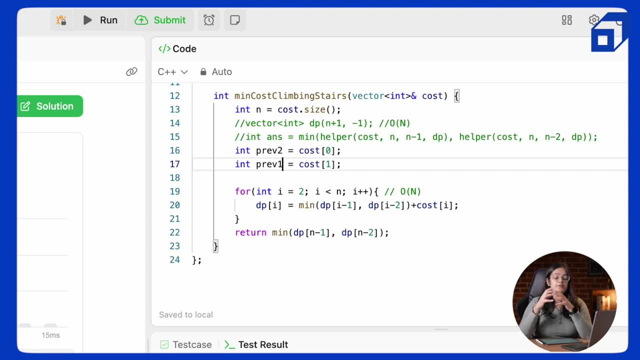 fixed. for 0 we have the answer as cost of 0 and for 1 we have the answer as cost of 1. so now we will start from value 2. so previous 1 to value 2 is the answer that will be present for the value 1. so essentially the answer for. 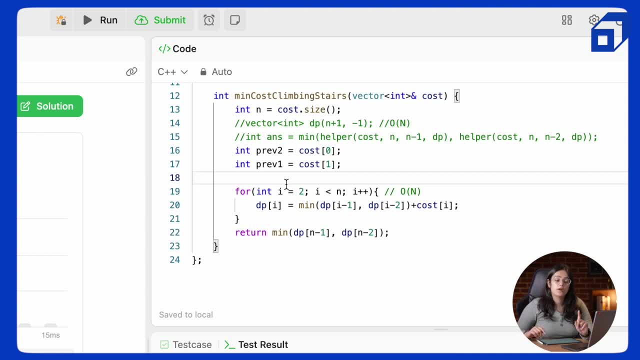 value 0 was 0 and the answer for index 1 was 1, so for 2 we have, if we are coming on index 2, we have two previous values, the index 1 and the index 0, so previous one will be corresponding to index 1 and previous 2 will be corresponding to. 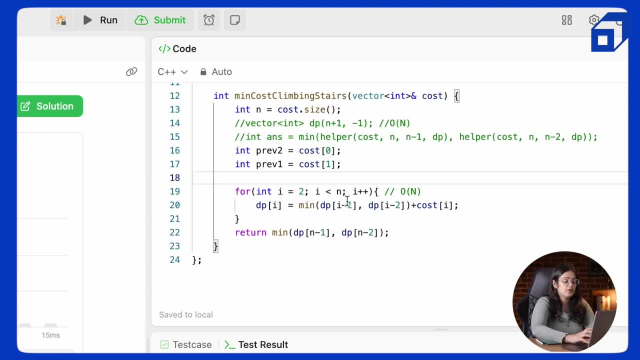 index 0. so now to calculate it for all the other values, we will just calculate the current answer for this index. that will be minimum of previous one, the previous value and next to previous value, and then we'll be adding the cost of I. now we'll have to update the previous values, so, as I showed here, we'll have to. 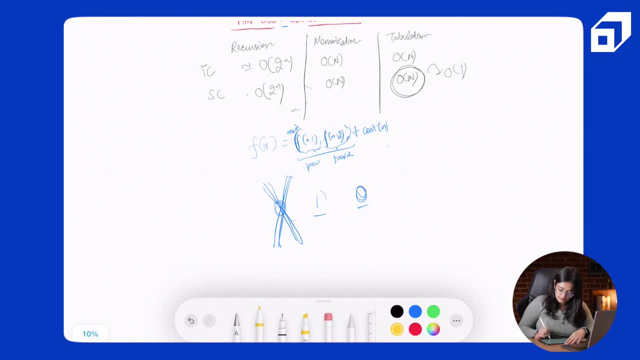 discard this value so earlier. so earlier: this was previous one, this was 0 index, 1 index, 2 index. so then previous of 2 was this one index, previous one and this was previous 2 and current value. we have calculated so for 3 this will become: 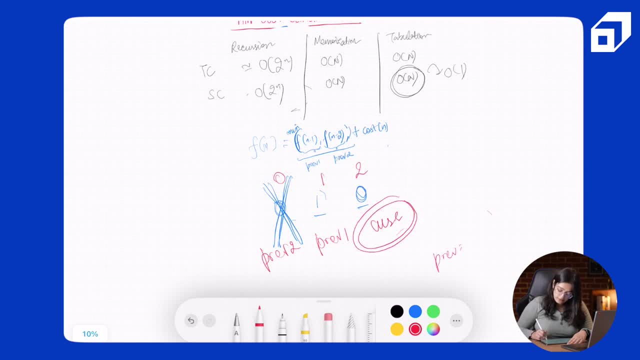 previous one. so previous one will become curve and this will become previous 2. so previous 2 has to become previous 1. so we're just moving one value forward to update the previous for the next index. So we'll just write previous2 equal to. 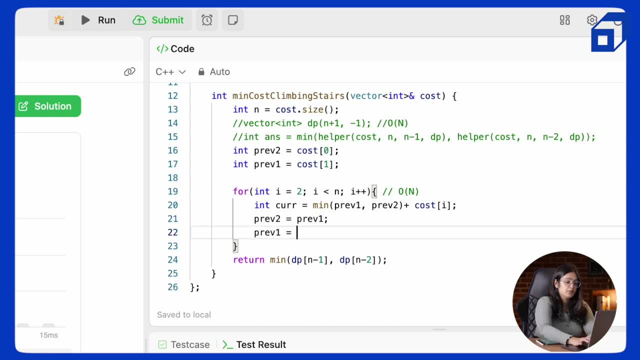 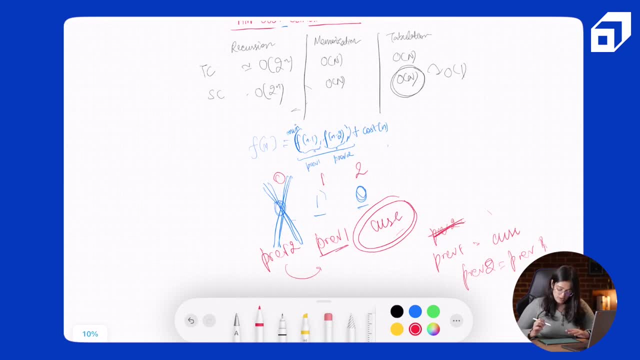 previous1, and then we'll update previous1 equal to curr, and then this will go on and at the end we'll be we'll have updated previous1 and previous2 and we'll have reached n-1.. So let's say this was the complete array of length 3.. So 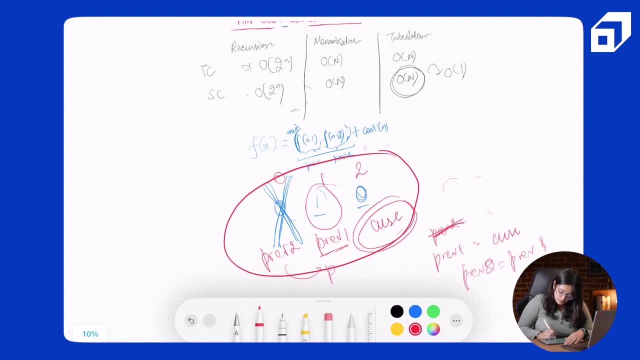 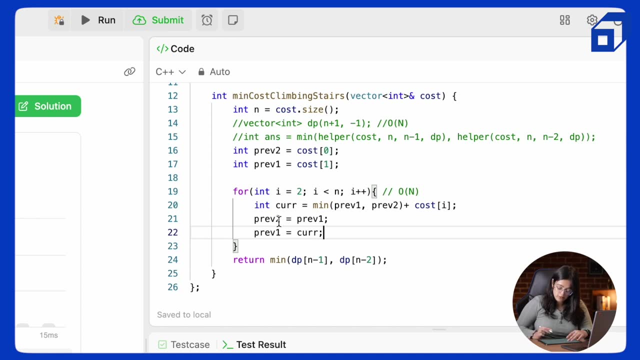 these are the two values, like: this would have become previous2 and this would have become previous1. after the updation, After we update in our line number 21 and 22,- the previous1 and previous2 would have updated and, if you want to. 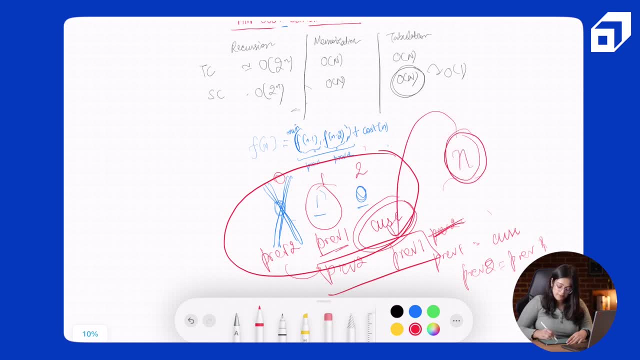 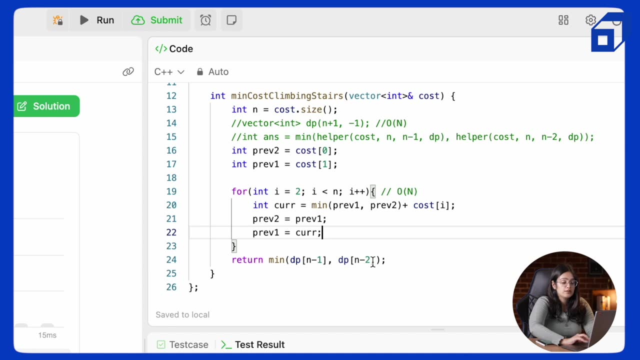 find the answer for n we just have to look at previous1 and previous2 and take the minimum of both, because it's, you know, the previous answer and the next to the previous answer. So to return the answer, we can just say previous1, previous2. 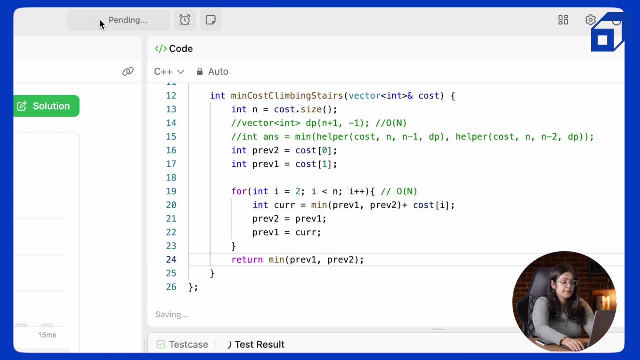 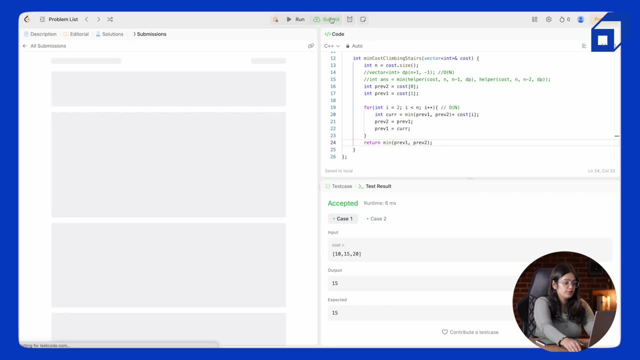 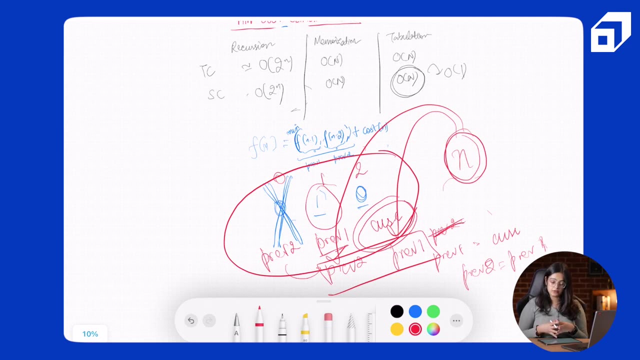 and run the code. Yeah, it's accepted. I'll try to submit it and, yeah, it works. So in this solution we optimized the space complexity even further and made it as O. So now let's discuss the next problem of the DB series, which is: 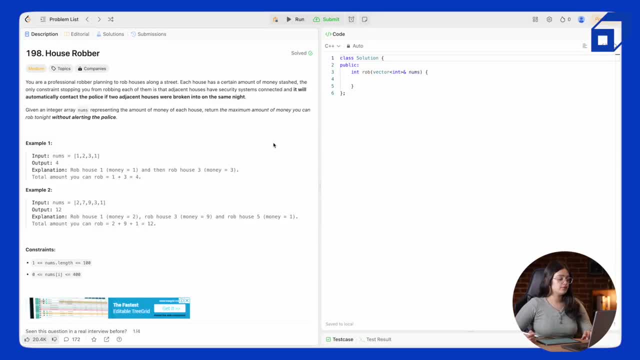 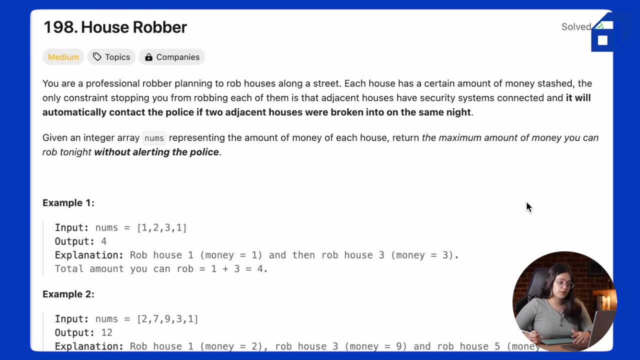 house robber. So this is a problem on leetcode as well. It's a medium level problem. So let's say you're a professional robber planning to rob houses along the street. Each house is a certain amount of money stashed and the only constraint 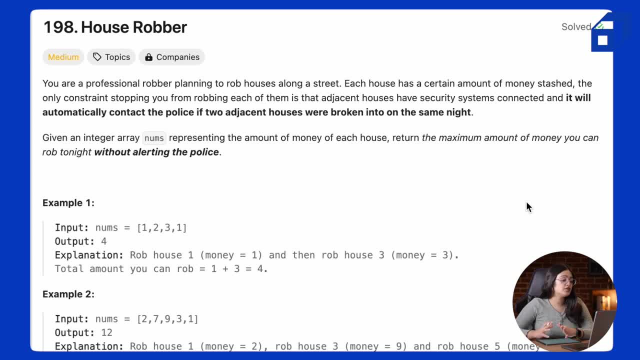 stopping you from robbing each of them is that the adjacent houses have security systems connected and it will automatically contact the police if two adjacent houses were broken into on the same night. So the constraint you have is that you cannot rob two adjacent houses, because it will allow the 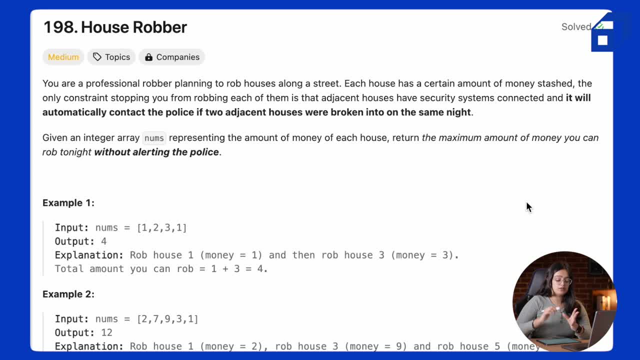 So the constraint you have is that you cannot rob two adjacent houses because it will allow the security system. So in this question you have to make sure that no two adjacent houses are robbed together. So to further like, show the amount of money and to give, to further provide the amount of money they've given an integer array. 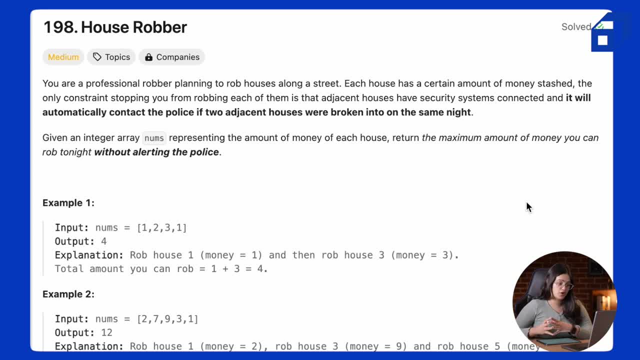 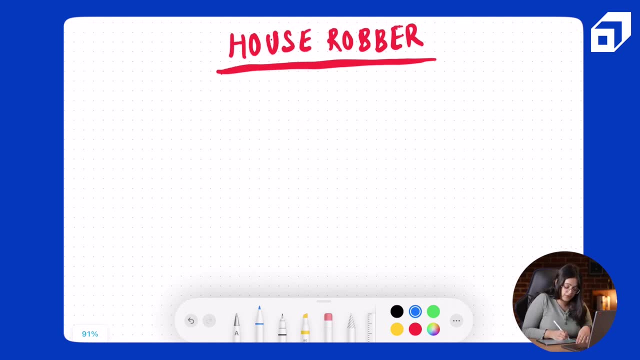 nums and that represents the amount of money of each house. So you have to return the maximum amount of money that you can rob without alerting the police. Without alerting means you cannot rob two adjacent houses. So let's say, let's take the examples that are given in the question We have. 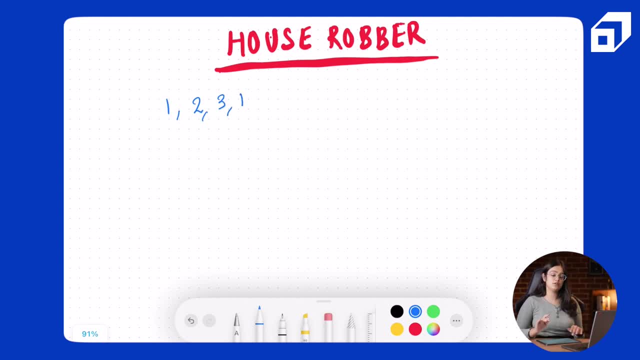 the array as 1,, 2,, 3 and 1.. So there are four houses and the money that the houses have is 1,, 2, 3 and 1 respectively. So here you can rob 1 and 3, the answer. 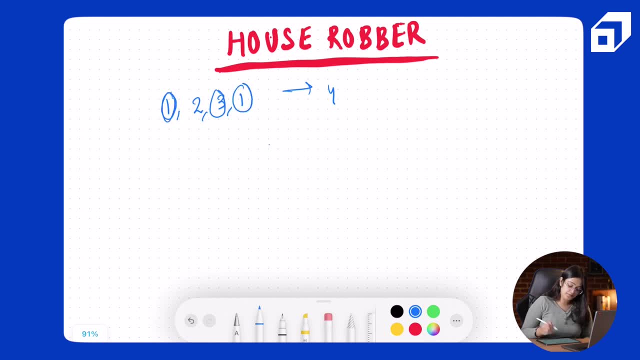 would be 4.. You can rob 1 and 1, the answer would be 2.. You can rob 2 and 1, the answer would be 3.. So the maximum amount of money you can keep is 4, without alerting the. 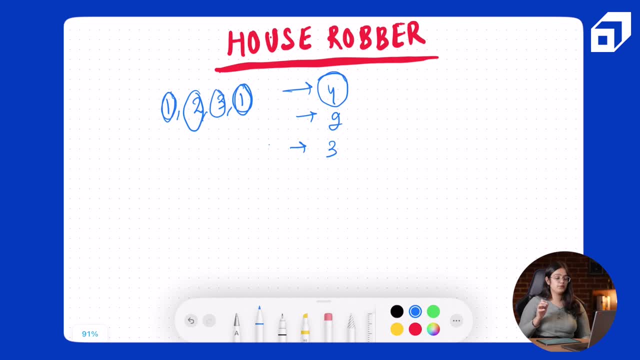 police. So essentially it is broken down into simpler terms. You just have to find the maximum sum from the array and you cannot take any two adjacent numbers Right. So maximum sum of a sub sequence of array where adjacent numbers aren't included. Taking the next example as well and trying to find the answer for it, 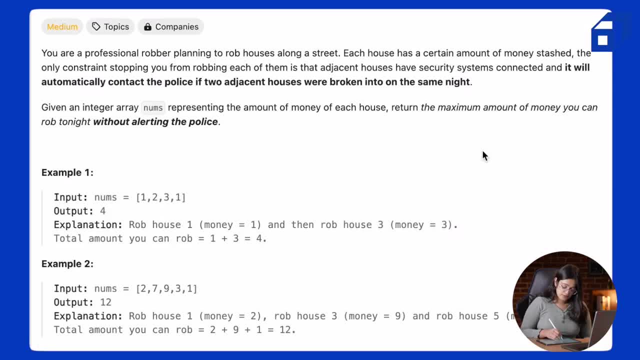 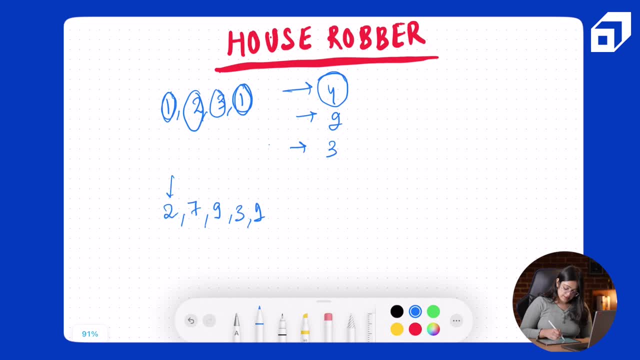 So we have 279.. 3 and 1.. So here our answer will come out to be 2 plus 9 plus 1, because if we take any other combination it's gonna be definitely smaller than that you can try and verify. so the answer here is gonna be 12.. So 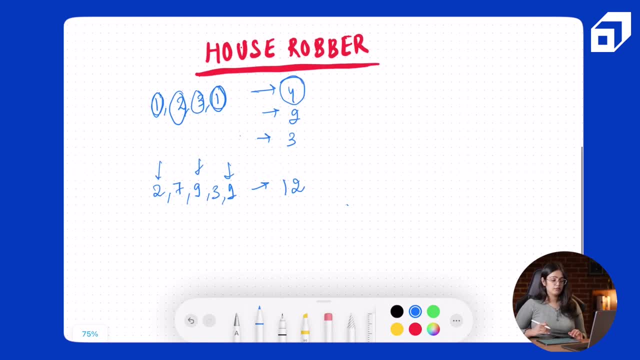 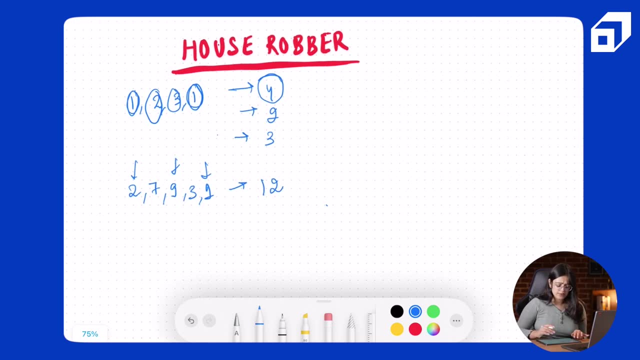 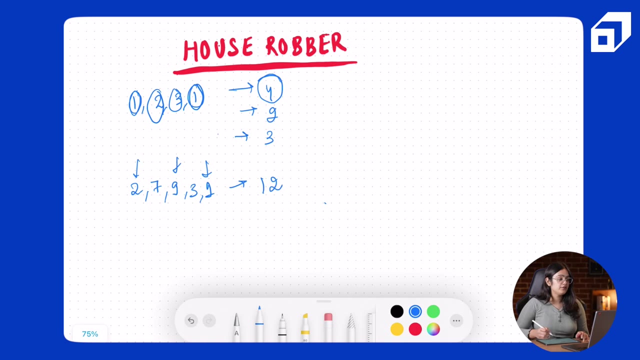 these are quite small examples and can be solved manually. but moving on to the bigger examples, we can try solving it using code, so that this will be a simple. this will also be a simple recursive solution, as we've been doing, so we can start a recursion tree. 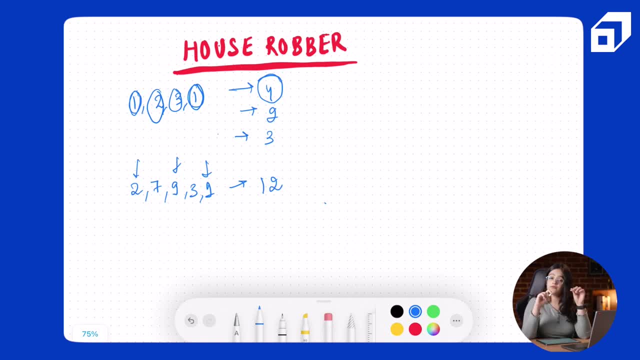 so like: what is the constraint here? once we rob one house, we cannot rob the next house. that's the only thing that we have to keep in mind. so when we start formulating a solution, let's say we are at index 0. okay, so either we can include. 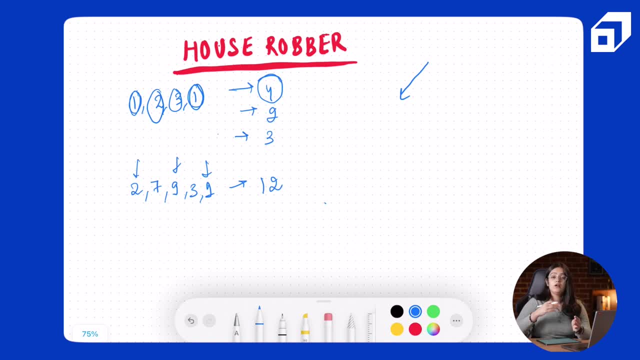 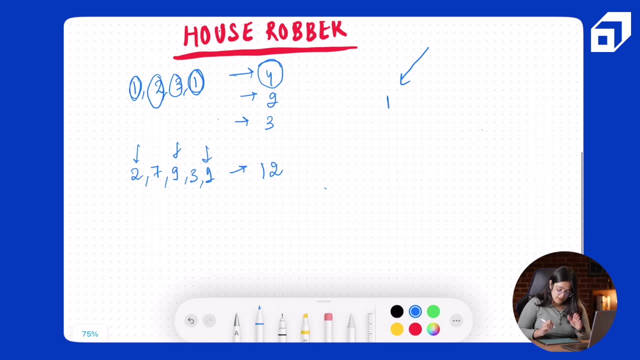 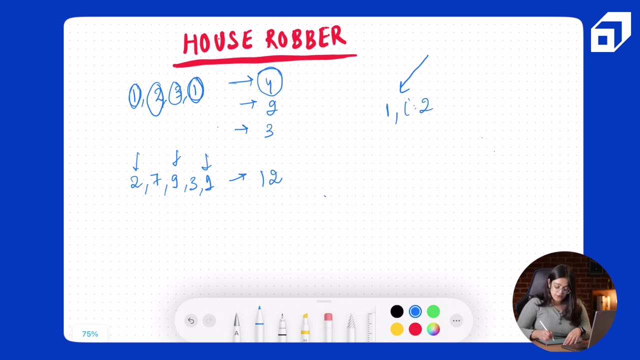 the index 0 and we can put a constraint that we cannot include the index one. so if we include the index 0, our answer is 1 up till now, and then we can, you know, pass on the index 2, because we cannot pass on index 1. so for: 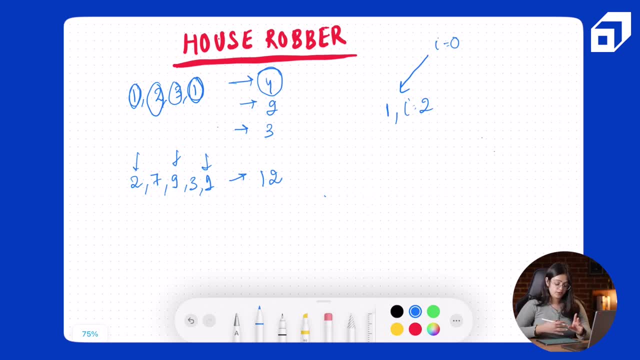 i equal to 0, we will pass on index two if we are including i equal to 1. if you're not including it, then we can just pastor the next i plus 1, because the we can have the best answer. It's possible to include i equal to 1, it's. 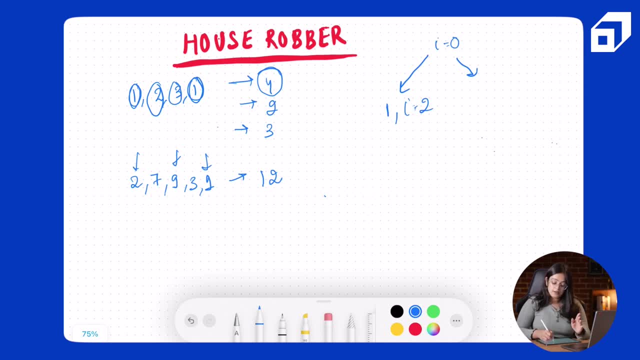 possible to not include i equal to 1, but from our end, we are saying that we haven't included index 0, so now, any answer that comes, whether we include one or whether we don't include one, that will be a best answer. but we can start. 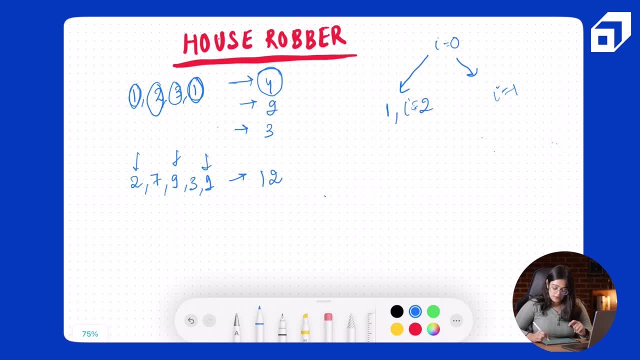 from index 1.. We have that freedom. It's not restricted. So if we are passing on index equal to 1, the answer is still 0, since we haven't included the house at index 0. So the recursive calls will go like: including a specific index and. 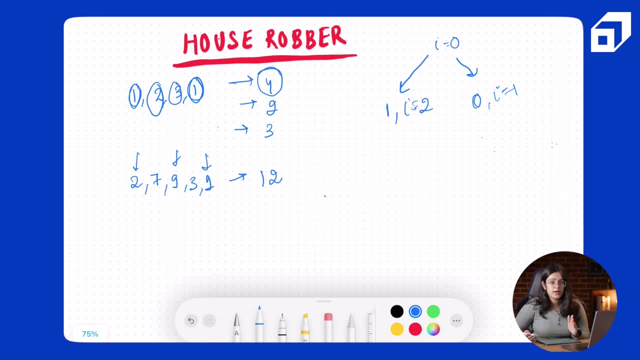 skipping the next index or not including the current index. and then you know, we can skip the next index or we can take it, So we only pass the next index. So the recursive relation for this particular problem will be: one call will be to include the current index and that will be f of i plus 1.. 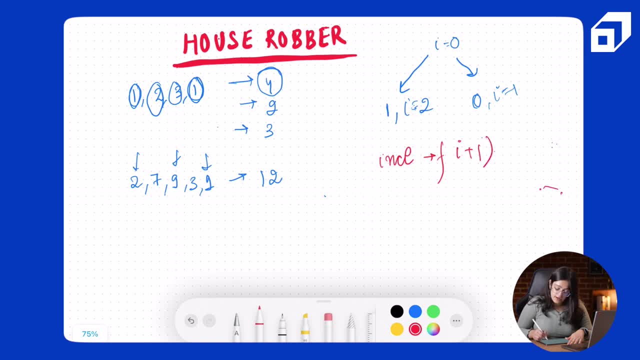 And while taking the value at the nums of i, like including this house, and if we exclude this, it will be f of sorry if it will be in the first case, since we're including i, we won't be including i plus 1 and it will be f of i plus 2 plus nums of. 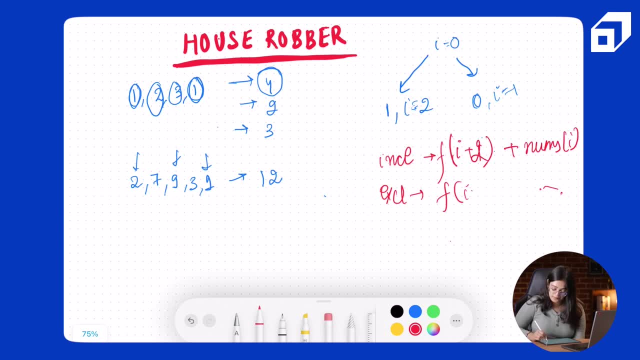 i and for excluding it will be f of i plus 1.. And we will be taking the maximum of both of these because we have to return the maximum amount that can be dropped. So whatever possibility returns the maximum amount, that will be our answer. 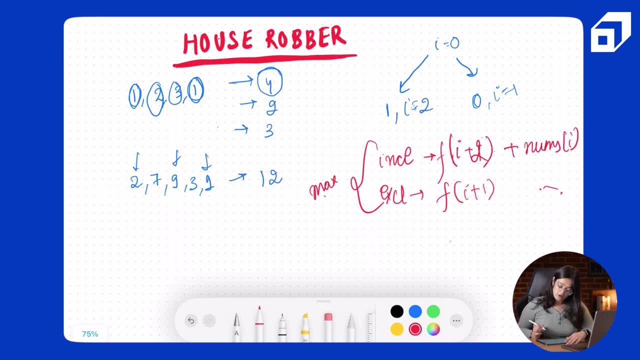 We can also write this in the exact opposite manner. So for our complete answer for any particular index, let's say we're standing at index i- the answer for index i would be include index. i skip this one and get the answer of i-2.. So it will be f plus. 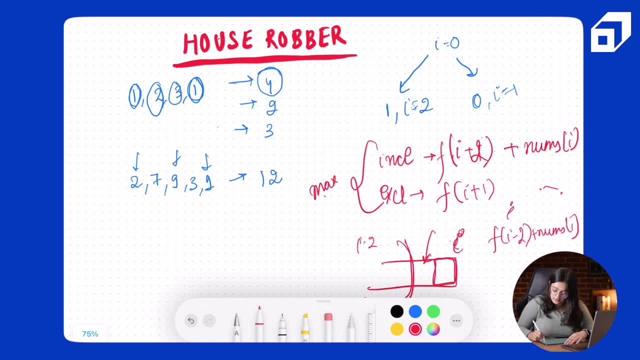 nums of i in the include query and if we're excluding i, then we'll take the answer of i-1.. Whatever answer is still here, that will be our answer. So whatever answer has come till i-1, whether it includes i-1 index. 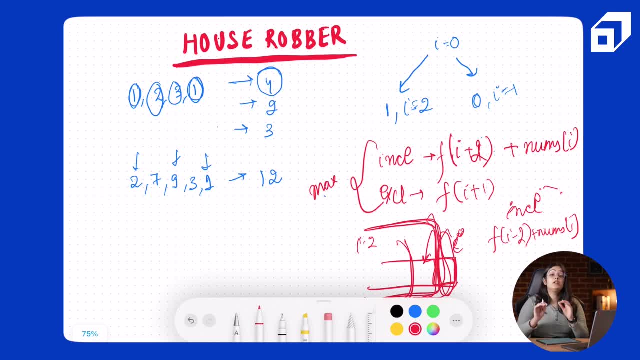 whether it doesn't include i-1 index. it doesn't matter, because we're allowed to include that. So we'll just take the answer that has come to the previous index. So when we're excluding i, the query will be f. So the 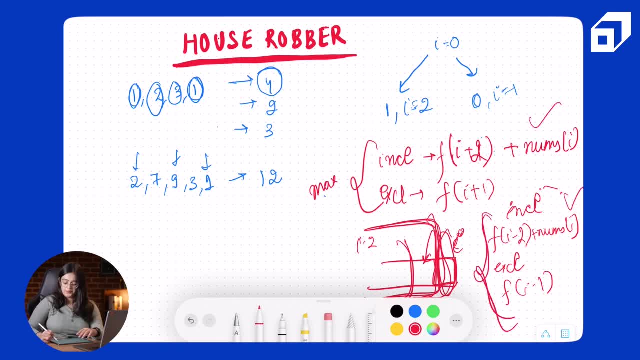 maximum of these will be our answer. So either ways we can write. I'm going to be writing the code using the second one and talking about the base case in this particular solution. So for i equal to 0,, when i equal to 0,, the only house that a. 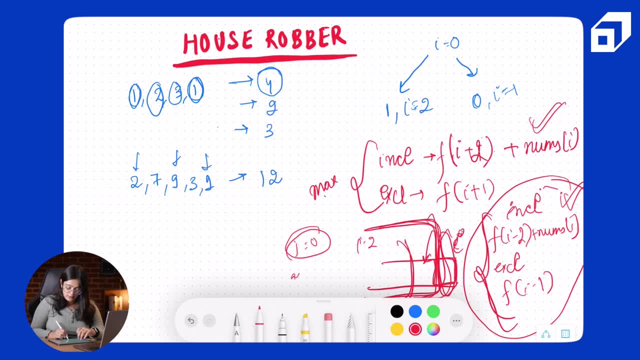 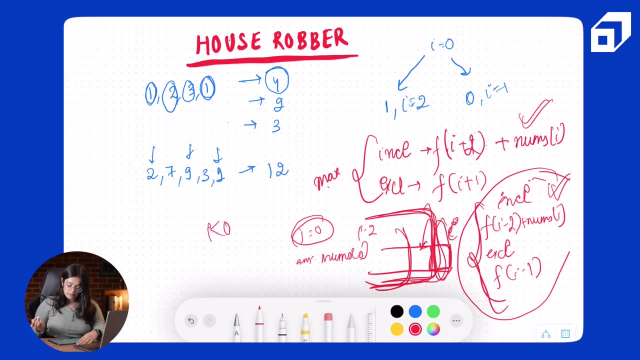 person can drop is house number 0. So the answer would be nums of 0. And for i less than 0. So let's say win are subtracting 2 from the previous index or one from the previous index, if in any case we reach. 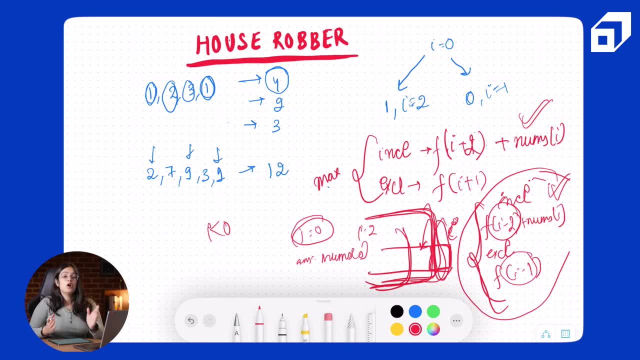 a value where it's less than 0, then there'll be no houses before 0, right? So the answer we have to return is 0 at that point, because there can be no cost that is possible. So if there is no house, so there's no money to drop. 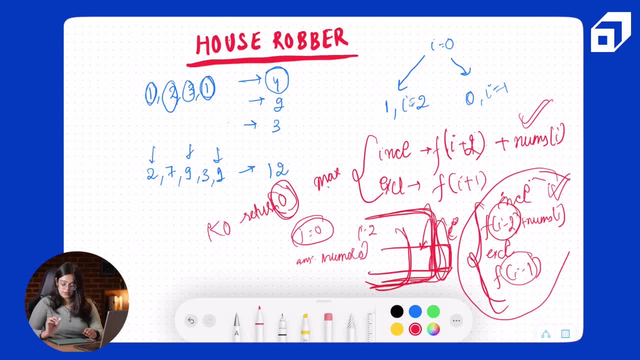 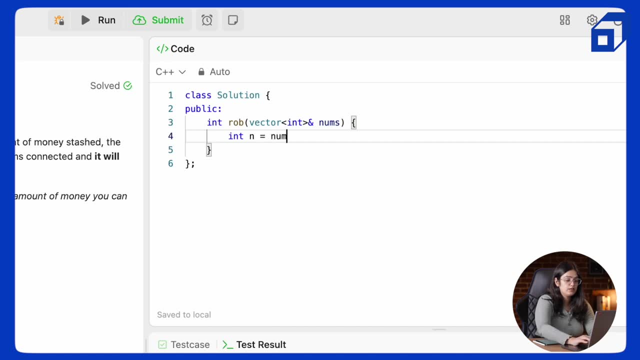 So for i less than 0, the answer will be 0. So we'll have to return 0. So we can write the recursive code for this quickly. So we have n equal to numssize. I'll quickly create a helper function to help us calculate our answer. 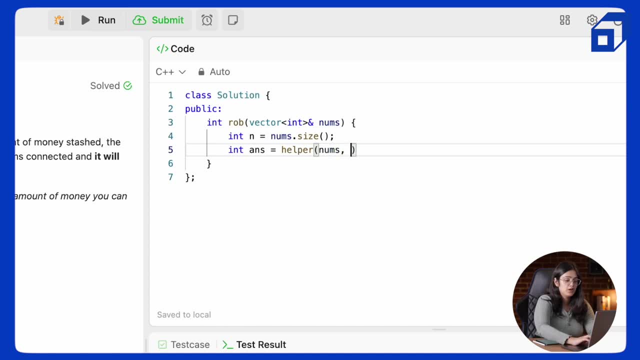 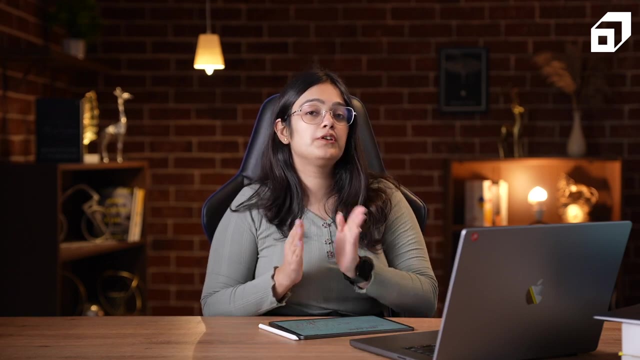 So our answer will be helper and we'll pass on nums. We'll pass on. we'll actually pass on n minus 1, because we have to calculate the answer till n minus 1.. So whatever is the answer at the last index, since we are checking at every index whether to include it or not- 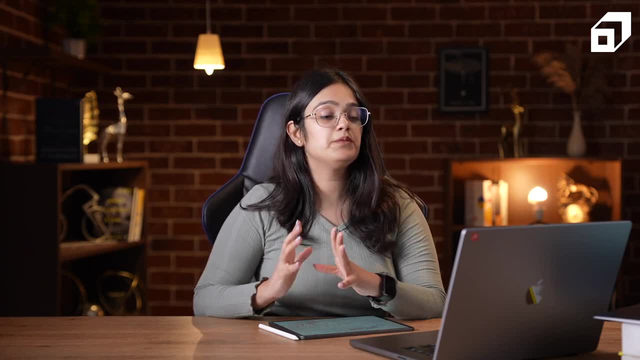 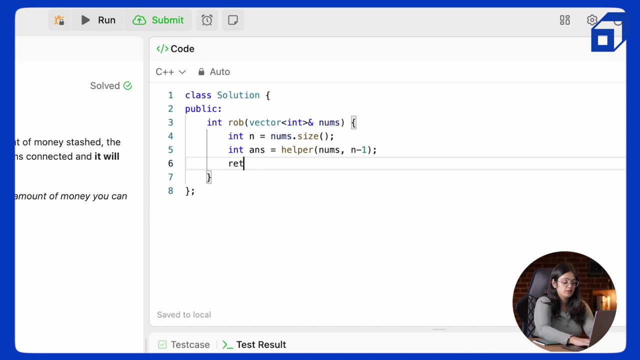 So whatever is the answer till the last index till the end of the array, that will be the maximum cost. So we have to calculate the answer for index n minus 1.. We can return the answer. I will write the helper function. 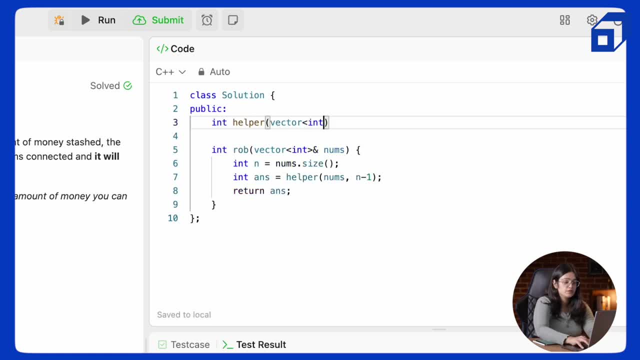 So it will take our vector nums, It will take the index. So if our index is less than 0, as we already discussed, if our index is less than 0, then we can return 0, because there is no houses before 0. 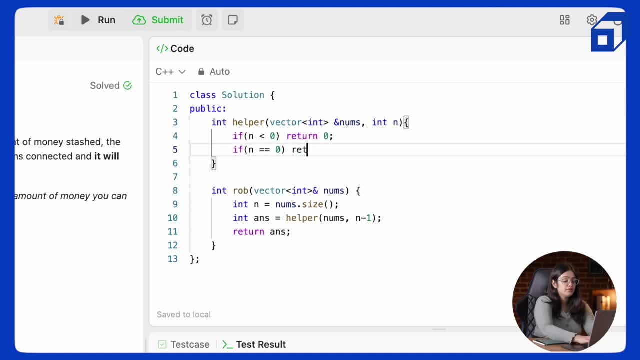 If our index is equal to equal to 0, then we can return nums of 0.. Only one house is there and that's the answer. Else, for the generic case, we can either include the current index and the value added. We can include it in our final answer. 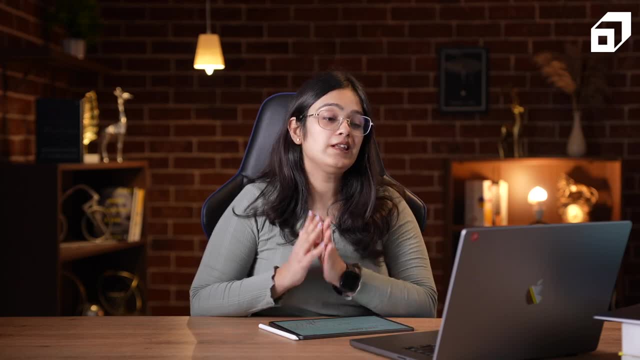 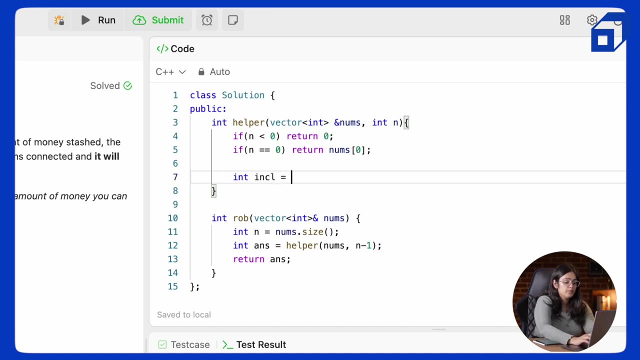 And then we'll have to go two indexes back, Or we can exclude it and we have to go one index back. So I'll be writing the include query. That will be helper of nums. We'll be passing n minus 2 and we'll be including nums of n in our answer. 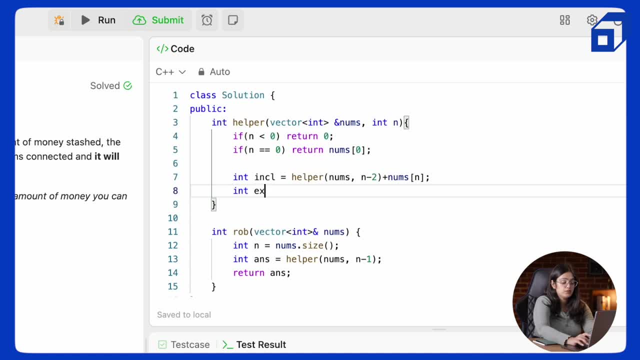 The current index, And if we excluding this, we'll be passing n minus 1, and we won't be including anything. So that's simply nums of n minus 1, and then we'll be returning the maximum of both of these. 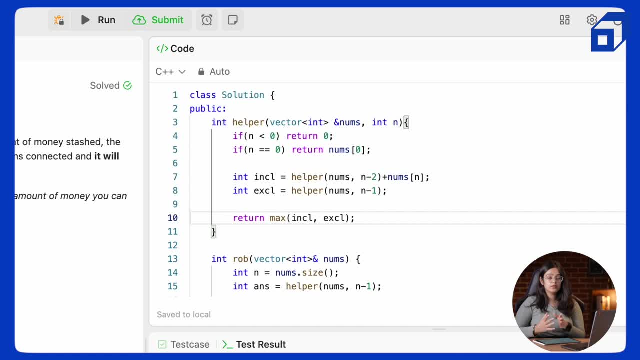 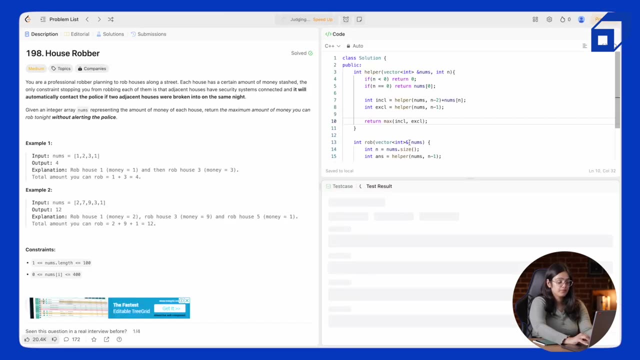 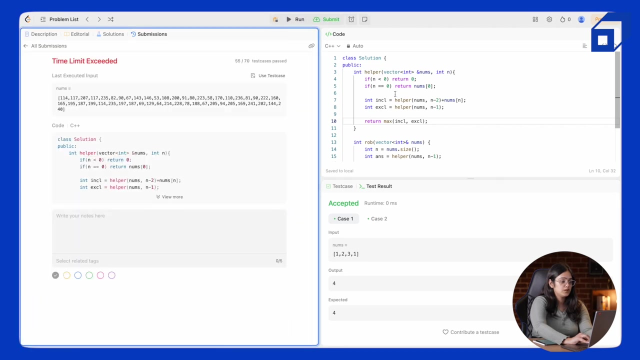 So for every index, we have two choices right: Either to include the current index or to exclude the current index. Our answer is the maximum of both of these possibilities, So at the end we're returning the maximum of it. Let me run this code. Yeah, Try and submit this. 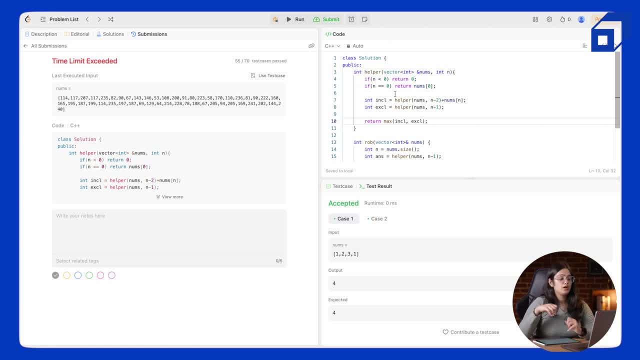 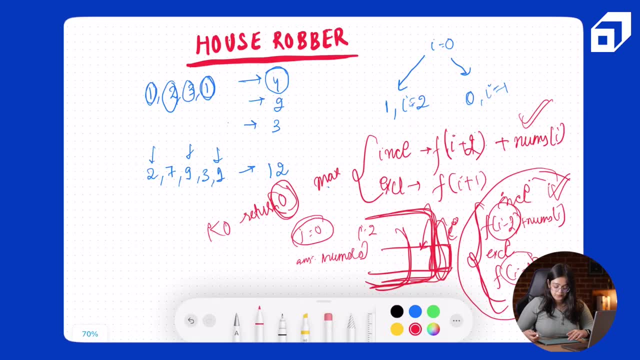 So we're getting a time limit exceeded, error due to a lot of recursive calls and a lot of repetitive calculations. So, as we did in the previous questions, we'll again do the memoization solution for this one, because there will be possibilities that when we are 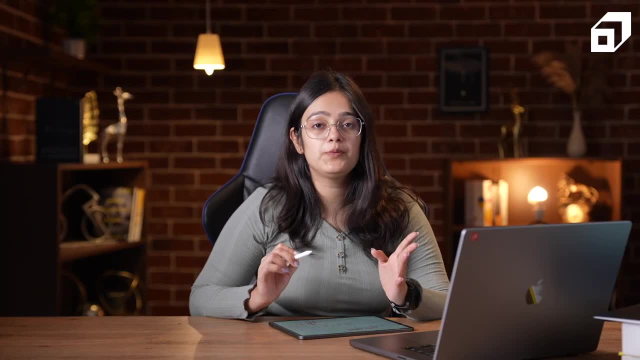 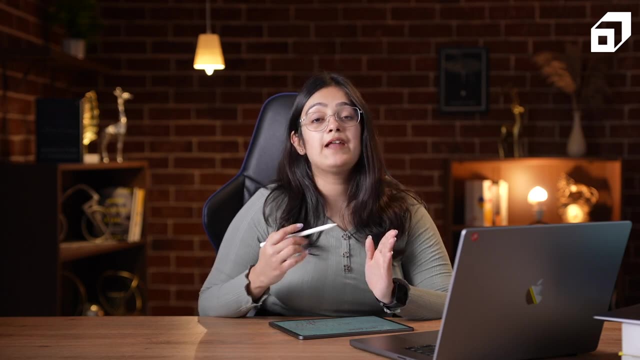 coming one step back or two step backs from any particular index. there will be possibilities that we'll land on the same index multiple number of times, And when we are landing at the same index, we're calculating our answer again and again by the recursive calls. 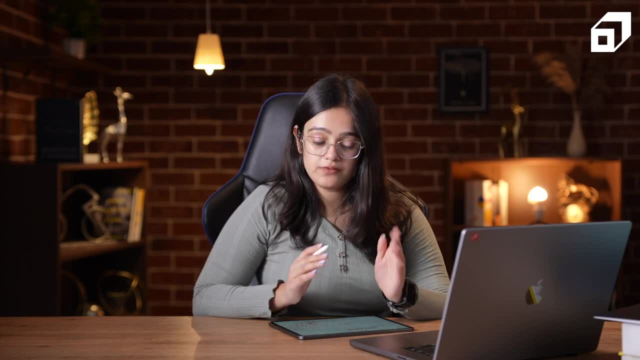 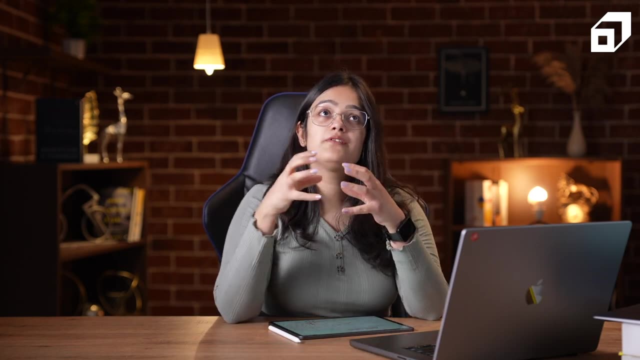 So what if we cache the answers for each of these indexes, like we did in the previous questions? What if we maintain a DP table and whenever we find an answer we store it in the DP table? So whenever it occurs that again we have to calculate the answer for? 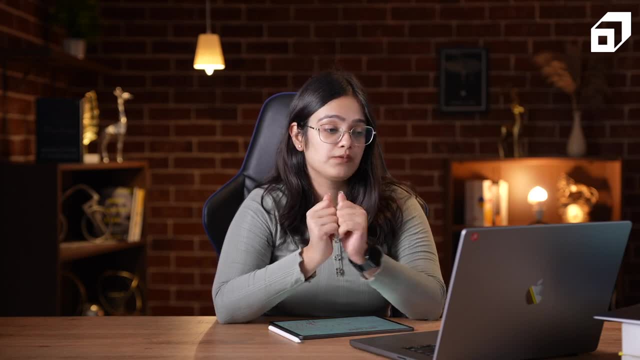 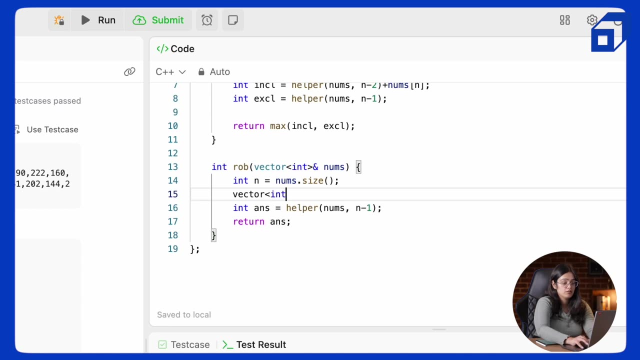 that index. we can just reuse our previously calculated answer. So I'll just memoize this solution. I'll create a DP table of size n And I'll initialize it with minus 1.. I'll pass it on in our helper function query And. 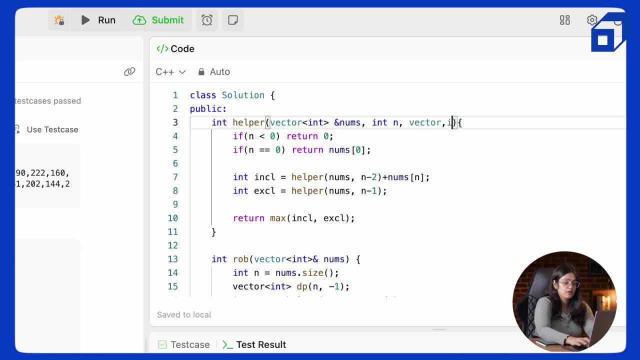 I will also take this one here. Have to pass it in the calls Now. initially, the DP table has values of minus 1 for all the indexes. If we encounter an index where the DP of i is not equal to minus 1, which means we've already calculated the 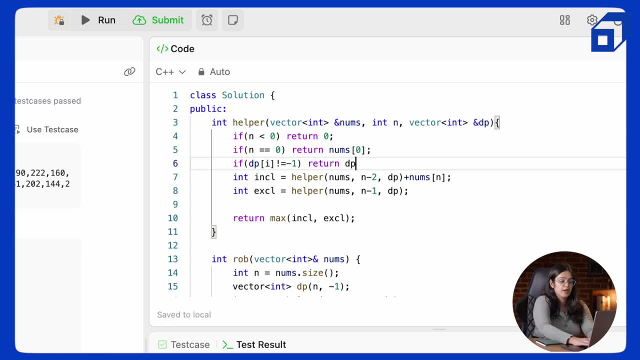 answer and stored it in the DP table. In that case we'll return the DP of i. In other cases, where it's still minus 1, we'll populate dpi to be the maximum of include and exclude query. We'll populate it with our answer and we'll return it. So, since we're populating the 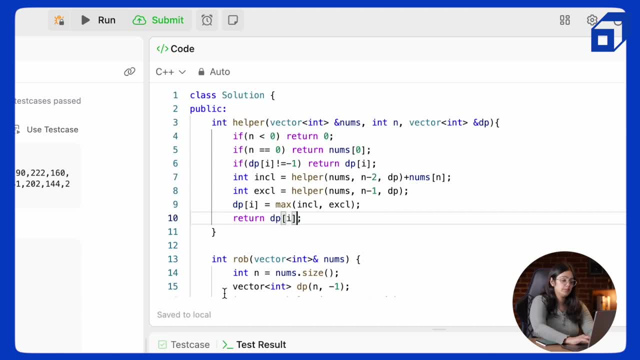 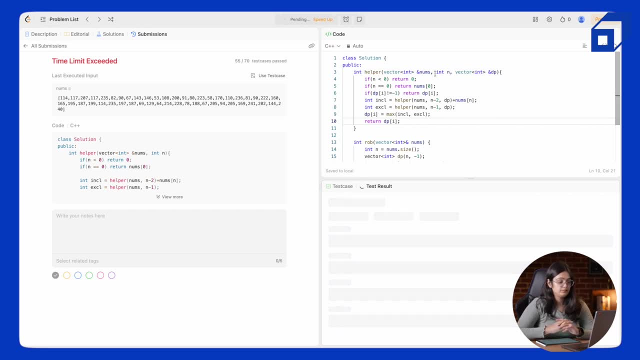 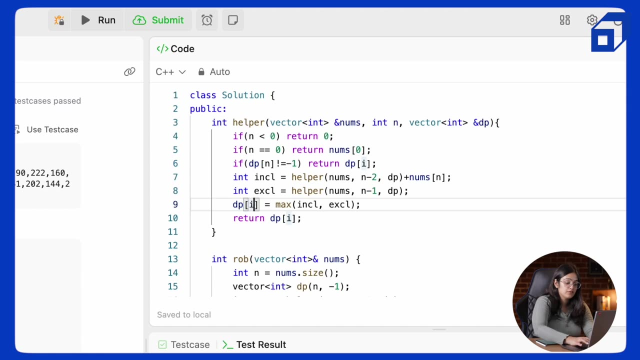 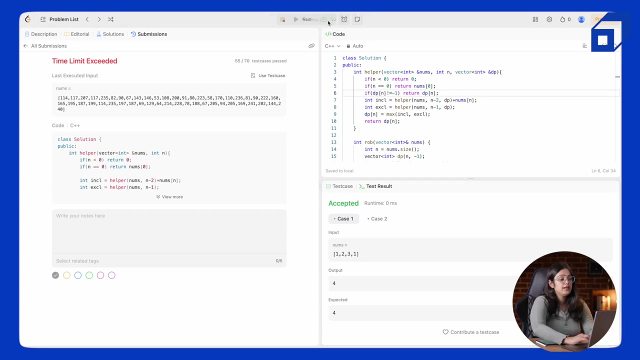 time anybody tries to reuse, the answer will be available in the DP table so we can run this. okay, so actually we are using n as the index here. we'll run this again. DP of n. and yeah, it's accepted. let's submit this and see if the TLE is still. 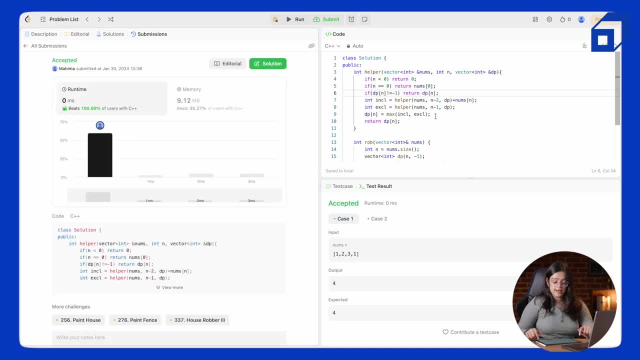 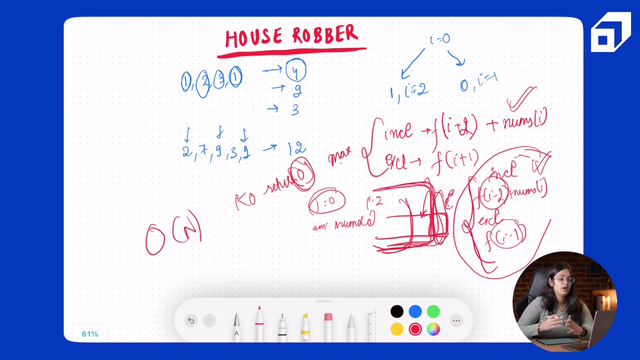 coming. yeah, it's accepted, and the TLE is gone because we significantly optimize the recursive solution and now we are calculating once for every value. so now again our time. complexity becomes o of n, coming from O of 2 to the power n, where we were making an inclusive call and an exclusive call. 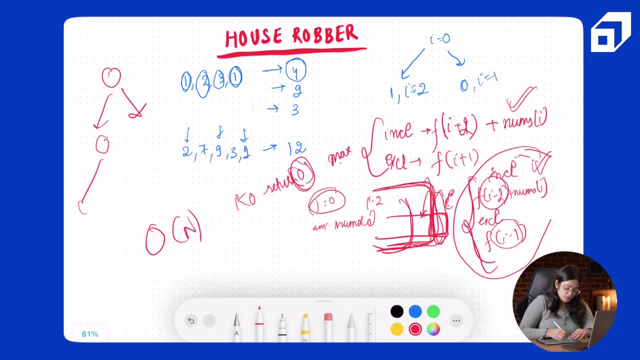 So we were making two calls at every step and trying to calculate the answer. So, from 2 to the power n, we have reduced it to O of n And for the space complexity as well, since we're using a helper array and a DP array. 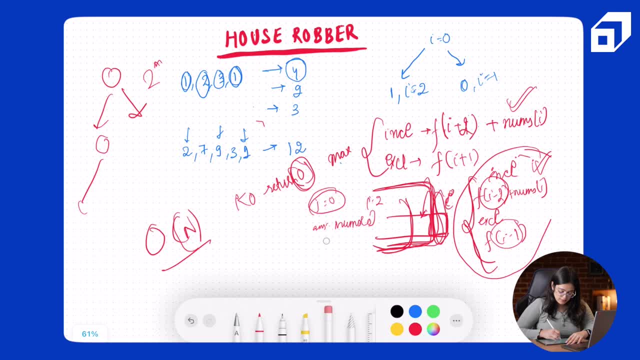 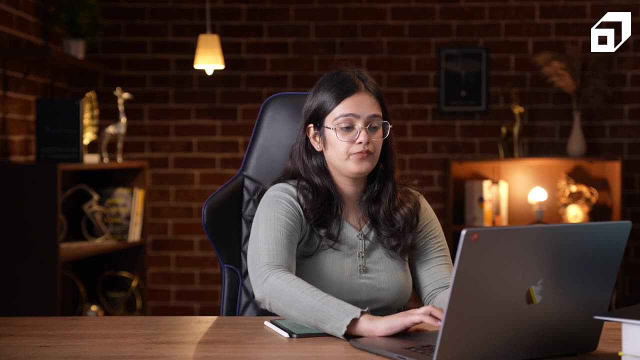 so we are also using the space complexity of O, of n here. So now let's also write the tabulation solution for the same. So in the tabulation solution the other things are going to be same. This base case is going to be same. 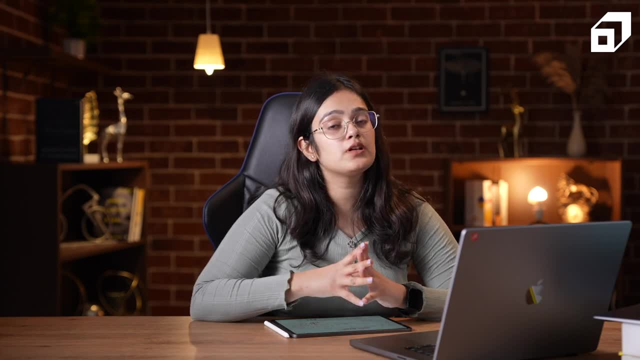 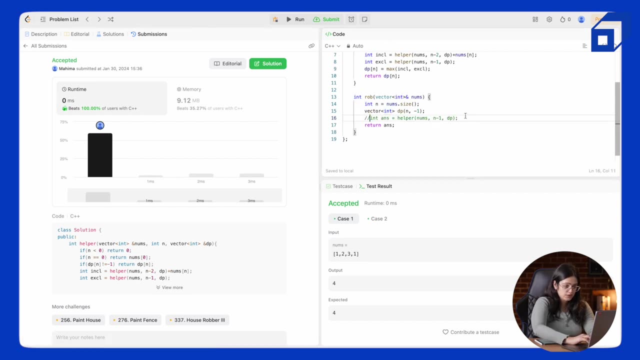 The recursive relation we're going to be using is going to be the same. We're just using a for loop to formulate the solution here. So our DP table is here. Let me comment out the code for the memoization solution. I'll just initialize our DP for our base case. 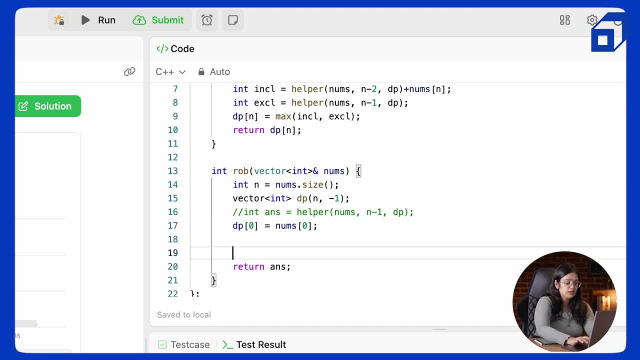 Which is DP of 0. That is nums of 0. We'll start calculating the answer for i equal to 1, i less than n, i plus plus. Now our answer will be inclusive. So there'll be two queries, again like the previous one. 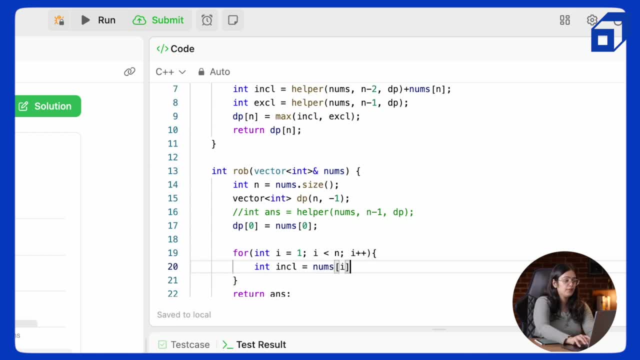 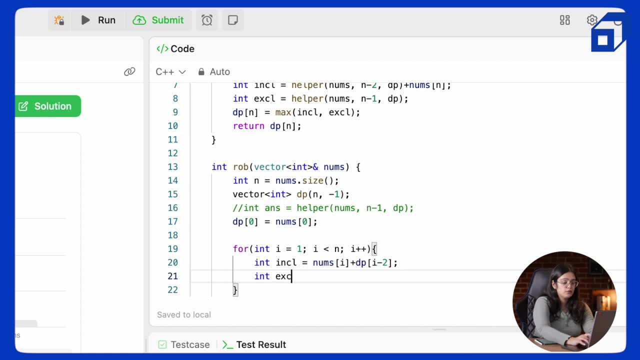 In the inclusive one, we'll be adding nums of i plus we'll be adding DP of i minus 2.. And in the exclusive, we'll be adding nums of i plus we'll be adding DP of i minus 2.. And in the exclusive, 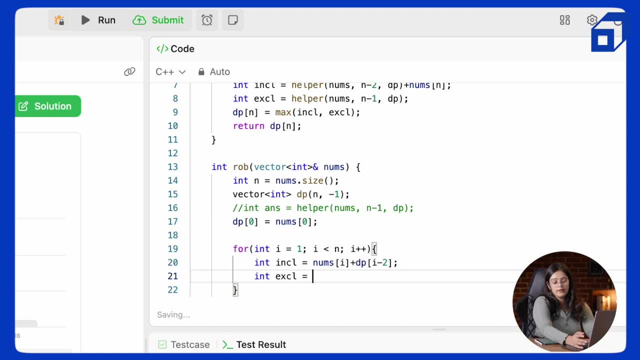 we'll be adding nums of i plus. we'll be adding DP of i minus 2.. And in the excluded query we'll be not adding the current value because we're not including it, And we'll be taking DP of i minus 1.. 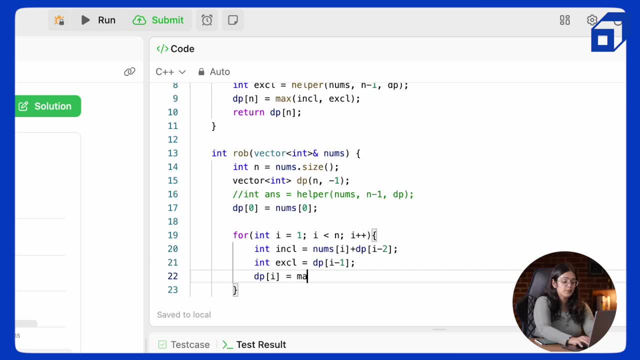 And the answer for DP of i will be the maximum of inclusive and exclusive. At the end we'll have to return DP of n minus 1.. The answer to the last index- One small thing here- is that for i equal to 1, i less than n, i plus, plus, plus. 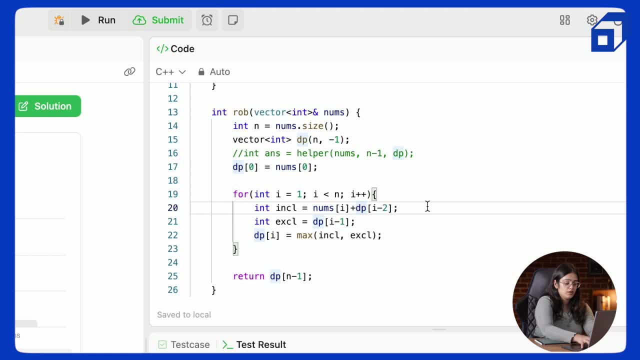 i equal to 1, i minus 2 will not be there, like it will be out of bounds. So we can just put a condition: if i minus 2 is greater than equal to 0, then only we have to take DP- i minus 2, otherwise we can take 0.. 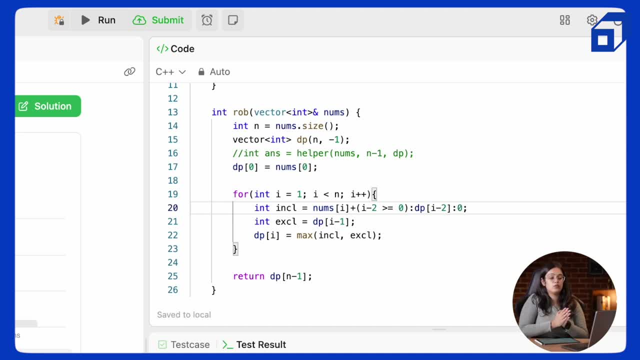 Because if it goes out of bounds it's anyway. there's no house present, so we'll take 0 here. So I'll just use this ternary operator here and I think we should be good to go. Let's run the code. 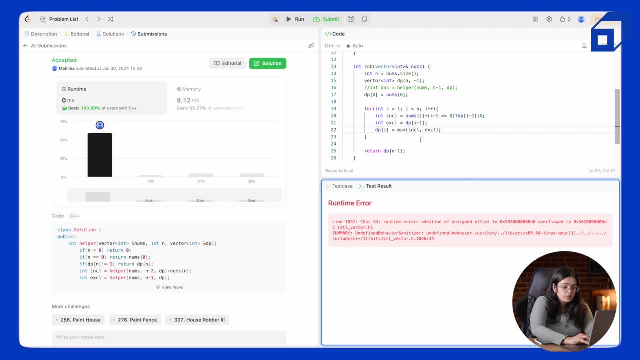 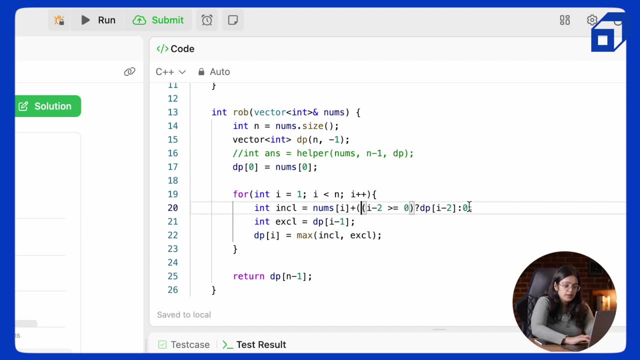 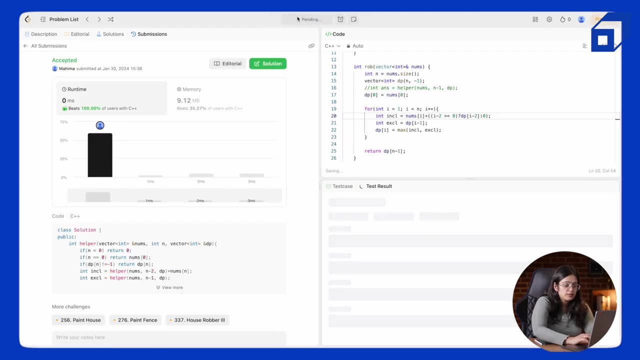 Let's put this in brackets. Yeah, so it's accepted. Now we can submit the code and check if it works. Yeah, so it works. So this was the tabulation solution of this question. Now, one thing that we've done in the previous question is that 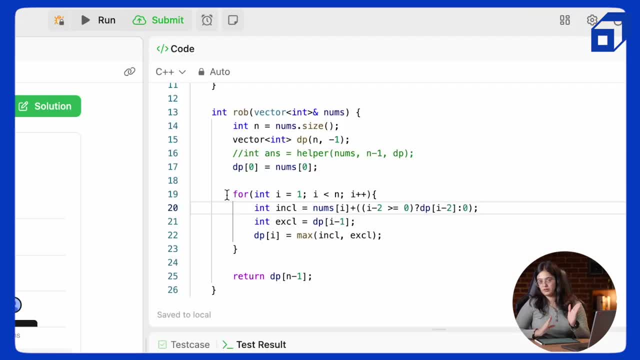 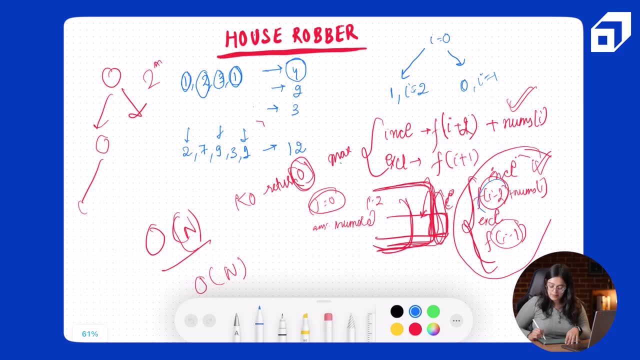 we noticed that our answer was depending on only two previous states: previous 1 and previous 2.. If you notice, in this question also our answer is depending only on two states: i minus 1 and i minus 2.. So, like we did the space optimization in the previous question, 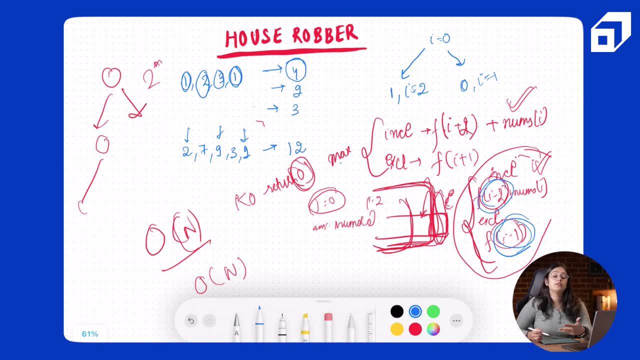 where didn't we declare two variables- previous 1 and previous 2, instead of minus 1 and minus 2.. So we're just making a DP array and storing the answers for all the values In this question. also that space optimization can be done. 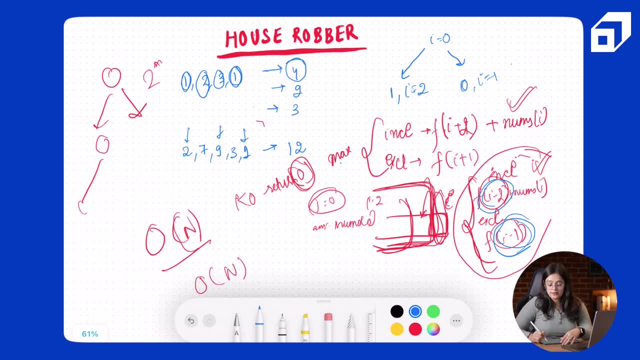 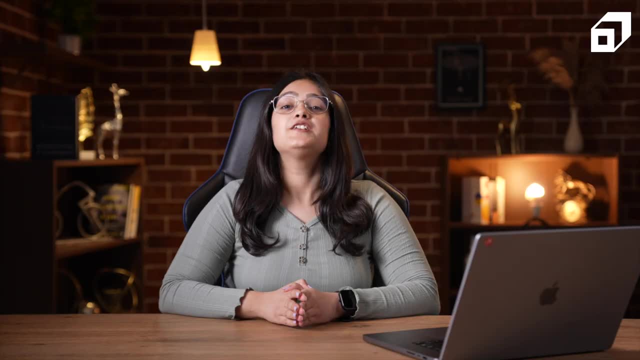 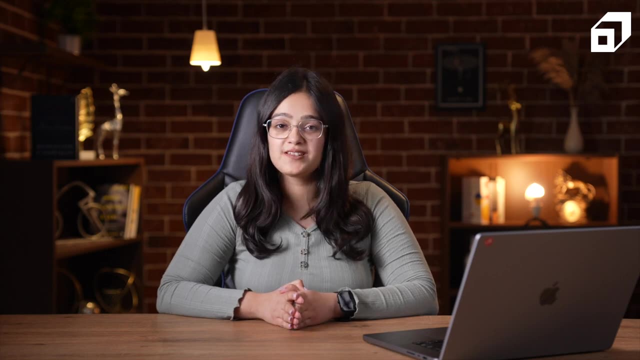 That's what is your homework. You have to do the space optimization and try to make the space complexity to be O of 1.. It will be very similar to the previous question, So it will be very easy to do that. So I hope you were able to understand how dynamic programming problems are solved using top-down and bottom-up approaches. 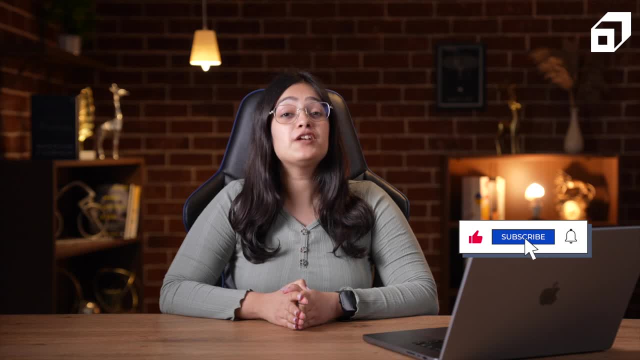 If this video was helpful for you, make sure to like it. Make sure to mention it in the comment section below. Make sure to mention any comments or any doubts you have in the comment section and we'll be happy to answer. Subscribe to Scalar's YouTube channel for more such informative content. See you.